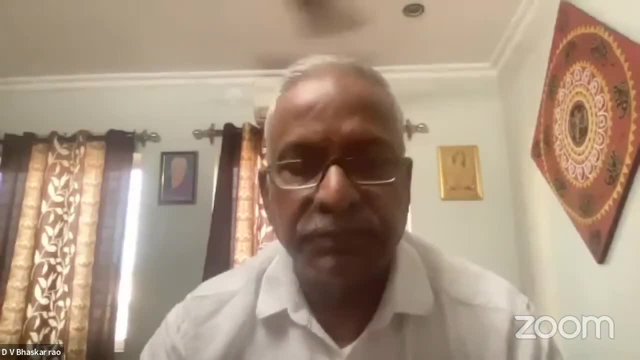 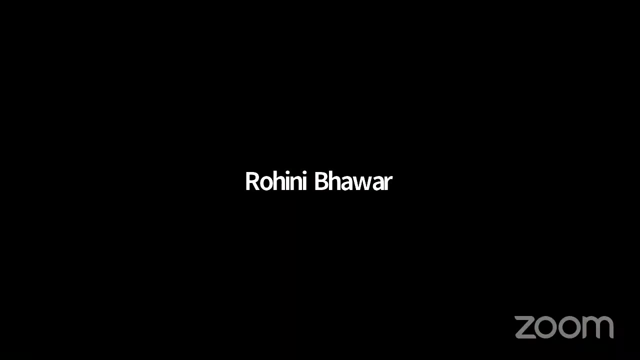 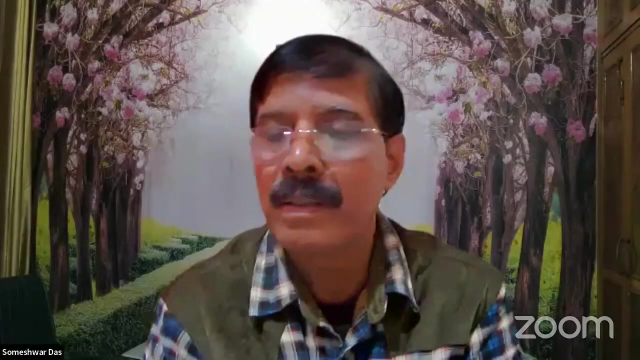 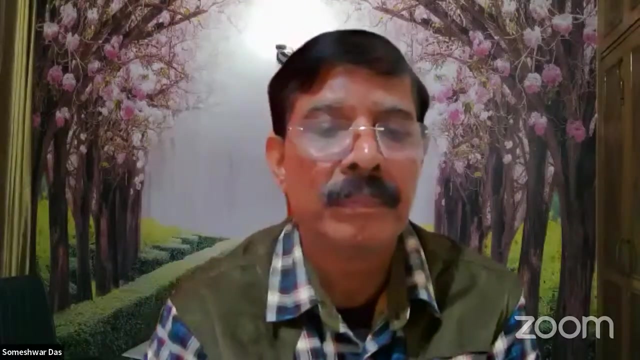 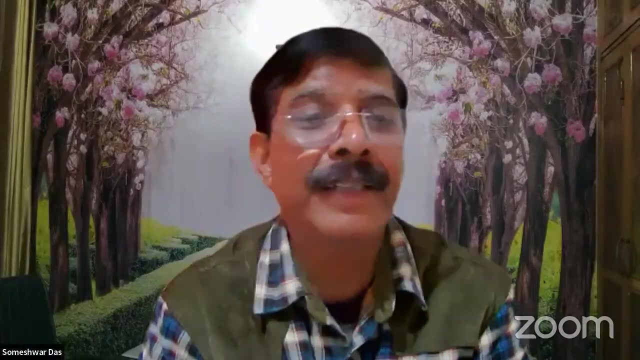 No, It shows. sir, you are a co-host already, Yeah, and who can share? All panelists can share, So he should be able to share. So I am going to share, you know. In the meantime, I can say that previously it has happened. You did something and I could show. 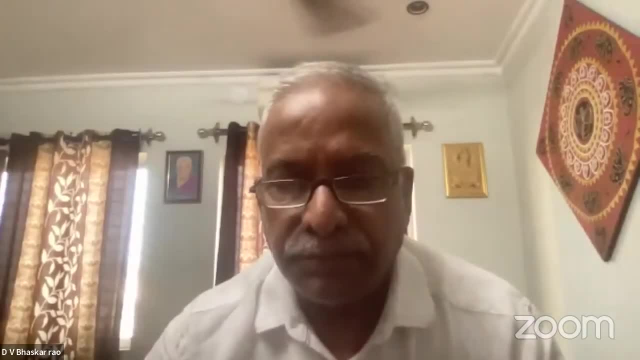 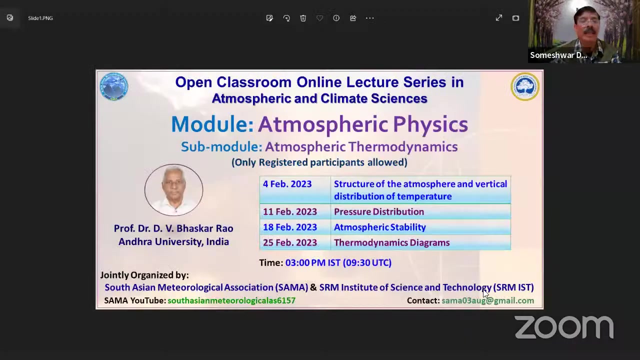 Do you think I should rejoin? Maybe Try. Okay, sir. Okay, Share screen button is coming on my side. Okay, Yeah, it's okay. Yes, from my side. also, share screen. No, share screen. but I think sir is saying that he is not able to share. 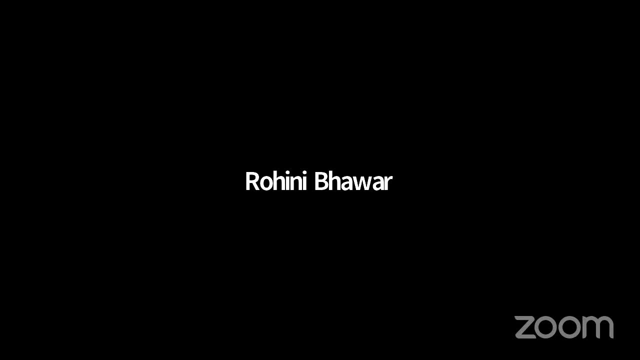 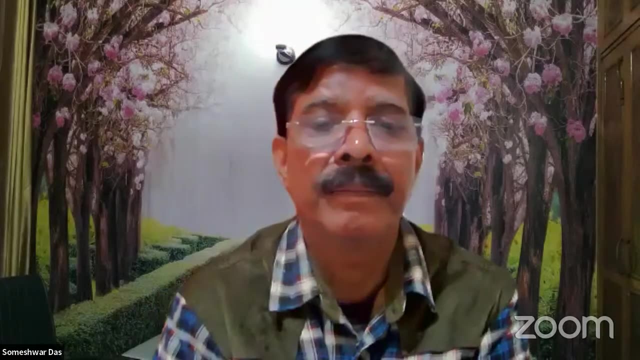 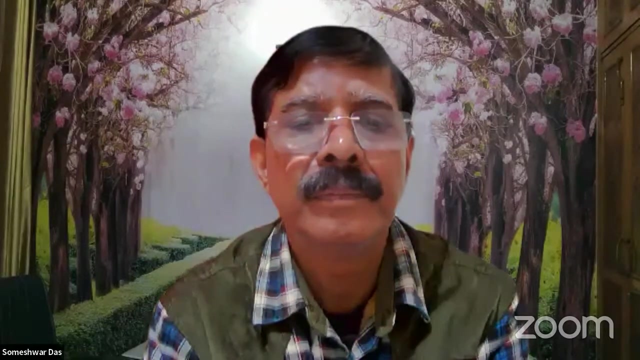 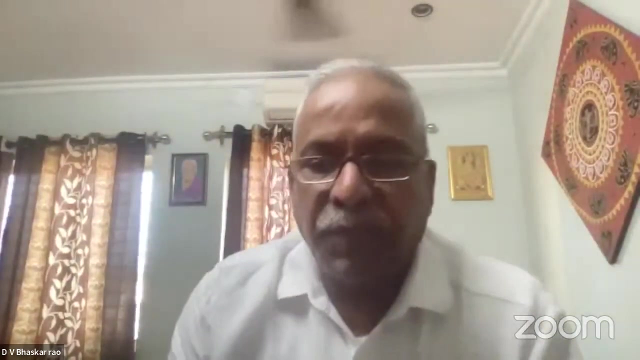 Even it is there, but why I can share directly. yeah, He is trying to log in again, but he has logged in again. I couldn't see and share. Oh, the green button is not there. It's there, You see. 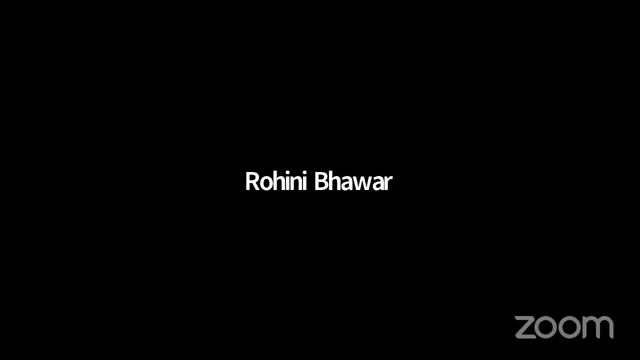 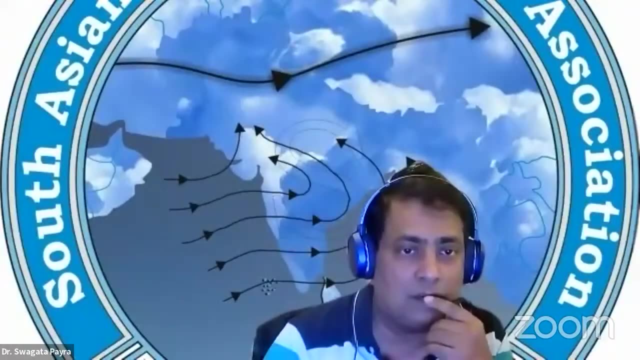 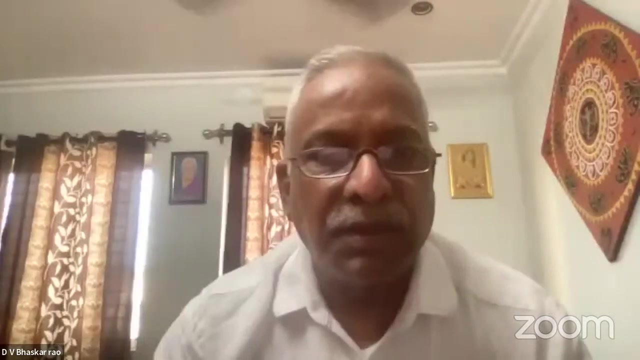 Sir, can you click on that? only Yeah, I clicked, and Okay, Okay, Okay, Yeah, I clicked, and then a screen came. So click on that screen. What screen? And then in the right below corner there is a share. 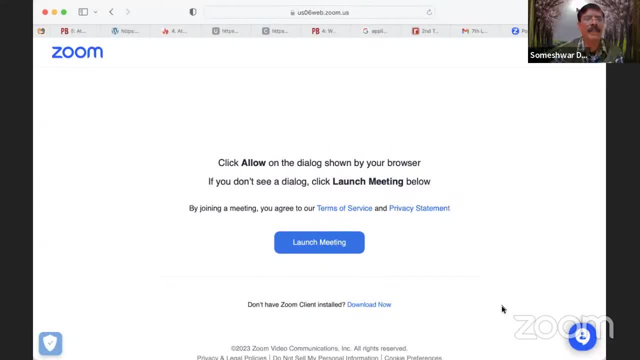 Yeah, correct. Yeah, it's coming. Yeah, yes, yes, it is coming. Yeah, we can see your URL. TPT is not seen. TPT is not seen. Zoom is not seen. Yeah, we can see your URL. 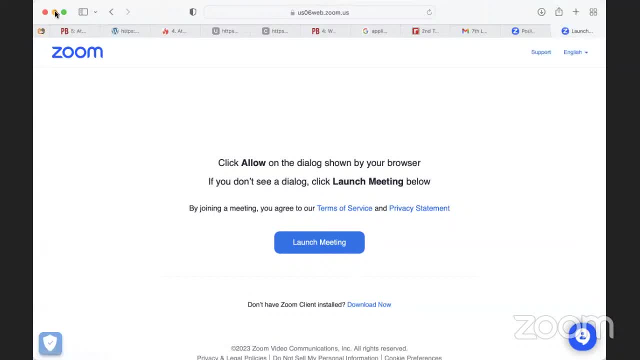 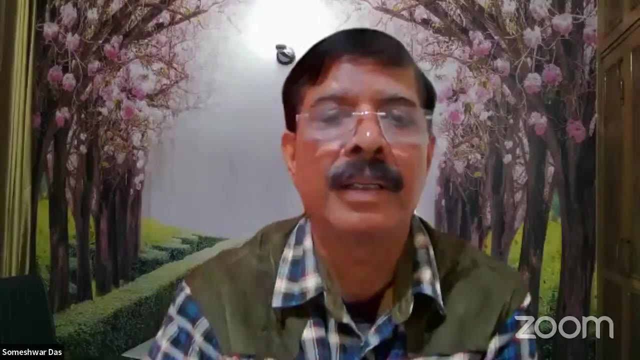 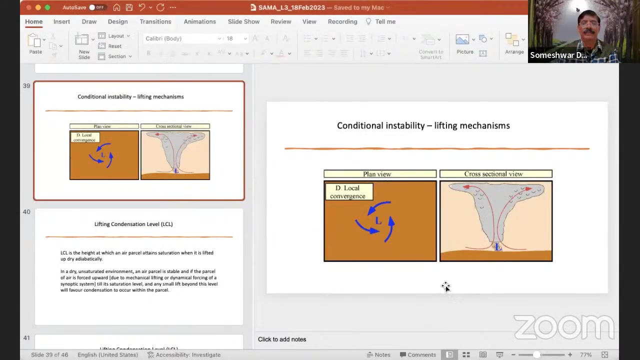 So we are live now. Yeah, we are live now. So we are live now. Yeah, Yes, Yes, click on the launch meeting, or no, no, no, no, no. now you just click to the ppt. oh, just click, yeah now. oh, i got it now. i got it so disappeared now. no, okay, yeah, yes, yes, this is fine, yeah. 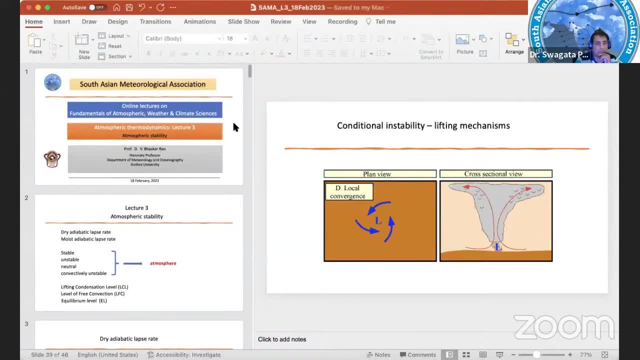 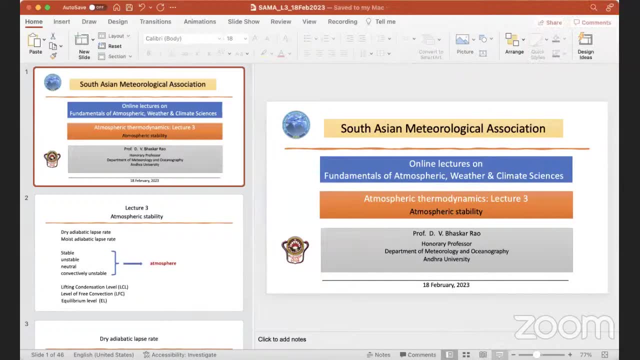 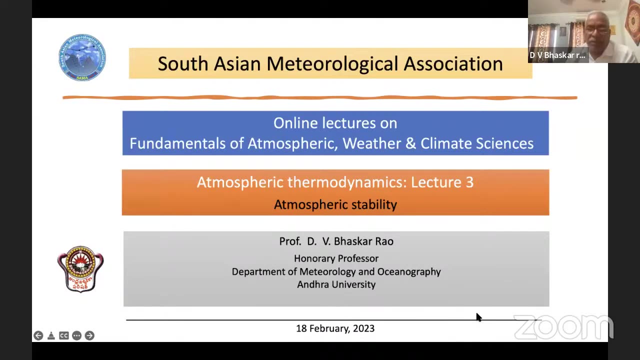 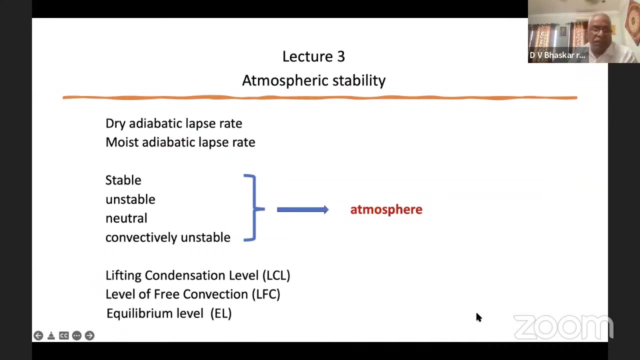 so can i start? yes, please. good afternoon everyone. this is my third lecture in the series on atmospheric thermodynamics, and today's topic is atmospheric stability. i will be speaking on certain aspects of atmospheric thermodynamics. previously, in my first lecture, i have given the expressions- mathematical expressions- for dry adiabatic lapse rate and moist adiabatic lapse rate at that. 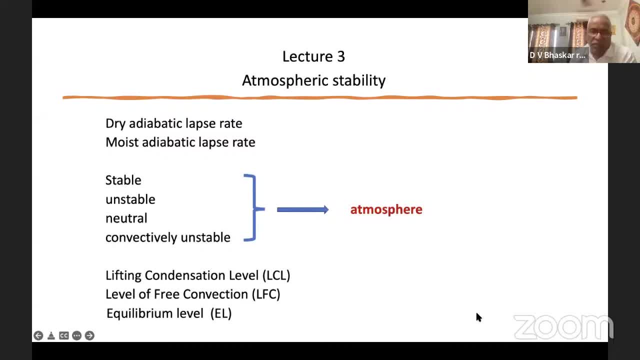 particular time. i have mentioned that i will show the mathematical derivation briefly, how to get them, and i will first work out these two. what are the expressions for dry adiabatic lapse rate, moist adiabatic lapse rate? and then i will go on to the stability. i will discuss about stable, unstable, neutral and 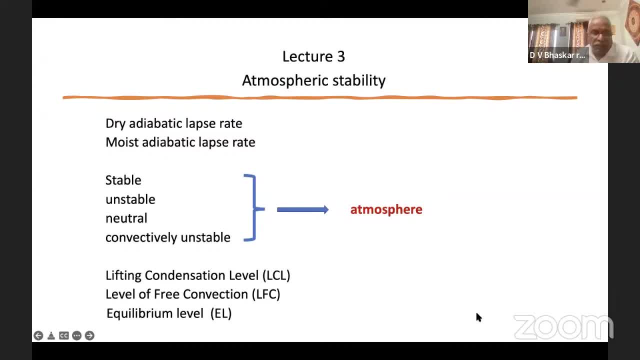 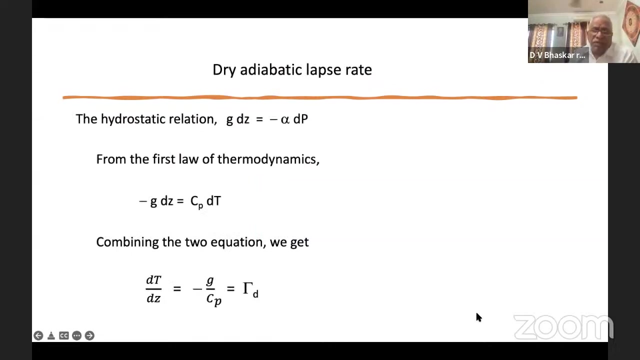 conditionally unstable atmospheres. and also later i will speak about lifting condensation. yes, please go ahead, sir. lifting condensation level, level of free convection and equilibrium level. so these are the things which i would cover today. first, the dry adiabatic lapse rate, because previously i have mentioned, we are talking 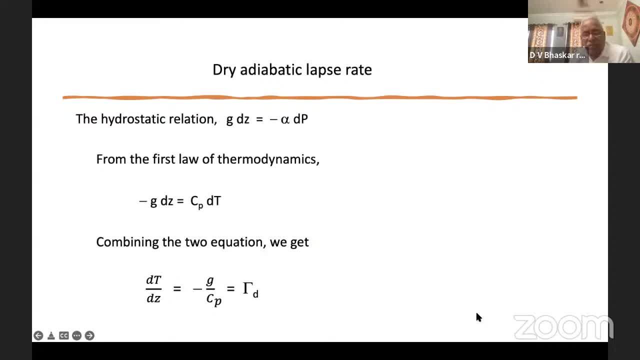 about when the thermodynamics has started. there are two important concepts. one is the air parcel. the concept of the air parcel and how it would move about in the atmosphere and how the temperatures decrease with height. we have seen that temperatures decrease with height, but at what rate and what? 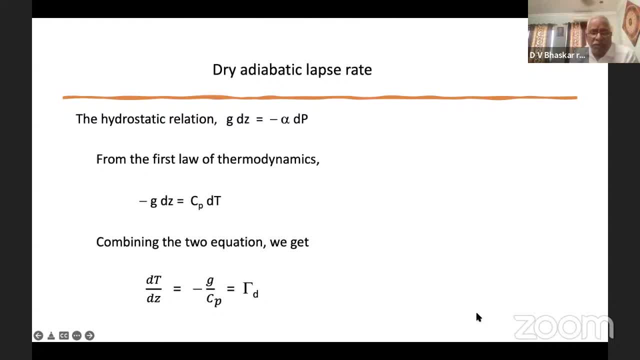 particular kind of atmospheres, because in the dry atmosphere- moist, dry and saturated and fully saturated atmospheres- i have gained the expressions for these three, but most importantly purely dry and saturated and dry atmosphere and the moist. i have given you some lapse rate expressions, so first i will show you. 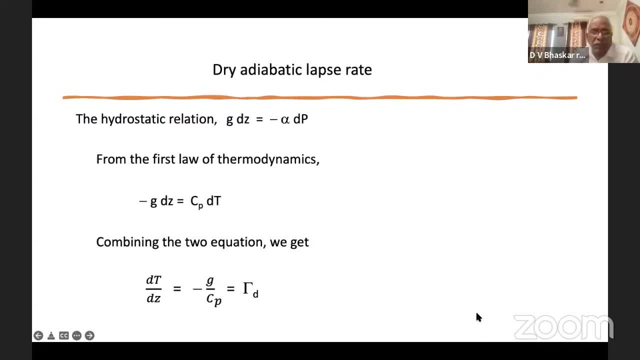 how to get an expression for the dry adiabatic lapse rate. we start with the hydrostatic relation, the level of the thermodynamics, pretty much the same as the flow rate, and then the speed in the atmosphere region. so we start with the flow rate. i will show you what is the flow rateという. 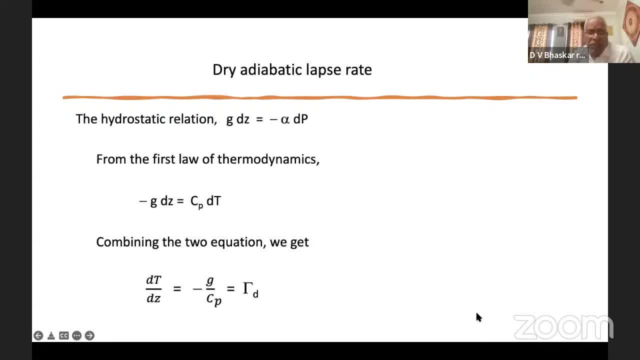 how is the flow rate now? the flow rate is the same. basically, it is just a so relatively large graph and it is really simple, just a small graph. but instead we come up to the flow rate, which is: the flow rate is equal to g dz, and that means g dz is equal to minus alpha into dp, or dp is. 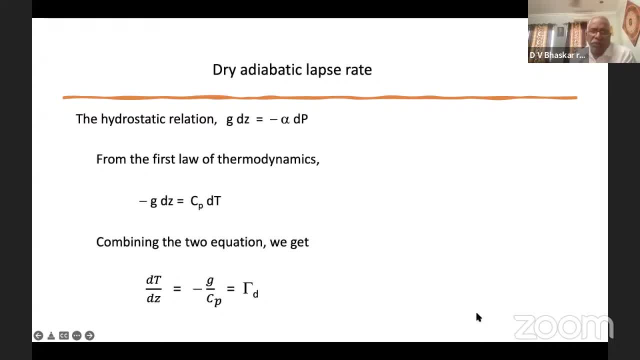 equal to minus g, rho d z. these things we know, and from the first law of thermodynamics we know that we take it as zero. So Cp dt will be equal to minus G dz. Combining the hydrostatic expression and the first law of thermodynamics. these two expressions we combine, we see that it is. 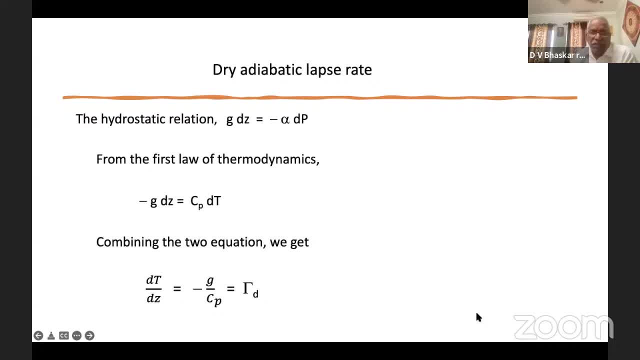 dt by dz is equal to minus G by Cp. That is the expression for dry adiabatic lapse rate. So we got an expression for the rate of temperature with height in a dry atmosphere and it is being given by minus of G's acceleration due to gravity In the denominator. 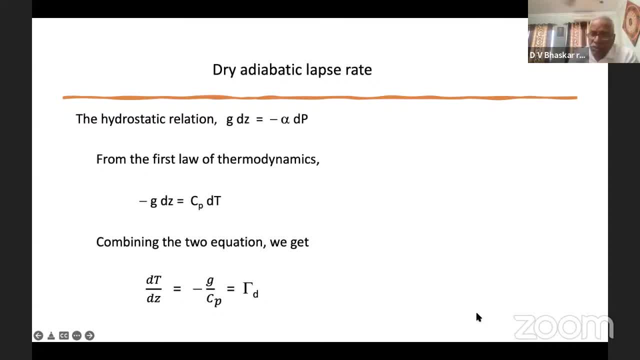 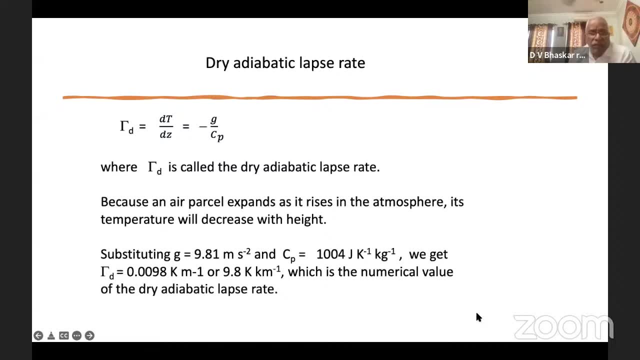 we have the Cp-specified constant pressure. So this is the expression. The derivation is very simple. I have shown you. And we know the values of G, We know the value of Cp. G is equal to 9.81 meter per second square and Cp is 1,400.. 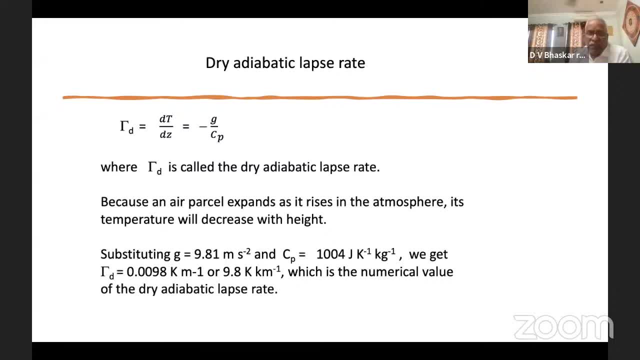 Joules per kilogram per degree Kelvin And substituting them we will get the value of dry adiabatic lapse rate as equal to 9.8 degrees Kelvin per kilometer. And this is the value for minus G by Cp. So more or less tau d value is constant. The dry adiabatic lapse rate value is 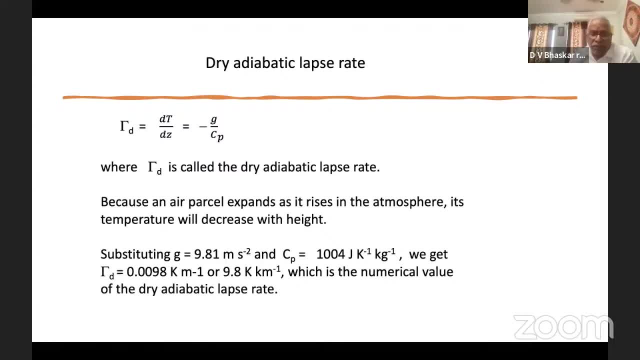 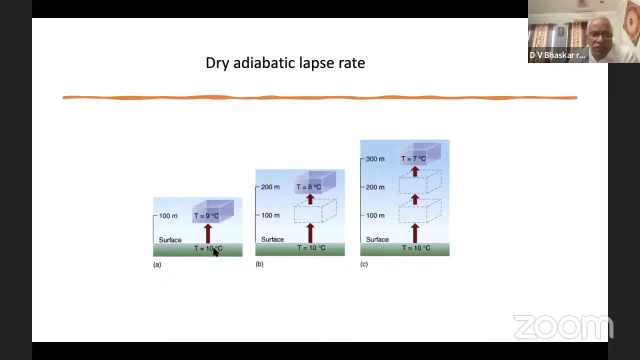 constant, which is 9.8 degrees Kelvin per kilometer. So if you use this small cartoon, it shows if you have the value at the surface and if you go to 100 meters, then 2 degrees have decreased. Those 8 parts will have the value of 9 degrees centigrade, So 1 degree. 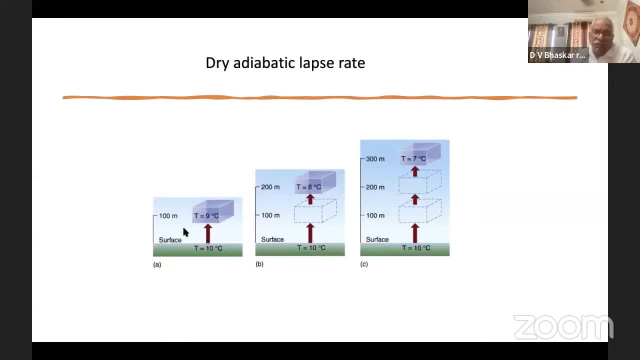 centigrade has fallen in 100 meters, So approximately in 1 kilometer, about 10 degrees centigrade. So that is what it is shown And if you go 200 meters, the 10 degrees centigrade, the. 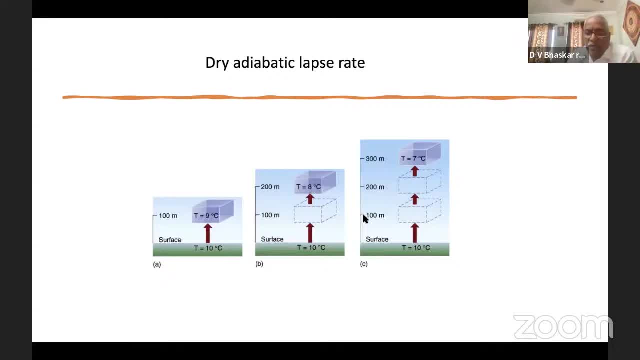 parcel will attain a value of 8 degrees centigrade approximately, And like that if you go to 300 meters it is about 7 degrees centigrade. So the rate of decrease of the parcel temperature with height in a dry atmosphere- dry atmosphere, the parcel is absolutely dry. then you will. 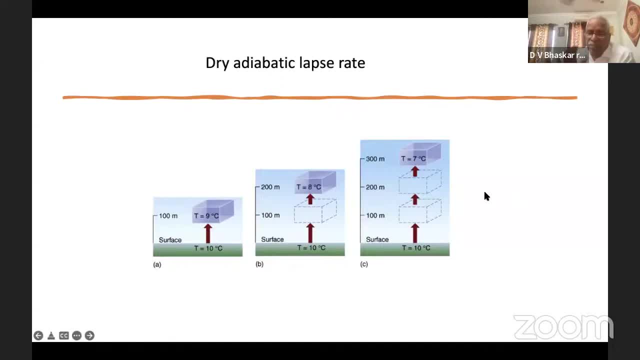 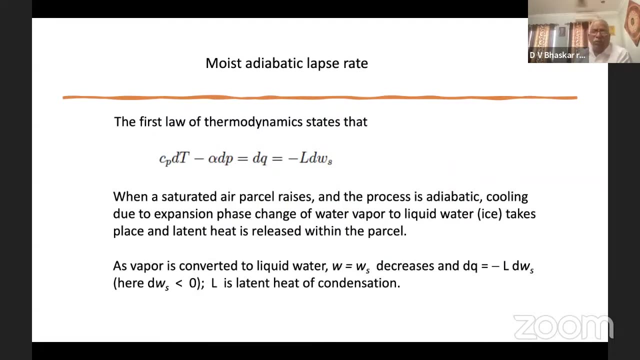 have. the degree of decrease is approximately approximately 0.9, accurately, 0.98 degrees Kelvin per kilometer, or approximately 1 degree centigrade Kelvin per 100 meters. So we go to moist adiabatic lapse rate. Again, we start with. 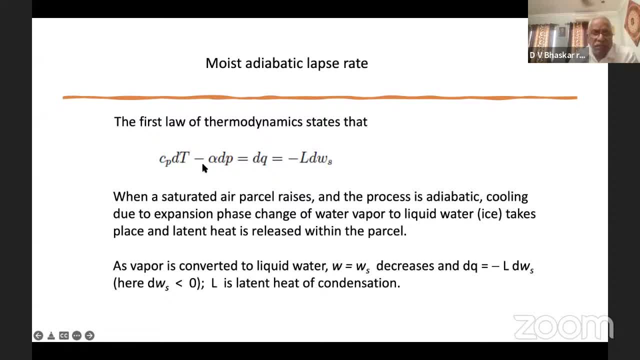 the thermo thermodynamics first law of thermodynamics. As I said before, Cp, dT minus alpha dP is equal to dQ, But in this case anyway, we have the dQ as equal to minus L into dWs. Ws is the mixing ratio of the water and air. 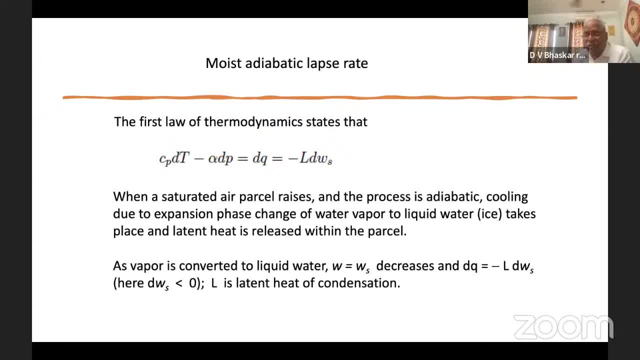 DQ is the mixing ratio of the water vapor. Moist. adiabatic lapse rate means we are now considering how the rate of change of temperature with height would be when the parcel is completely saturated. So that is the situation we have. We are trying to check how to get an expression. 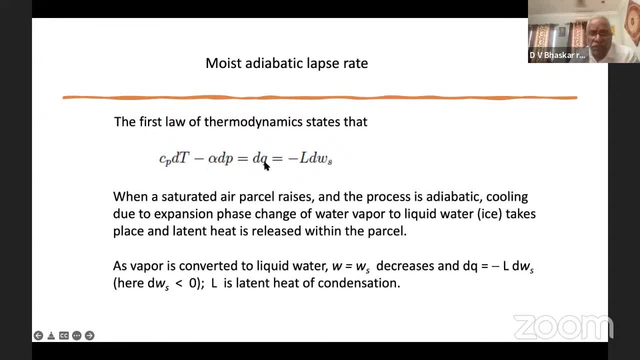 for that. So, first, law of thermodynamics, because this dQ is how to get the expression. dQ is the heat change, But that can. that is written as the change in the temperature of the parcel. What is the difference? It is because you have to measure the temperature. 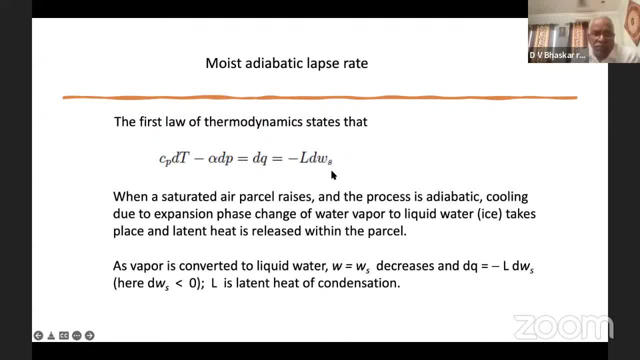 with the temperature. we want to measure. because of the temperature, we want to measure heat or the moisture, we want to measure heat And we measure heat. it has to do with the temperature, water vapor content, how, how it happens. so when a saturated air parcel rises, 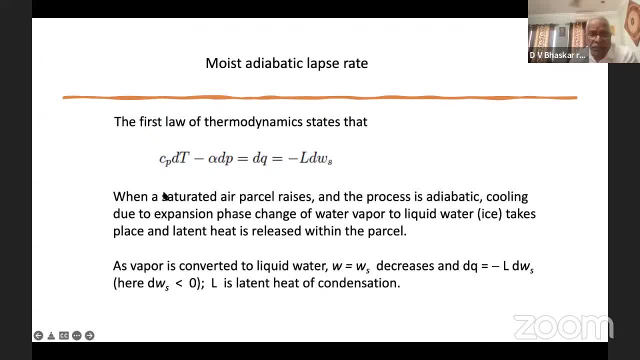 in a saturated air force. this is very important for you to remember because we are considering the saturated adiabatic lapse rate. as the saturated air parcel rises and the process is adiabatic, that means there is no heat, heat exchange between the parcel and the. 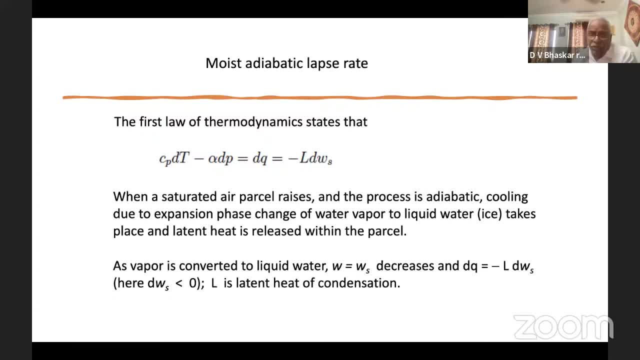 environment. the cooling due to the expansion. that means there is a phase change of the water vapor to liquid water. so because of the cooling there will be condensation within the air parcel. so there is a phase change of water vapor to liquid water and any phase change from water vapor to 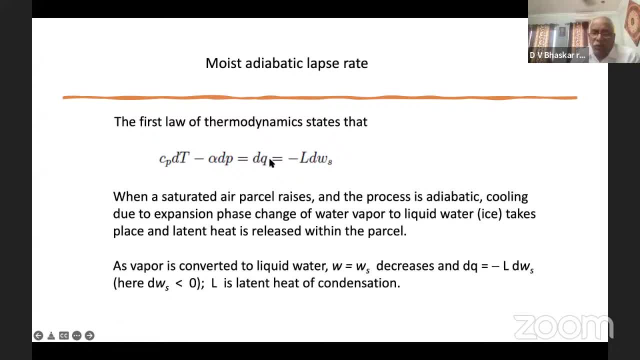 liquid water, we will have the latent heat released. that is what is written here: latent heat and how much of the heat is being released, and you the. if the air is, if the vapor is converted to liquid water anyway, it is saturated w. that's mixing ratio is equal to saturation value and the decrease is dq is minus lws, that is. 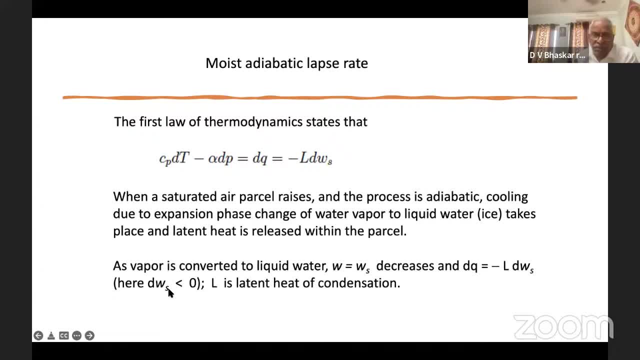 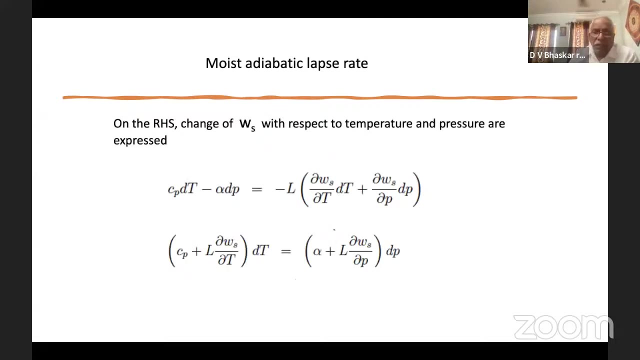 dws, the change of the saturation mixing ratio is less than zero, so it comes down, and the l is the latent heat of condensation. so we can write the first law of thermodynamics in this way: cp dt minus alpha dp is equal to minus l dws and the, the, the ws. now we are going to see. 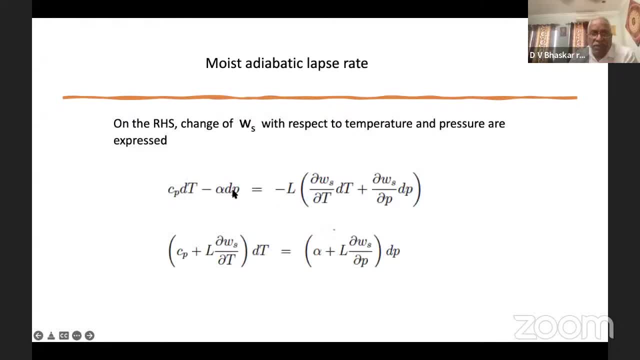 how it changes. cp, dt and left hand side is same. right hand side we have the dws. so now i am writing a mathematical expression: how ws changes with temperature and how ws changes with a pressure, because the saturation value depends on both of them. So the first on the right-hand side. 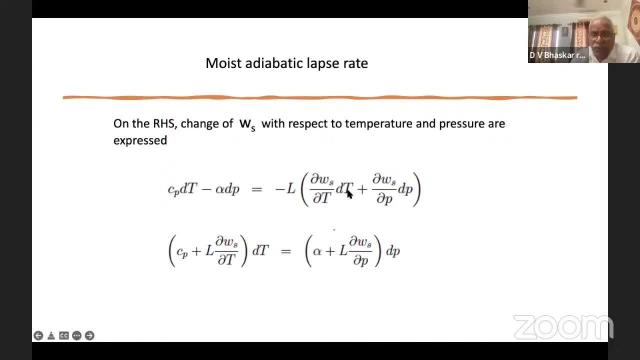 the Ws is being written: dou Ws by dou T into dt for a small change in the temperature, dou Ws by dou P into dp. So this came as to find the change of the dWs. So these two now can be, can be manipulated. bring down these terms of the dt onto the left-hand. 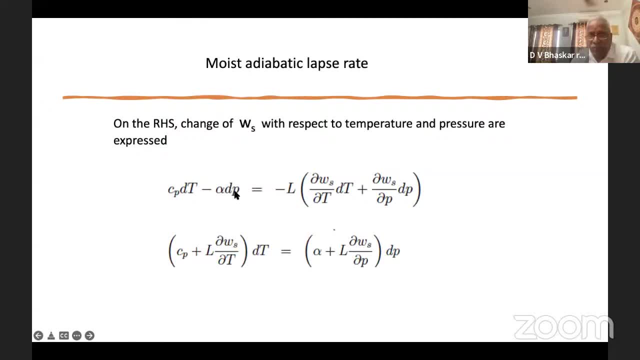 side. take the terms of the terms of the dp onto the right-hand side. now we will see: Cp plus L into dou by dou T of Ws into dt is equal to alpha plus L into dou by dou P of Ws, all of dp. So we. 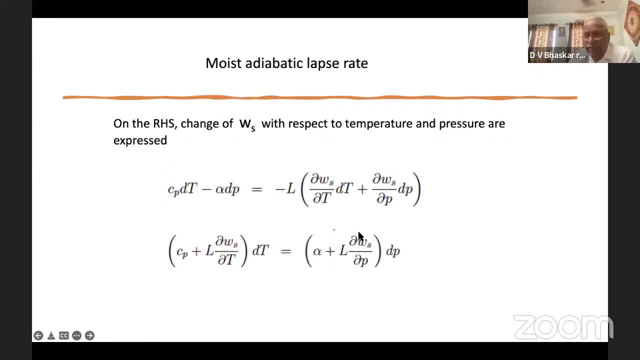 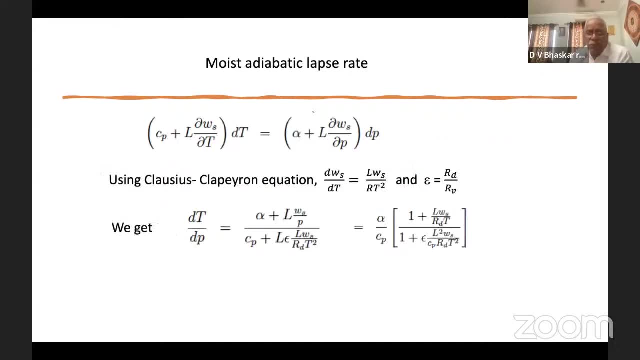 have just rearranged the terms on the left and right-hand sides to bifurcate the terms related to the dt and dp, So using the Clausius-Clapeyron equation. so we know the famous Clausius-Clapeyron it gives you. 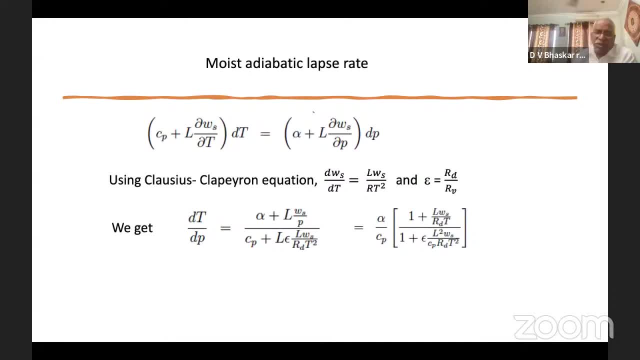 how the mixing ratio or the water vapor content changes with respect to temperature. So there are- this expression is from the Clausius-Clapeyron equation- d by dt of Ws is equal to L into Ws by RT square. And we also know epsilon, the ratio of the gas constants to the dry and water vapor. 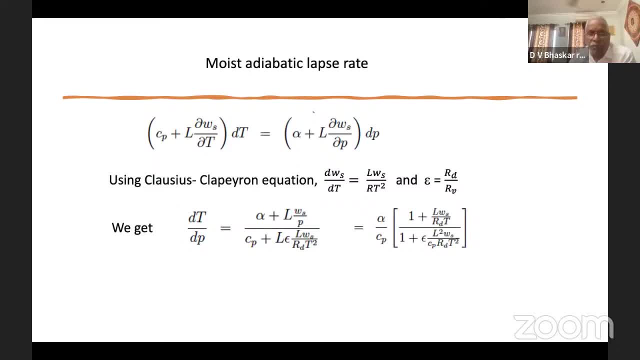 we know the epsilon previously. I presume that you know that the ratio I have shown you in the first lecture what is the value of epsilon, about 0.622.. And this expression now, by substituting this dW by S, by dt, we will have in the, in the denominator, in the 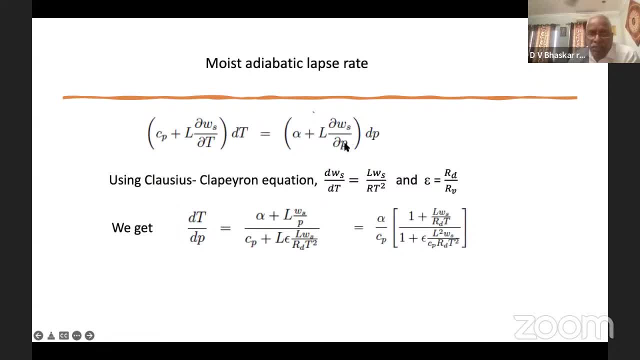 numerator we have dWs by dp as Ws by P and in the denominator dou Ws by dou t. we have written this expression, So here this expression is being substituted. epsilon came in because this R is written in terms of epsilon and Rd, so that the reason why you get right here and here. so we. 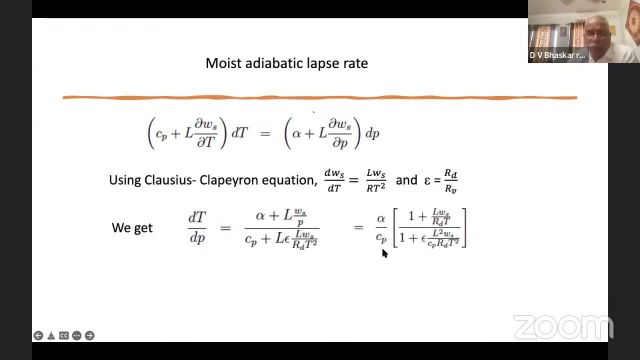 separate alpha by Cp. So we have written this expression and here, so we separate alpha by Cp And into the whole of this expression we will get 1 plus L Ws by R dt by 1 plus epsilon into L square, Ws by Cp, Rd, t square. So this can be written very easily from this expression substituting: 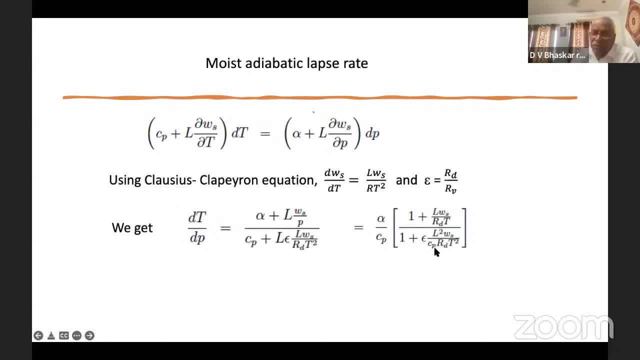 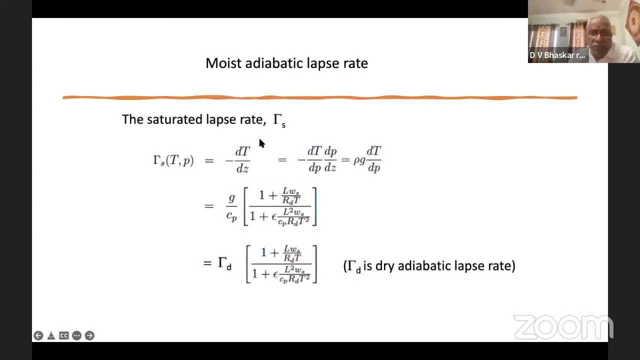 this and using this we will get this expression for dt by dp. And the saturated adiabatic lapse rate should be equal to minus dt by dz, So that we write it as minus dt by dp into dp by dz. So that is equal to g rho into dt by dp. So now substitute for dt by dp from here. 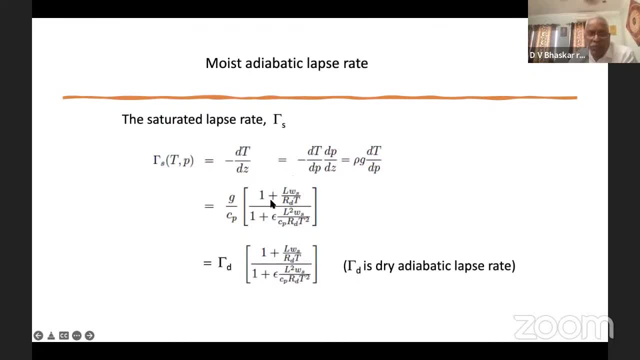 and we get this expression g by Cp into some place: 1 plus L Ws by Rd t in the numerator and in the denominator, 1 plus epsilon into L square, Ws by Cp, Rd t square. So. but we know already that g by Cp is the dry adiabatic lapse rate, So tau s the saturated. 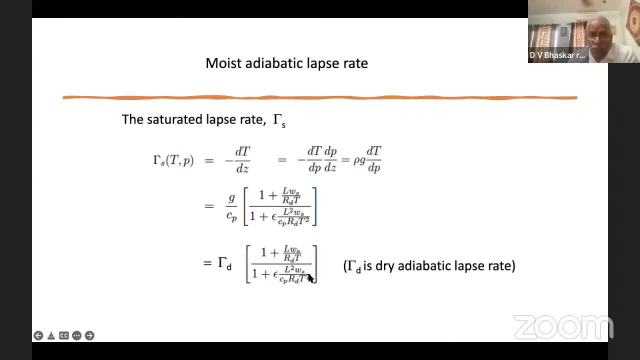 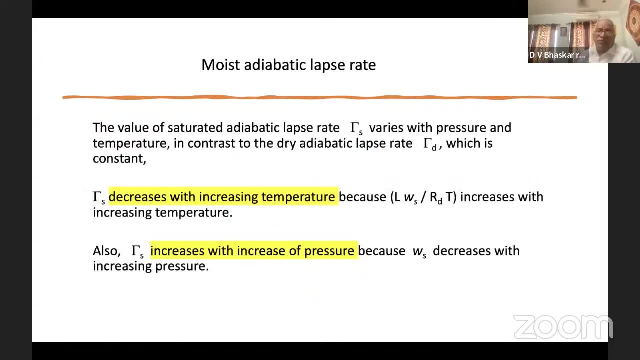 adiabatic lapse rate is equal to tau d into something. what is going to be the numerator was what is going to be the denominator. Now we can see its characteristics very easily: The, unlike the dry adiabatic lapse rate, as I said, which is constant and has a value of 9.8 degrees. 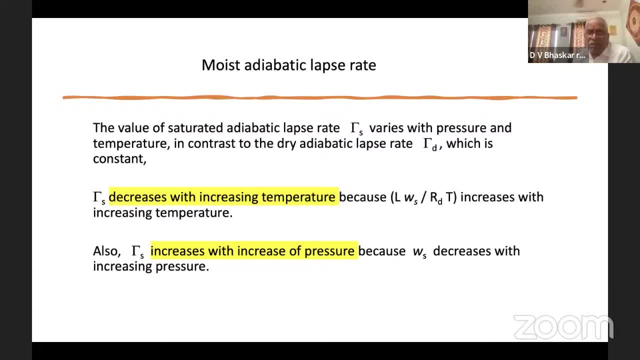 Kelvin per kilometer. the saturated adiabatic lapse rate varies with the pressure as well as temperature, as we see from the expression, And we see that the saturated adiabatic lapse rate decreases with the increasing temperature. because this particular L Ws by Rd t, which is there in the 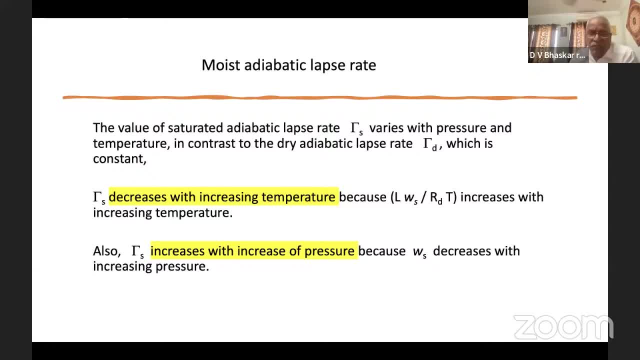 1 plus denominator way. that increases with the temperature value. So when the that increases, the denominator value will be more and then so tau s would be. tau s would decrease. Similarly, saturated adiabatic lapse rate increases with the increase of pressure. 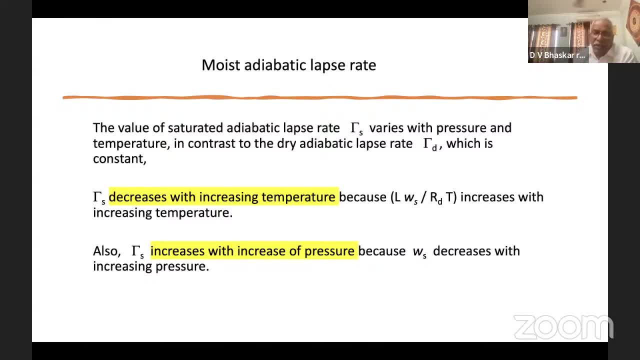 because we have Ws by P in the numerator, and if P increases then the 1 plus that value becomes smaller, and so the, the 1 plus a smaller value- 1 plus Ws by Rd, t plus Ws by P in the numerator, that will be smaller and so you will have the tau s to be. 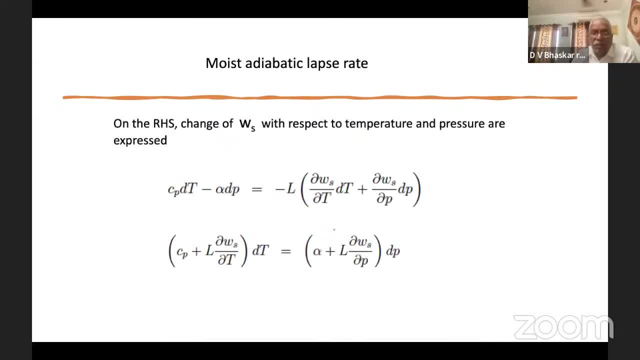 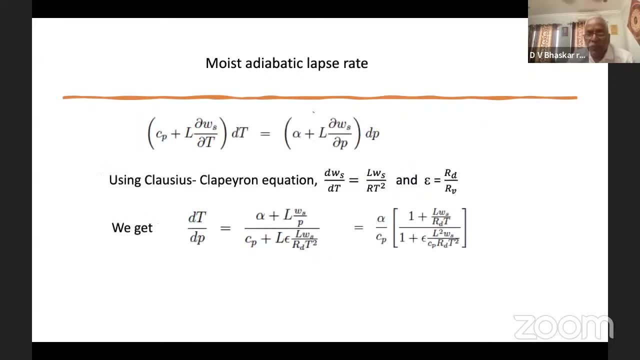 much more So here, in this expression. so here, here, here, this Ws by P. if you see this, if the pressure is more, if the pressure is increasing, this value would be, would be this smaller, this, this Ws. so we will have the, the smaller value here, and 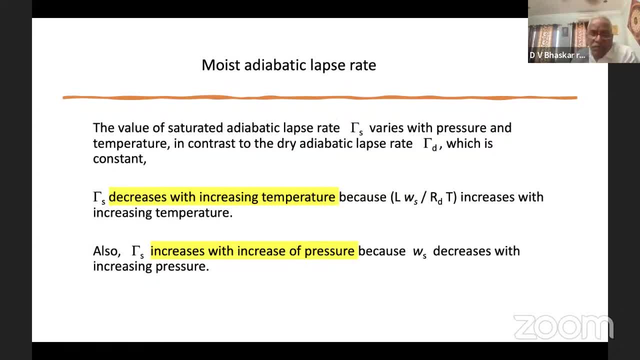 so tau s increases when you have the pressure increased, because Ws decreases with the increasing pressure. So Ws is, as you know, Ws is equal to epsilon E by P, epsilon E by P. So that particular expression gives us the clue: tau s the saturated. 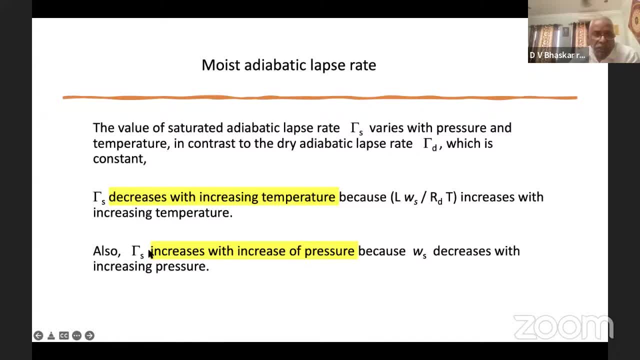 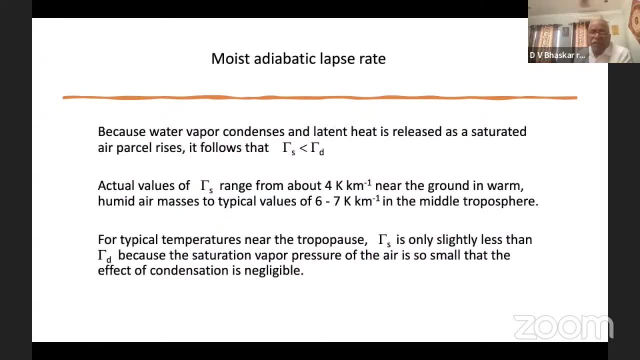 adiabatic lapse rate decreases with increasing temperature. saturated adiabatic lapse rate increases with the increase of the pressure and, most importantly, the saturated adiabatic lapse rate is always less than the tau s. So that particular expression gives us the clue tau s. the saturated adiabatic lapse rate decreases with increasing temperature. saturated adiabatic lapse rate increases with the increase of the pressure and, most importantly, the saturated adiabatic lapse rate is always less than the tau s. 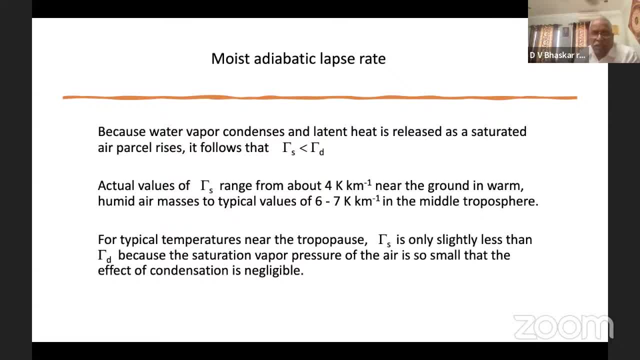 rate is always less than the tau d. less than the tau d because when water vapor condenses, there is a latent heat that is released. it will have, it will actually heat the parcel inside. so when the parcel starts condensation, um, then latent heat is released. that latent heat is used to warm up the parcel. so the parcel is. warmer than what it could have been without a con, without condensation, So tau s is always less than tau d in the atmosphere. normally the saturated adiabatic lapse rate values range from about four degrees Kelvin per kilometer near the ground in warm, humid air masses. 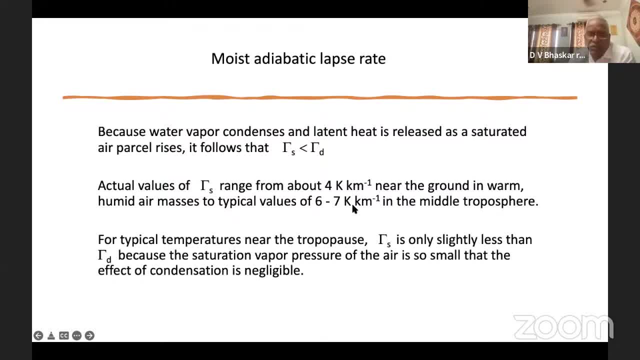 to typical values of six to seven degrees Kelvin per kilometer in the middle, middle, middle, A trobosphere where the humidity is very, very low and near the trippe pause. if NglO it will still go up because the humidity is very, very small. 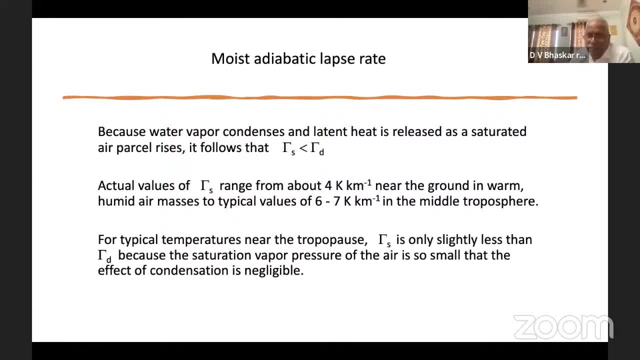 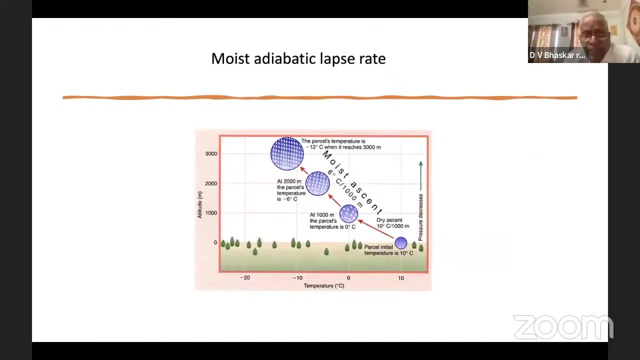 The TOAS, the difference between the saturated and dry adiabatic lacerates would be very, very small. However, TOAS is less than TODI at any time. So these are the things which I wanted to cover before we go to stability. 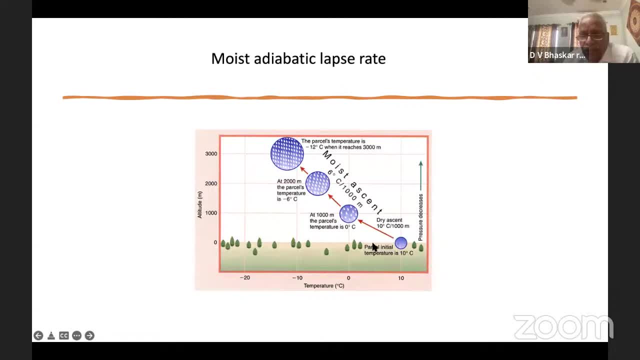 Anyway, you can see here the parcel. This is one curtain. So until it gets saturated it will be a dry ascent. So the temperature would decrease at about 10 degrees centigrade per kilometer, And after it gets saturated then it will be decreasing at about. 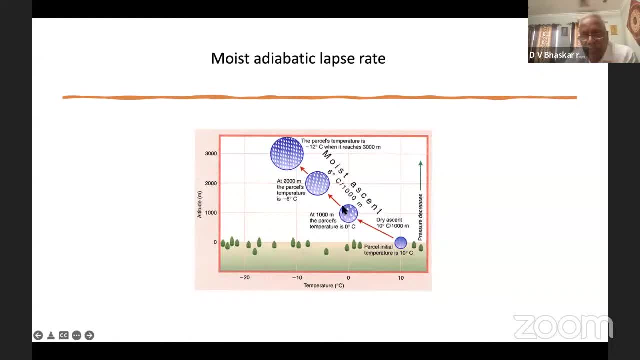 the moist adiabatic lacerate value. So you can see here the 10 degrees centigrade one kilometer. it became zero degrees Now it is saturated Now from here it is decreased. The temperature Decreases at six degrees centigrade per kilometer. 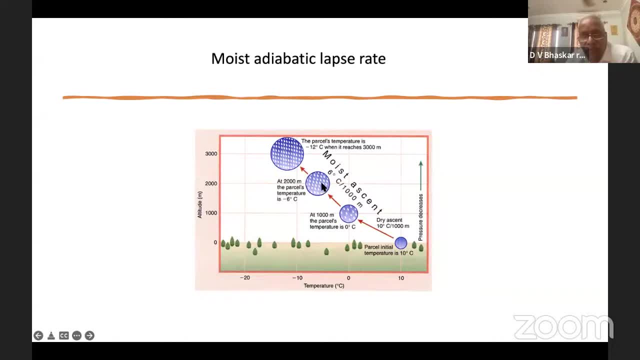 So from here, if you go to one kilometer more, it is minus six degrees, And if you go one kilometer still higher, it would be minus 12 degrees. So from zero we go to one, one, two and three. 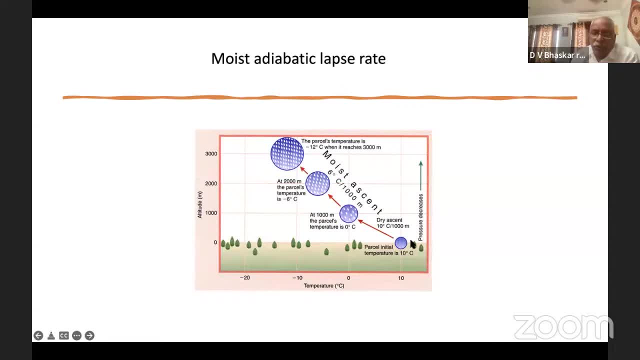 So zero, six and 12, as we see here. So from the surface to till the parcel gets saturated, it will be. the temperature will be decreasing. at dry adiabatic lacerate That is About 9.8 degrees centigrade per kilometer. 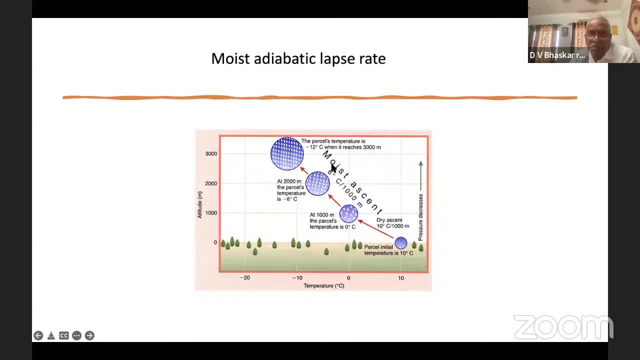 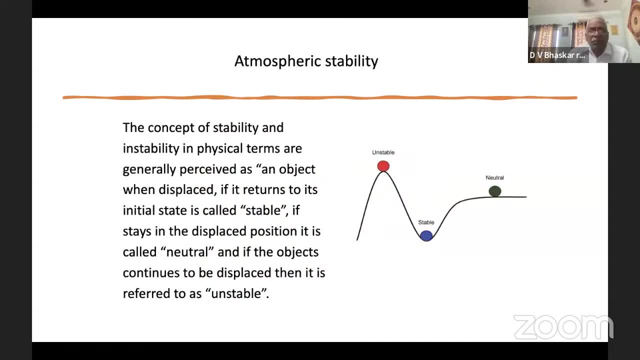 And above that, it would decrease at the moist adiabatic lacerate approximately six degrees centigrade or so. Now, uh, uh, I come to the stability. normally, uh uh, even in uh the fundamental physics, we talk about uh, stability and instability. 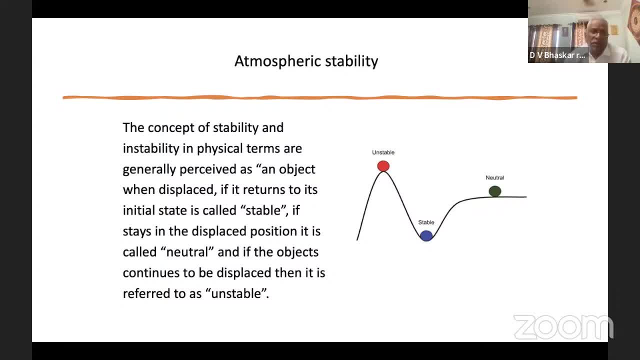 And normally it is um uh perceived, or normally it is understood that when uh an object is displaced from its original position, if it returns to its initial state it is called stable. If it stays in the displaced position it is neutral. 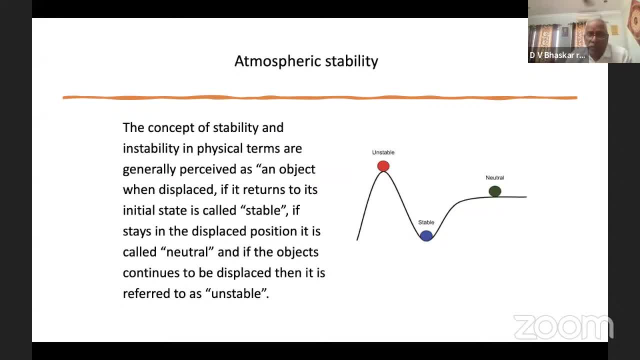 And if the object continues to move and then get displaced, then it is called unstable. That means if you disturb the, the, the moment of an object object and if it goes back to the initial state, then it will be stable and 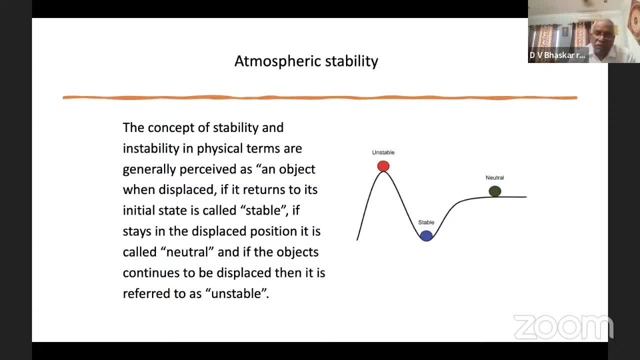 Uh, Uh, if you, if it stays in the- uh, displaced position, it is neutral. and if it continues to move it up, move about, then uh, it is unstable. you can see here, if the if the object is here, you just move up or he decide, decided to come back to the this state in this, in this particular case, you. 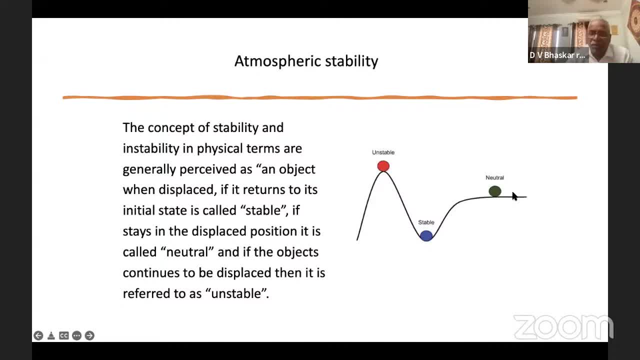 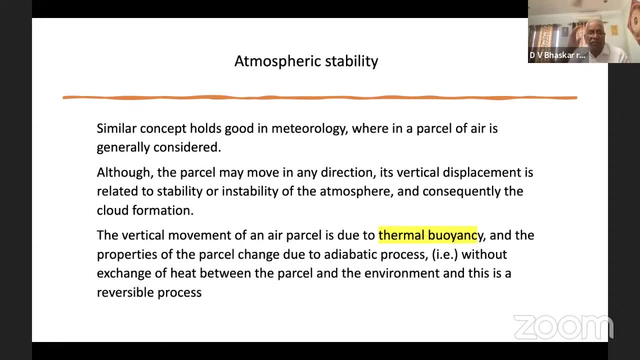 move the object. if you move, it doesn't uh move at all. it will be, it will stay in the displaced position. but here, if you just move it either way, it will fall down onto the other side. so it's basically a small picture to make. but uh, coming to our weather, 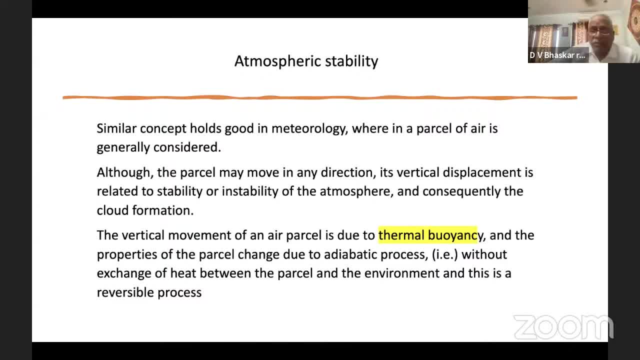 signs? uh, but we are. we are talking about the temperature and pressure rates, relations and an air parcel. so, uh, we have to see how the how the air parcel as it is moves in the atmosphere, whether it is going to be stable or unstable. that is a very vitally. 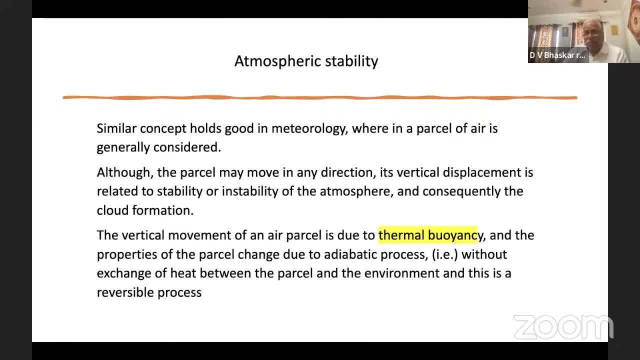 important for weather prediction to understand the state of the atmosphere. so if we say that if we move the parcel, so anyway the parcel may move in any direction, horizontally, vertically at all, but for the understanding of the stability and instability of the atmosphere, vertical direction displacement is, uh, the important is only only the vertical displacement is important to understand. 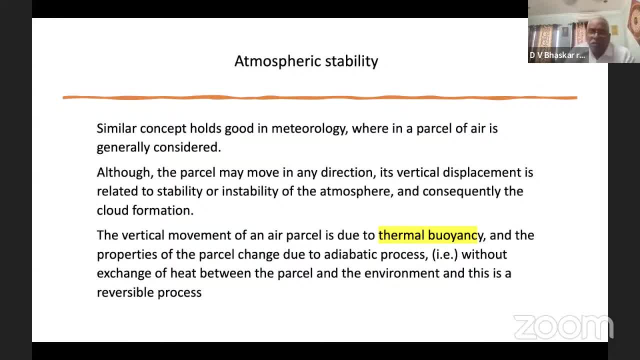 the stability or instability, because it is related to the formation of convection and clouds. so here we are. we are concerned mostly about the movement, or the air parcel movement in the vertical direction. so that's what we are going to talk about, and we know that the vertical movement of the parcel at any time is due to its thermal buoyancy. 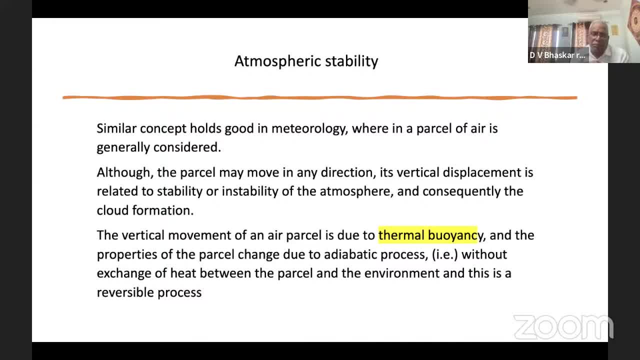 that means the, the state of the value of its temperature. so if it is warmer, then the. if it is warmer it will go up, if it is colder it will go down, comparatively with its surroundings. if a parcel, so the air parcel, the concept of the air parcel we are going to use time and again. 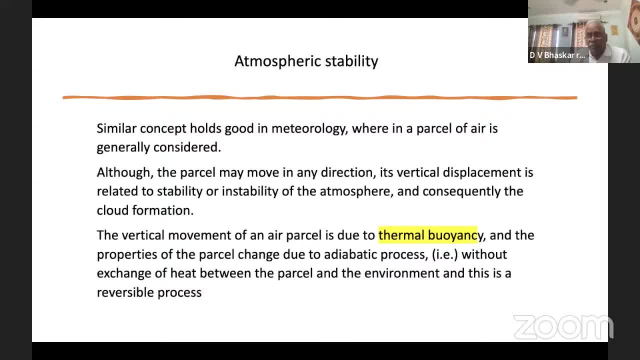 here we we consider an air parcel and the movement of the air parcel is clearly understood as purely due to its thermal buoyancy, that means its heat content and- and we are again, we are saying we are considering adiabatic process. that means the parcel and the 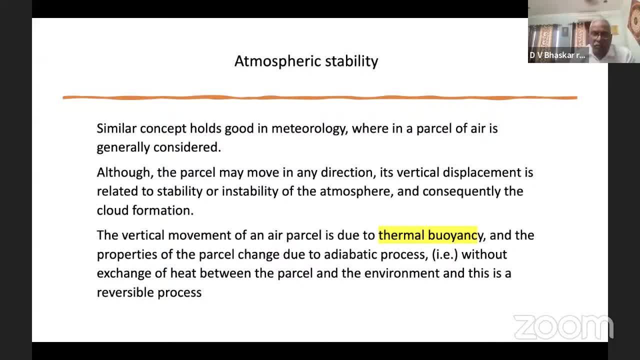 environment, the movement of the parcel emits the environment and the no exchange of heat between the parcel and the environment, and all so that this could be a reversible process. that means any change that is taking place can, can, can happen reversibly also. that means rivers also can happen. 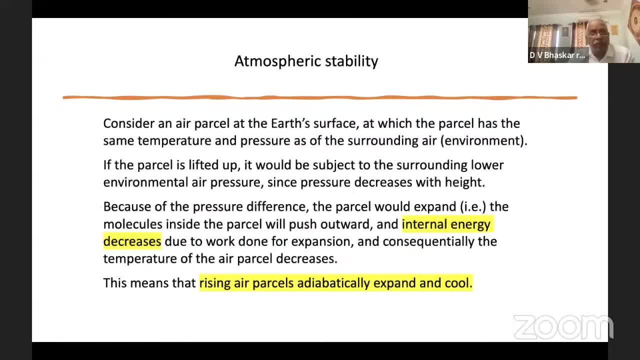 you will understand this as i explain a little more and more. so if we, if you consider, consider an air parcel at the earth surface, at the air surface, the air parcel, the temperature of the air parcel is the same as of the surrounding air. so it is, it is normally having the same characteristics of the surrounding air. so at 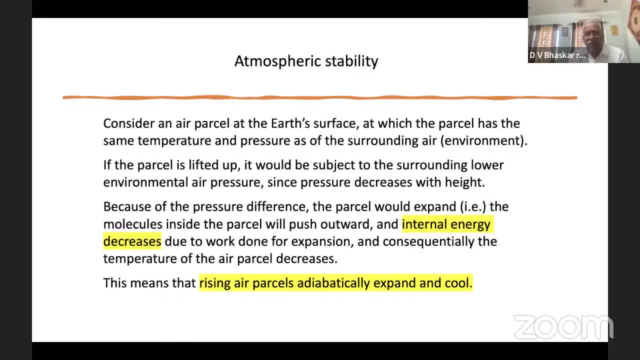 the surface, the air parcel is having the same temperature and pressure as of the environment. so that is the starting point. so now consider if the parcel is lifted up for any reason. so if we assume that the parcel is forced to rise, then it would be, the parcel will be subjected to. 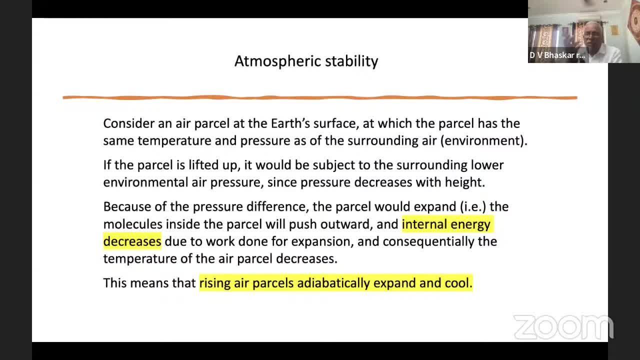 as as the parcel goes up goes up, then the pressure decreases with height. as the parcel is lifted up or it raises, the surrounding environmental pressure is lower and lower. it will be subjected to lower pressure. so at the surface the air parcel has certain temperature, temperature and pressure as of the surrounding air. But when the air parcel is lifted up, 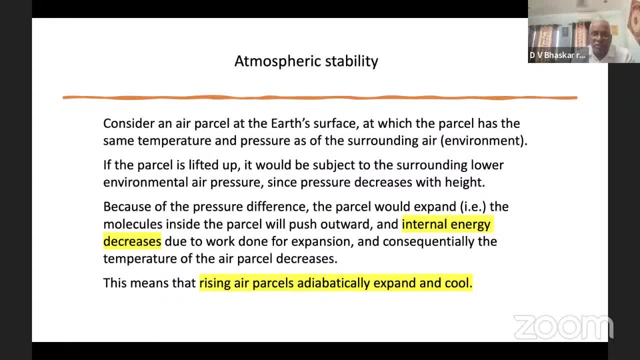 the environmental pressure is decreasing. So what happens is inside there is a pressure difference. the parcel would expand Outside the pressure outside the environment. the pressure is less than what it has inside the parcel and the parcel will try to expand, That is, the molecules inside. 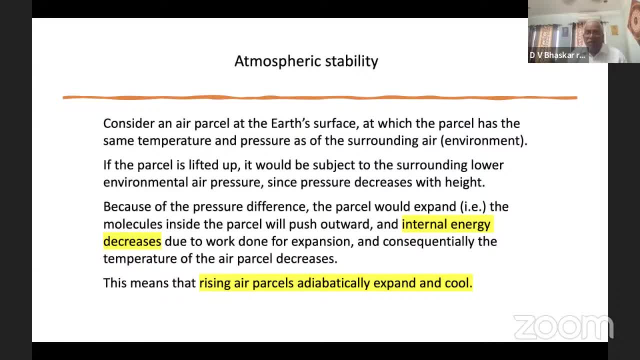 the parcel will try to push outward and in that process the internal energy decreases due to because it has to do some work, because the parcel has to get expanded, So area gets expanded, the volume actually increases. For that reason, because of the pressure difference, the parcel 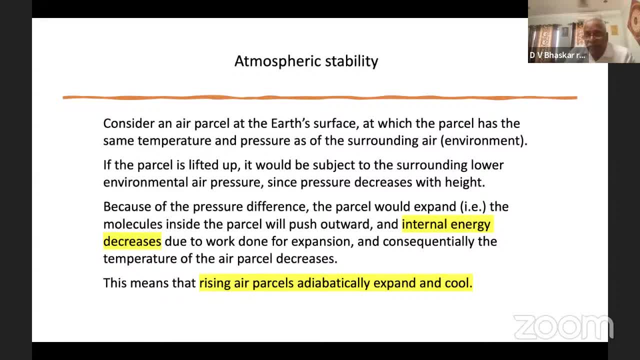 would expand and because of the work done for the expansion, the internal energy decreases. And so, because of the expansion, the internal energy decreases. So, because of the expansion, because of that, consequentially, the temperature of the parcel should decrease. So this is the 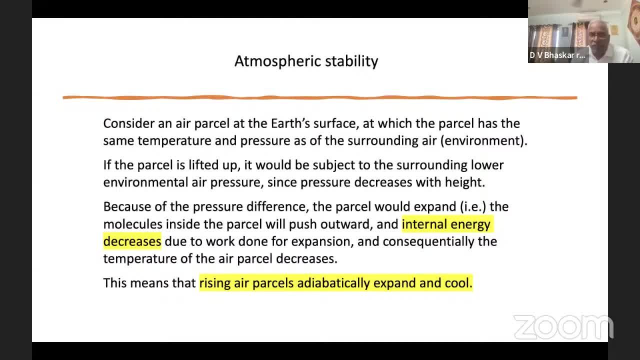 basic one. At the surface we have the air parcel with the same temperature and pressure as the environment. But when it is lifted adiabatically, that is, without any exchange of heat, then what happens is, as it moves up, it is subjected to lower pressure of the environment. 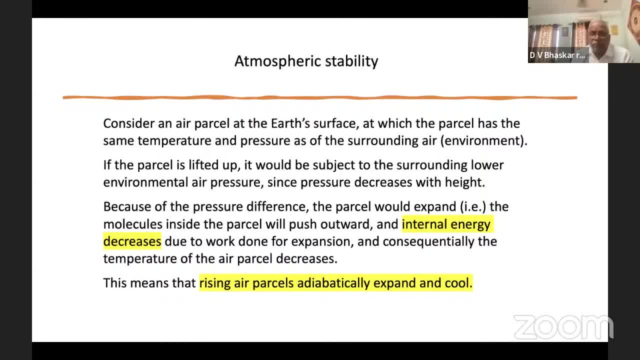 and the parcel will expand, because inside the parcel the air parcel will expand. So when it is lifted adiabatically, that is, without any exchange of heat, the pressure is a little more and outside the pressure is less. So it would. 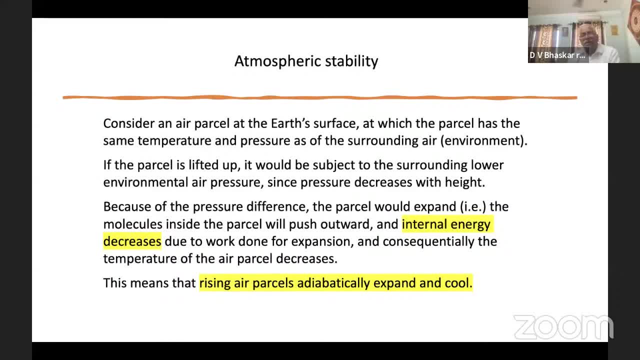 expand and in that process some work has to be done and the energy- internal energy- of the parcel decreases And so the temperature of the parcel decreases. So this is the basic process which we need to remember: how the raising parcel adiabatically. when a parcel raises adiabatically, 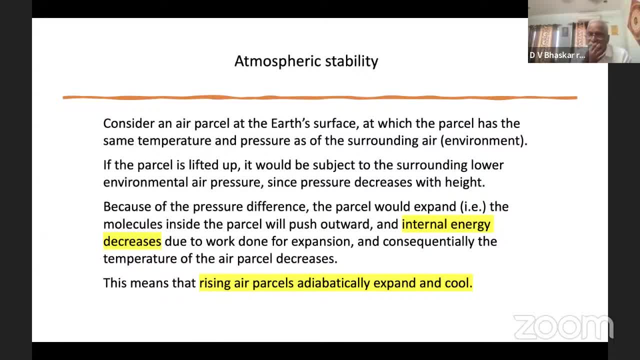 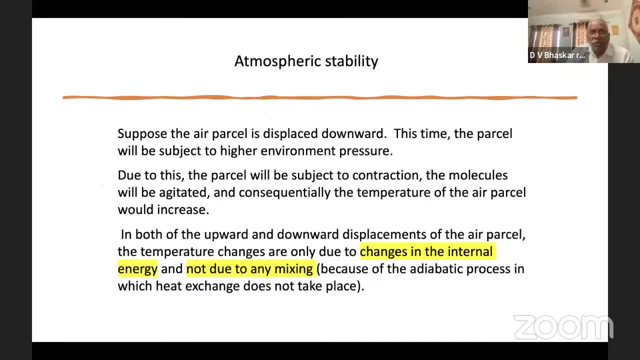 it will expand and cool because of it is subjected to lower pressures of the environment. So, conversely, if the air parcel is displaced downward from a higher level, this time the parcel will be subjected to the, so at that particular level. 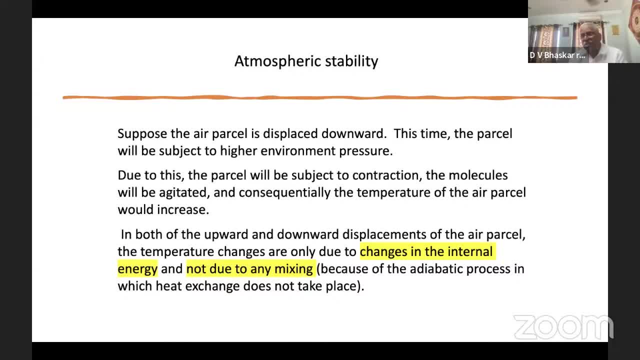 where we start. it has the inside, the parcel. it has the same pressure and same temperature. for example, at the same pressure, the same the temperature. let us say it is some value When it is brought down. when the parcel is brought down, what would happen is it would be subjected to higher. 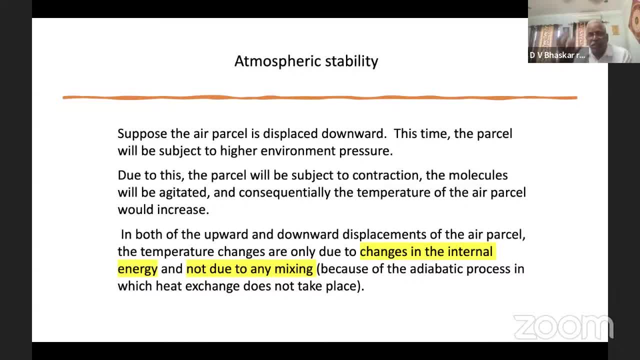 environmental pressure, So the parcel is being displaced downward. When it is brought downward, the it is subjected to higher environmental pressure relatively, and this will subject to, so there is a contraction, the contraction of the parcel. the parcel will be subject to. 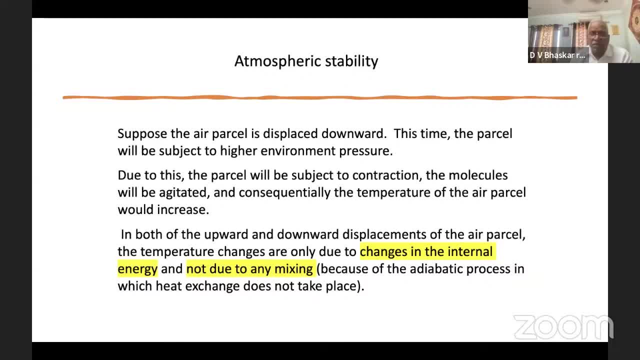 lesser volume all the molecules will have will get acidated and consequently the temperature will increase. So as we move the parcel down in the same way, adiabatically, what happens is the temperature of the parcel would increase at the same rate. 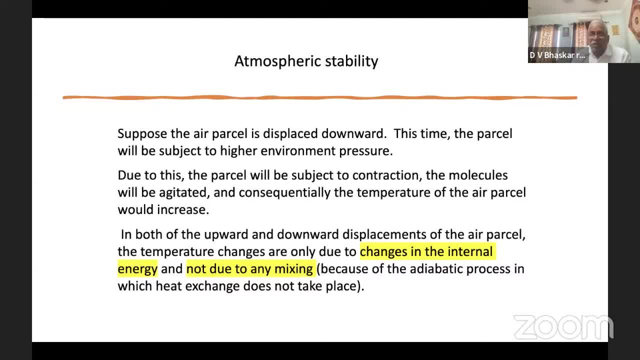 In both the upward and downward displacements, the that we have to remember that, in both of these upward and downward displacements we have discussed so far, the temperature changes are only due to, you do, the internal energy, valuing the internal energy. but 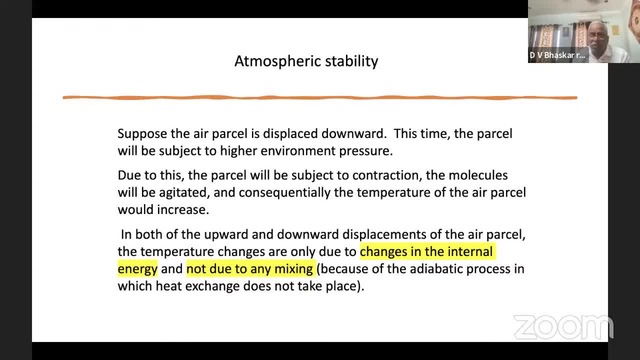 the temperature changes are only due to, due to the internal energy, valuing the internal energy, but not of any mixing, because this adiabatic process we're talking- we have to remember very importantly- it is not mixing with the environment at all. so, whatever the changes that take place, 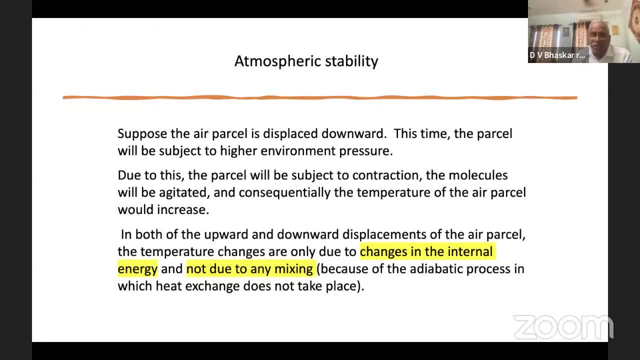 with regards to the temperature only because of either the expansion or the contraction of the parcel sub, and with respect to the difference in the pressures, and, consequentially, the temperature would rise, uh, in the, in the downward motion, and it would decrease when the parcel is being lifted upward. so this is a very important thing which we need to remember. so, uh, here it is. if it. 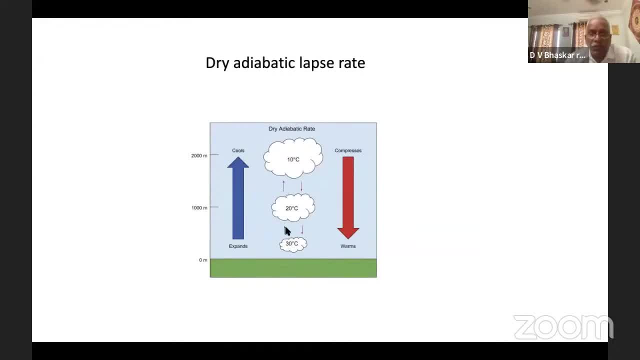 is the blue. the blue one shows as you move the parcel from uh lower to upper one, it actually decreases at uh 10 degrees centigrade per kilometer. so so, so it would be 30 degrees at the surface, at one kilometer it would be 20 degrees, and at 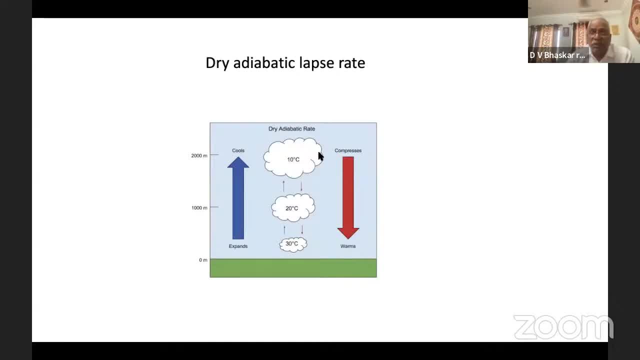 one, two kilometers, it would be 10 degrees centigrade. so again, if you want to compress this side, so it would be the same and then warms at the same rate. so this particular picture to show how the temperature would cool as it is lifted upwards and as it is, uh, displaced downwards, how? 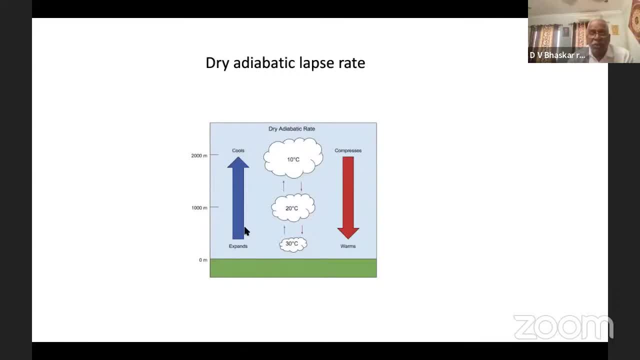 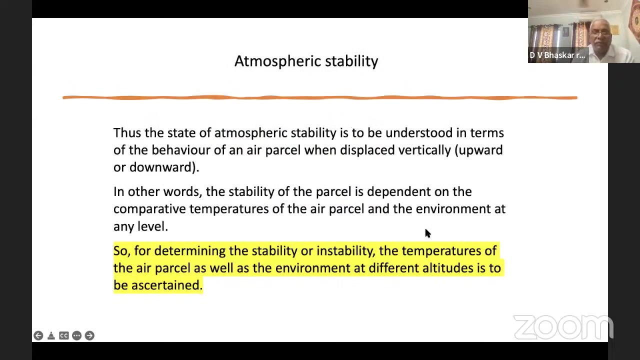 it warms. it compresses and warms. it is expands and cools. so there is an expansion and a cooling while the air parcel is being displaced upward, and there is compression and warming as the air parcel is being displaced downwards. so now we we have seen the displacement of the parcel. now we have seen the displacement. 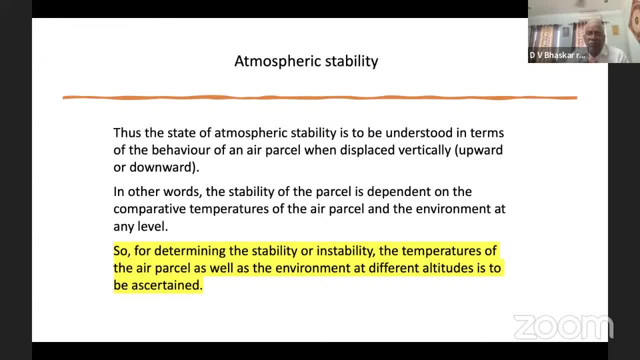 of the parcel and we see that the parcel is displaced vertically upward or downward, and downward. whatever it is, it is purely dependent, dependent on the difference in the temperatures of the air parcel with the environment. that means the, the moment, the, the, the way the particle, the air parcel, would move upward or downward is purely dependent on the temperatures of 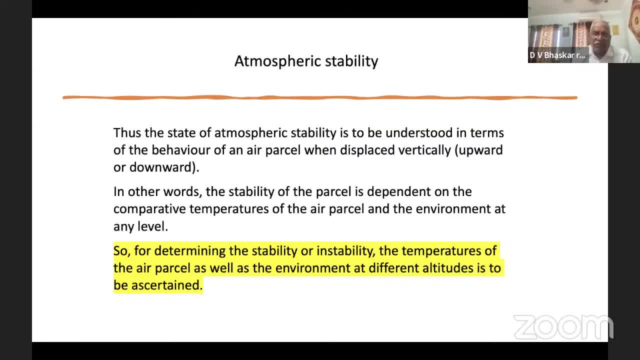 the air parcel and the surrounding environment at any level. so so this is, uh, the one important thing which we remember. so the the the moment of the parcel is essentially depend is dependent on the thermal buoyancy, that means, the temperatures of the air parcel as it changes within the air parcel, as it moves upward or downward, uh, with respect to 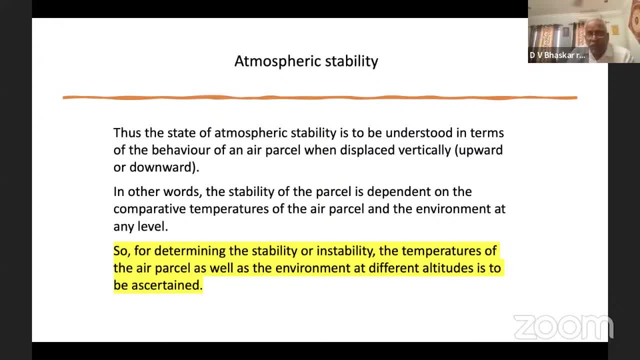 the environment. so we here know or clearly understand that for determining the stability or instability of the parcel, the temperatures of the, the temperatures of the air parcel, as well as the environment and different altitudes, is to be known. so if we want to have an understanding of this, of whether the air parcel or the atmosphere, 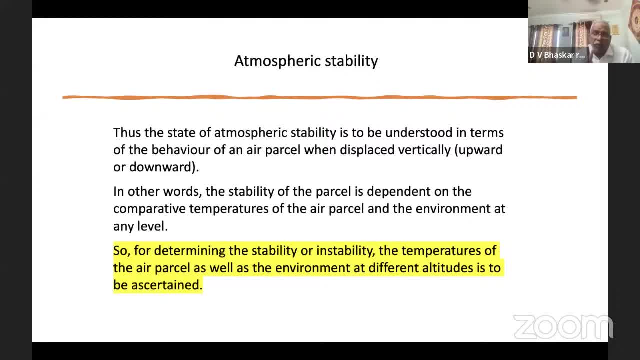 is stable or unstable. we need to have two: the temperatures of the air parcel as well as the temperatures of the surrounding environment at different altitudes is to be known, then, if we know these values of the temperatures of the air parcel and the environment at different altitudes. 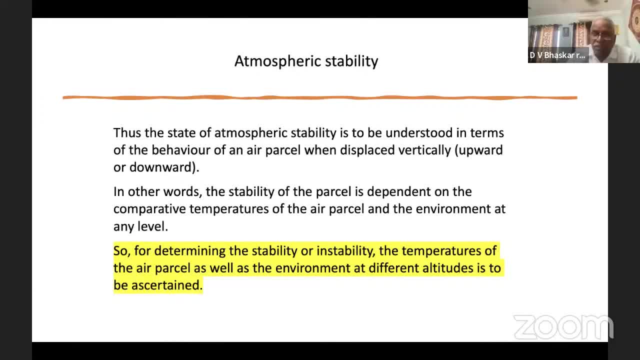 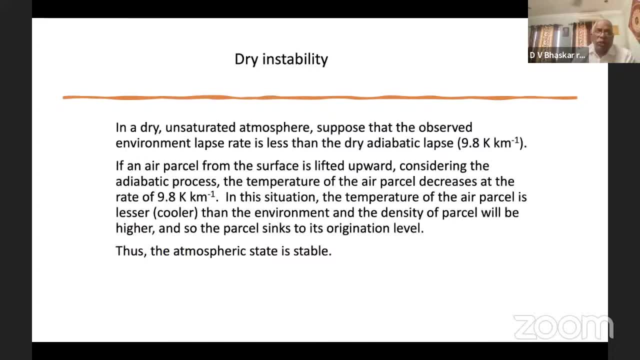 then we will be able to determine the stability or instability of the environment at that particular time at that particular location. so now, uh, so this is broadly, this is broadly a concept of the stability in the atmosphere now we see, in a dry atmosphere, in a dry unsaturated atmosphere. 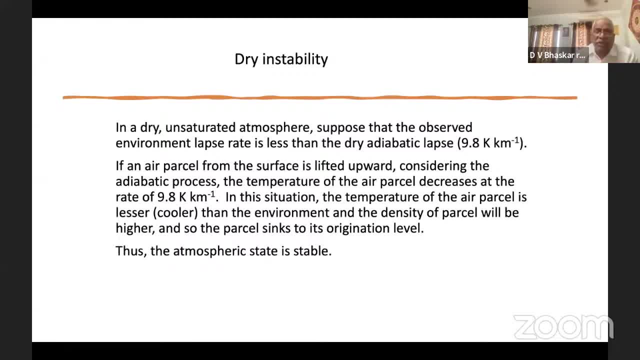 so step one: in a dry, unsaturated atmosphere, if the observed environment collapse rate is less than the dry adiabatic collapse rate, that means we have the surface temperature value and pressure value at the, at the surface, for example at the surface, and we know the. 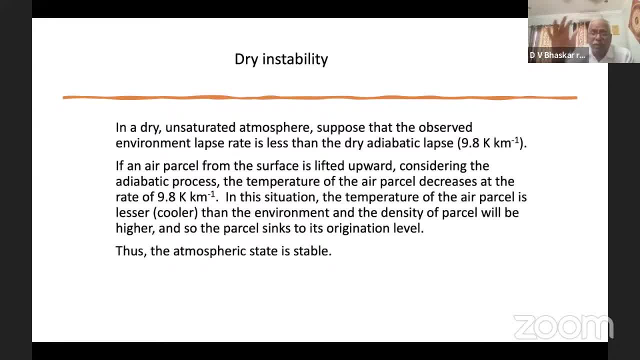 observed values of the temperature of the environment In the environment. somehow we make the observations. I'm not going to tell you here how to make the observations. Normally, radio sound observations are the most popular kind of thing that's being used to make the observations. 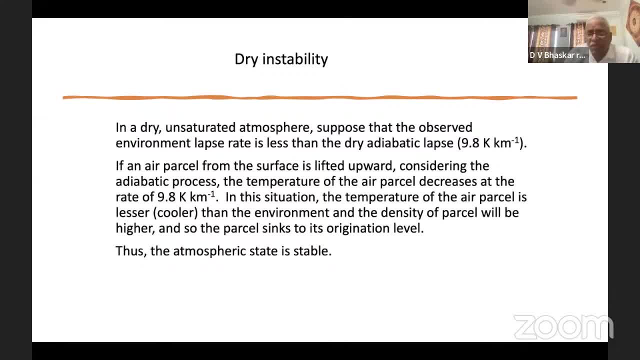 of temperature et cetera. Previously in my previous lecture I have mentioned this radio sound balloon observations give us the vertical temperature stratification in addition to other, even humidity, other things. So here we know, we have the observations observed. 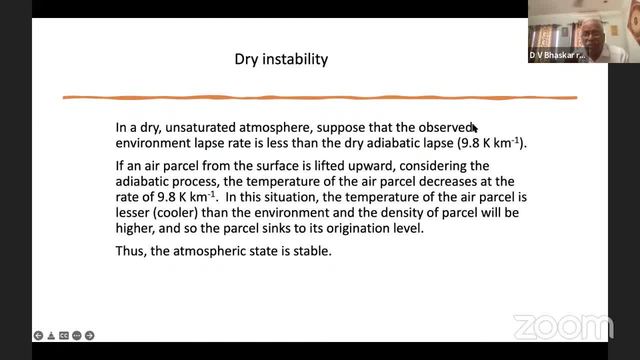 This is observed here. So this is very important. This observed environmental curve- we know how the temperature has its values in the environment at different altitudes- is from the observations. okay, Now, in that particular kind of an environment, if the environment lapse rate. 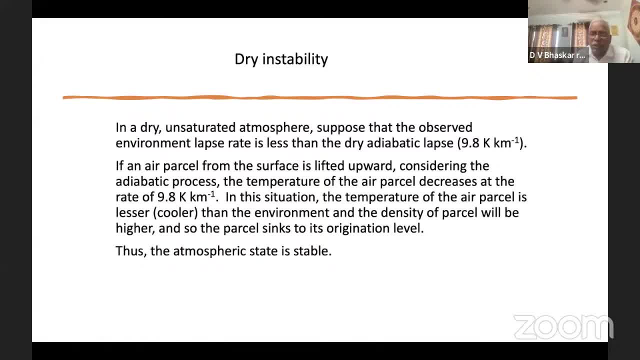 that means the environment curve shows a value less than the dry adiabatic lapse rate. That means when you have the values of the temperature at different altitudes then you can calculate the lapse rate of the environment. So if it is less than the dry adiabatic lapse rate, 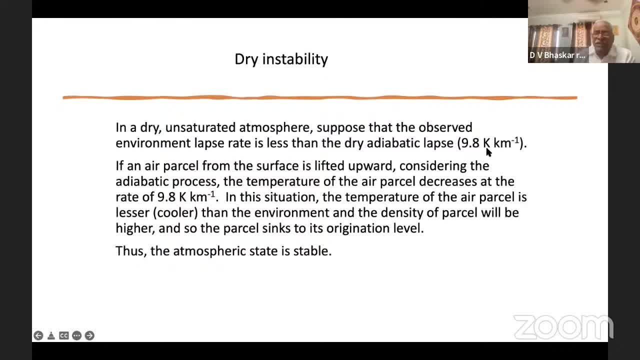 if it is less than the dry adiabatic lapse rate. we know it is 9.8 degrees Kelvin per kilometer And that is the status. And from the surface, for example, if the air parcel is lifted upward and again considering it an adiabatic process. 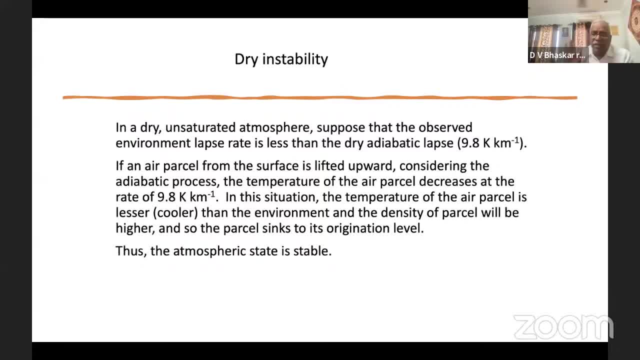 we know that the temperature of the parcel decreases at the dry adiabatic lapse rate, that is, 9.8 degrees Kelvin per kilometer, And in the environment. now we see that the the dry adiabatic lapse rate is less than. 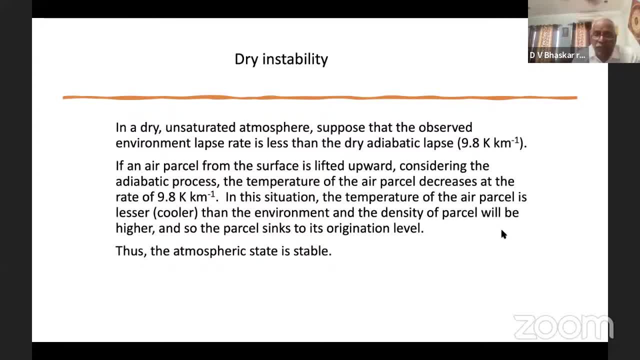 the dry adiabatic lapse rate. So we know that the parcel, as it is being lifted, it will have its temperature within the air parcel decreasing at the rate of the dry adiabatic lapse rate, that is, 9.8.. 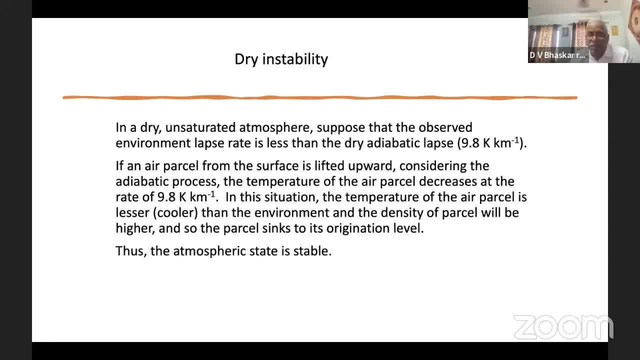 So the environment. the lapse rate, observed environmental lapse rate is less than the dry adiabatic. So less than the dry adiabatic. in which case what happens is the the air parcel temperature is always cooler than the environment. 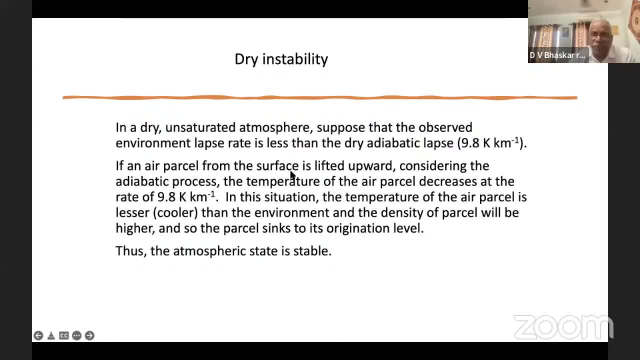 because this is. this is decreasing at a at the rate of 9.8,, whereas the environment, the decrease of the temperature with height is less than 9.8 and the air parcel, in the dry condition it is, the temperature is decreasing at 9.8.. 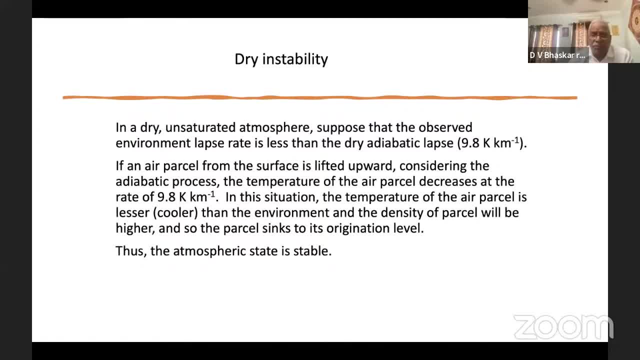 So when it is lifted, what happens is the air parcel is cooler than the environment. So in this situation, the temperature of the air parcel is cooler, is cooler than the environment, And the the you just leave it anywhere, It will go back to its original level. 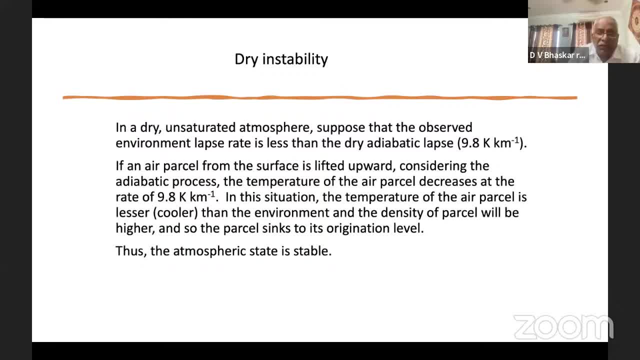 where it finds an equilibrium. that means the temperature between the air parcel and the environmental would agree. So this is the atmospheric state which is called stable. So one one particular type of situation we are seeing. environmental lapse rate is less than the dry adiabatic lapse rate. 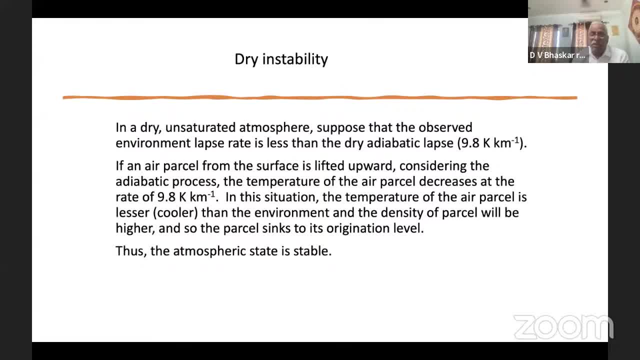 in which case any air parcel lifted from the surface, what happens is it would have the decrease of its temperature at the rate of 9.8,, whereas in the environment the rate of decrease is much less less than the 9.8.. 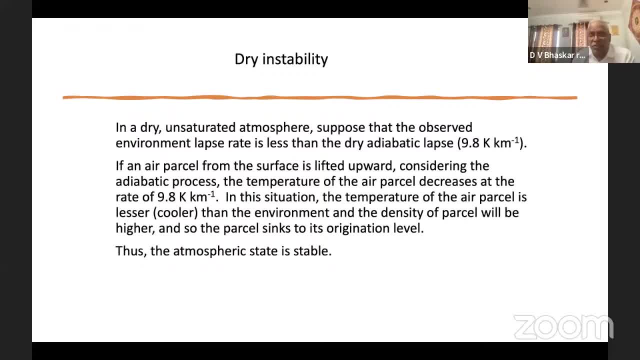 So environment is always warmer and the air parcel is always cooler than environment, And so at any particular time, you don't support the air. but the air parcel is always cooler than environment, And so at any particular time, you don't support the air parcel. 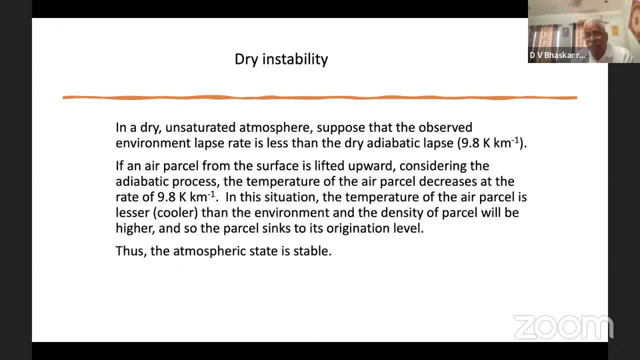 to rise, it will come back to its original position, So to a, to a level where the between the temperature between the parcel and the environmental would coincide. So this is a situation that means the atmospheric atmospheric state is stable. 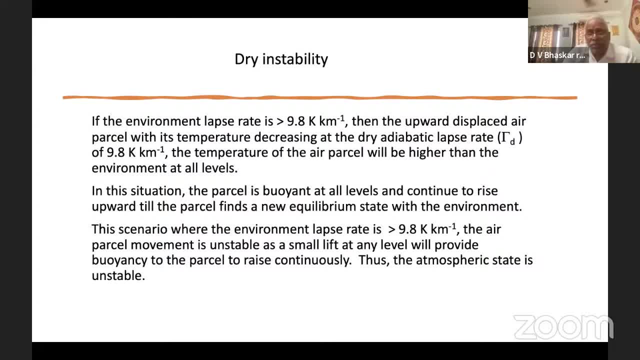 So in the second situation, if the environment lapse rate is greater than 9.8,, then in that situation also the displaced air parcel would have the same. it would have its temperature decreasing only at the adiabatic lapse rate. 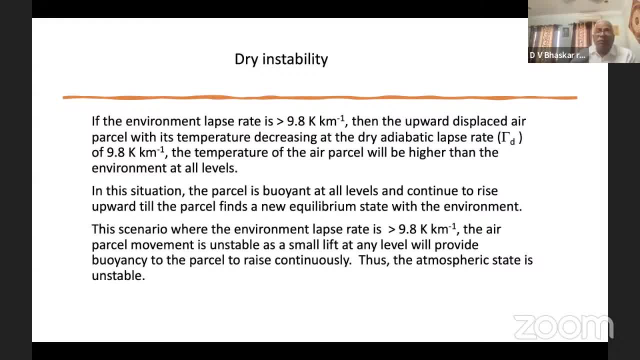 that is 9.8 degrees Kelvin per kilometer, but the corresponding the environmental lapse rate is greater than 9.8. So it is cooling much faster than the parcel. So the environment is always cooler, In this particular case, when the environmental lapse rate is greater than 9.8 degrees Kelvin per kilometer. what happens is because the air parcel would have its temperature decreasing only at the adiabatic lapse rate, that is, 9.8,, which is less than the environmental lapse rate. in that particular condition, the temperature of the air parcel will be higher. 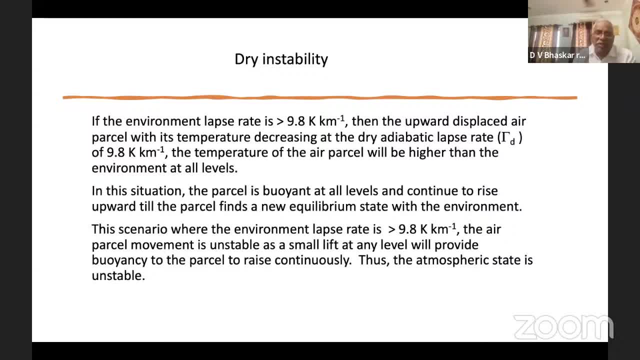 than the environment at all levels. So when, once it is displaced, it will be decreasing only at 9.8,, whereas the environment, the temperature, is decreasing at a rate higher than 9.8.. So environment is always cooler. The temperature of the parcel is always higher than the environment. 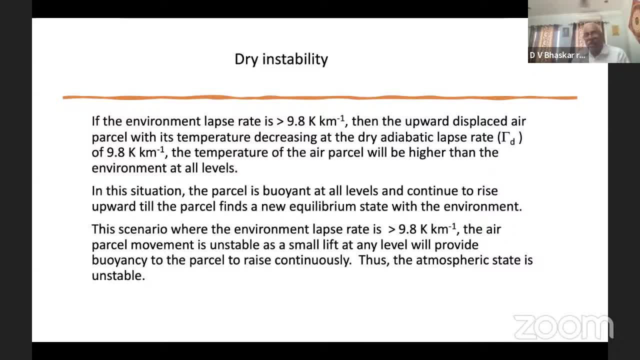 In this particular case, the parcel is thermally buoyant at all levels and it will continue to rise till a level. it will find a new equilibrium state That we will see a little later. but mind you, if the environmental lapse rate is greater. 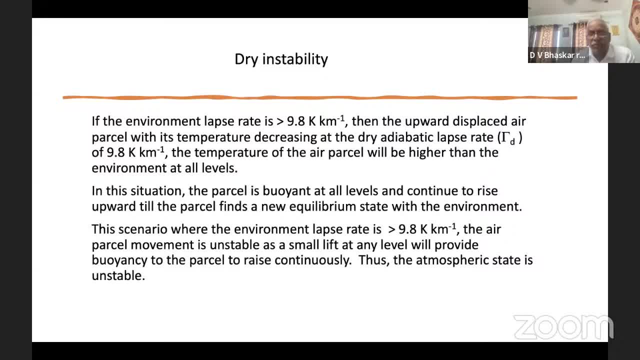 than the adiabatic lapse rate value, 9.8 degrees Kelvin per kilometer, then the air parcel, which will have a lapse rate of 9.8, with its temperature decreasing at that state. the air parcel will always be buoyant. 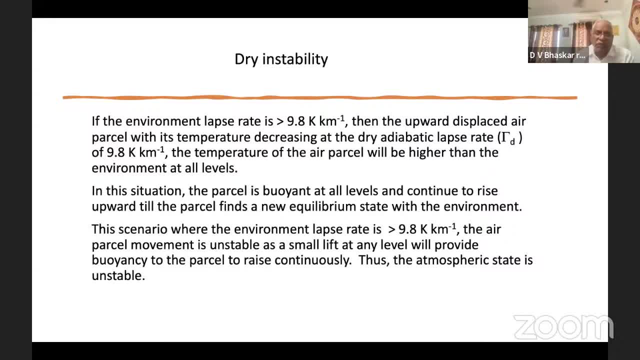 as compared to the environment, And so it will continue to rise. Once it is disturbed, it goes up At any level. the parcel temperature would be higher, So any small lift will make it move further up and up, And so this is a state which we denoted as unstable. 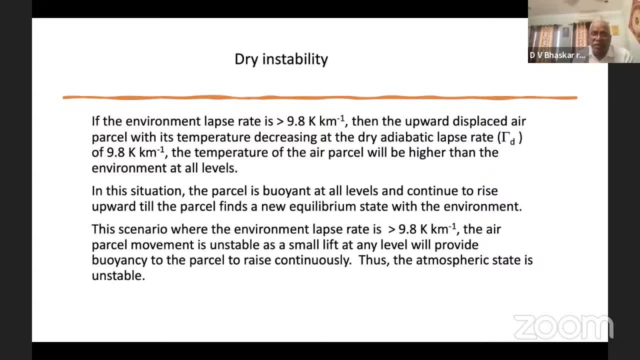 In the previous case, when the environmental lapse rate is less than 9.8,, the dry air parcel would have the temperature decrease only at 9.8,, but so the air parcel temperature will always be cooler, And so it will be. 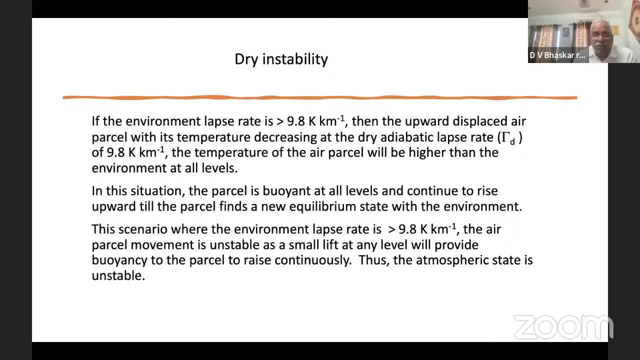 there will not be any buoyancy, And so it will come down to its original level. that is stable, And in the second scenario, where the environmental lapse rate is greater than 9.8 degrees Kelvin per kilometer, the air parcel would, with a small lift, given. 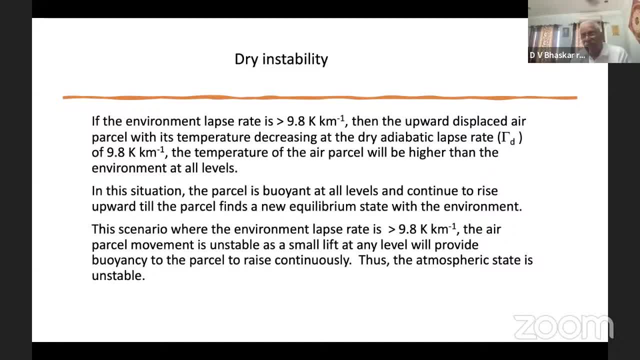 it would start becoming buoyant. that means its temperature will be higher than the environment at all levels, So it will keep on moving. So only a small lift at the beginning, because at the beginning we say that the temperatures of the air parcel and the environment are going to be the same. 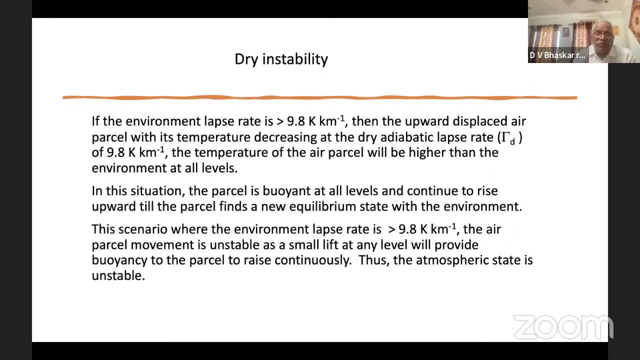 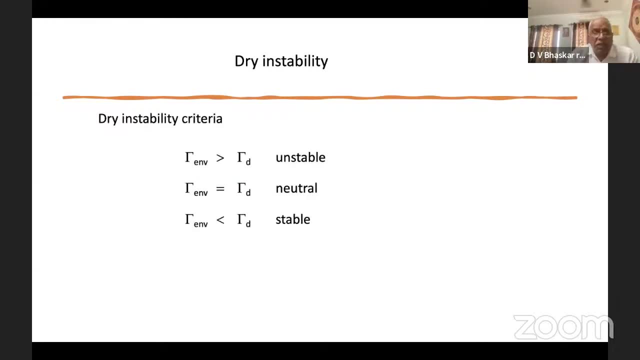 but any small flip to the parcel will make it buoyant and the atmospheric state we call it unstable. So in the dry condition we have seen, with respect to the dry aerobatics, lapse rate which is stable and which is unstable. So writing this criteria, tau, environment means 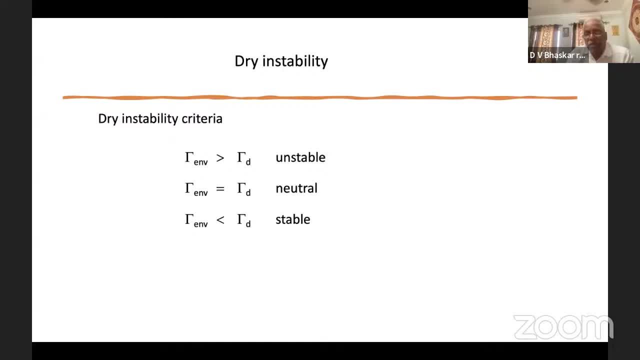 environment lapse rate is greater than the dry adiabatic lapse rate, it is unstable. The tau environment- that means lapse rate of the environment- is equal to tau d, which is neutral. So tau of environment is less than tau d, it is stable. So whatever I discussed, I have put. 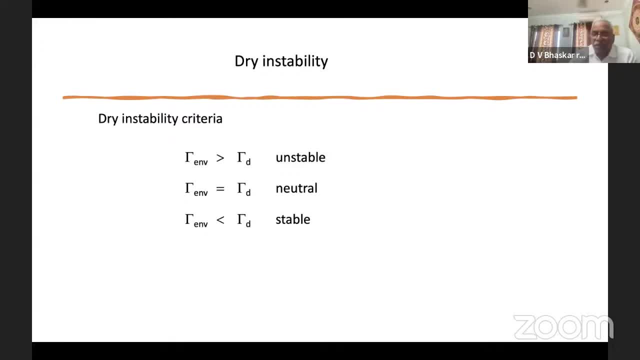 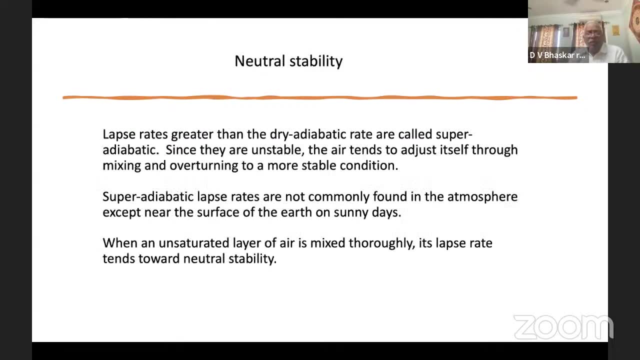 mathematically tau, environment greater than equal to or less, which would correspond to unstable, neutral or stable respectivity. Well, what is the neutral stability which we will see? just For example, there is a dry adiabatic lapse rate, Sometimes the lapse rate 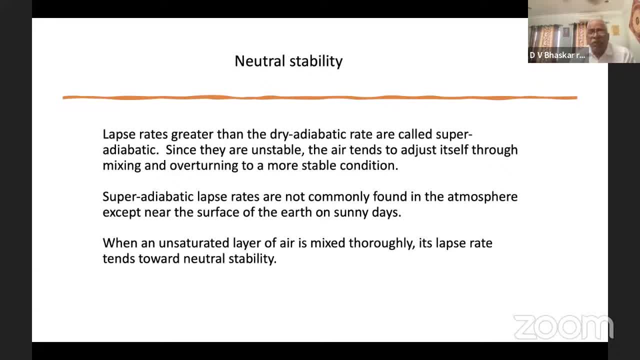 environment lapse rate goes beyond the dry adiabatic, Then it is called a super adiabatic, in which case we know that if the environment lapse rate is greater than dry adiabatic it is unstable. So the air, actually the atmosphere, tends to. 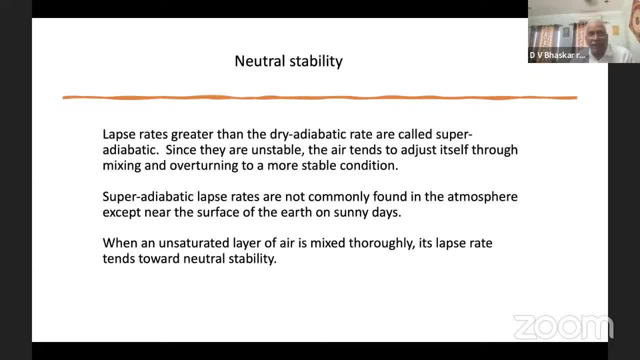 adjust itself through a mixing in that particular layer where it is unstable, And the vertical mixing generally brings it to a stable condition between two levels or in a layer. That means in a layer if the dry adiabatic lapse rate, if the environmental lapse rate goes beyond the 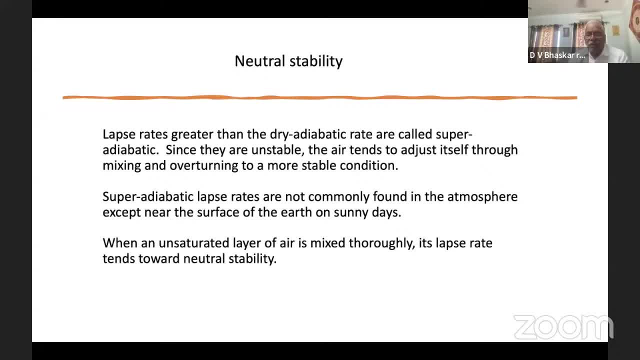 dry adiabatic lapse rate. we call it super adiabatic. then what happens is there will be vertical mixing of the air, leading to a more stable condition. So the atmosphere does not permit the super adiabatic lapse rates to exist for a long time. Super adiabatic lapse rates are. 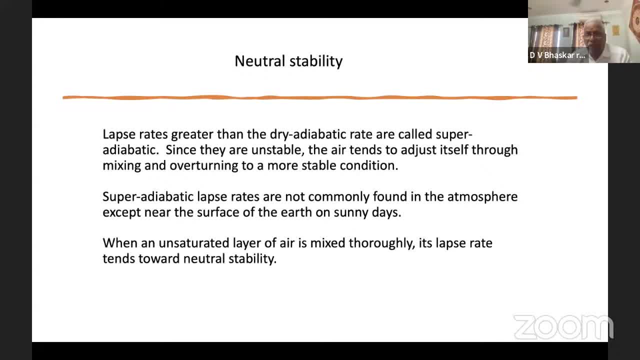 not very common to find, But what happens is the air tends to adjust itself. The atmosphere tends is on a very sunny afternoons when the earth's surface gets heated very fast, because direct heating of the sun at the earth's surface makes it makes the temperature to rise much faster than 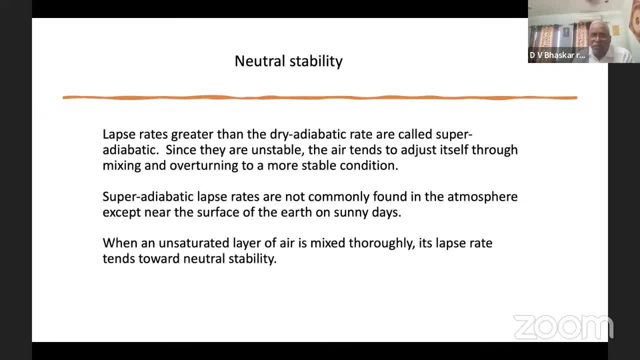 the environment, and so the surface temperature is much larger than the immediate layers above then. what happens is there is a possibility for the environment lapse rate to go beyond the dry aerobatic lapse rate, and in that particular case what happens is in a small layer very near the. 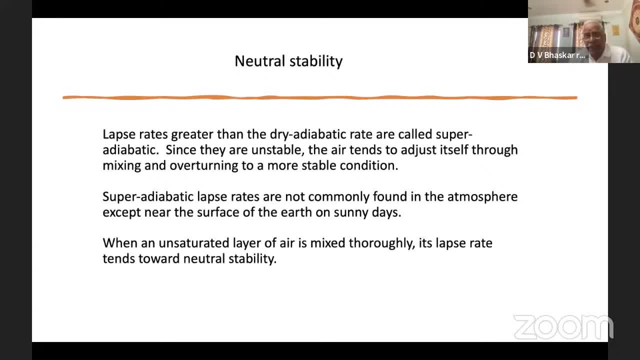 earth's surface there will be a lot of vertical mixing and and that particular kind of condition will lead to a state that means a neutral stability. that means in that small layer where there is a lot of vertical mixing. so the the lapse rate is constant. the lapse rate is neutral, neutral. 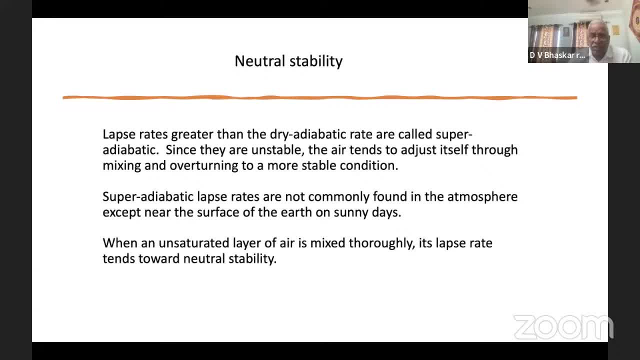 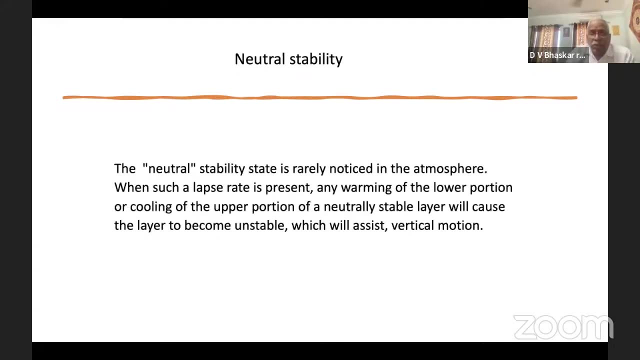 so everywhere it is, the temperature is same, between one level to, between the bottom level to the top of that mixing layer. what happens is: the temperature is same, so you will have neutral stability. so, but when such a neutral, stable state is present, what happens is that, though it is, 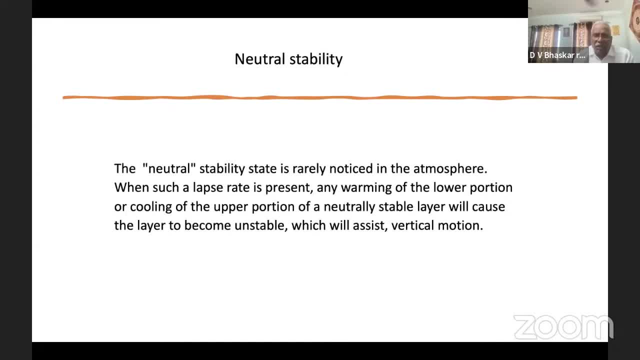 stable, neutrally. neutrally stable that means the temperature everywhere is same. but any smaller disturbance like warming of the lower part and cooling of the- either warming of the lower part or cooling of the upper part- will disturb the neutral step, neutral layer, very easily and the layer will become unstable. so the neutral state, although 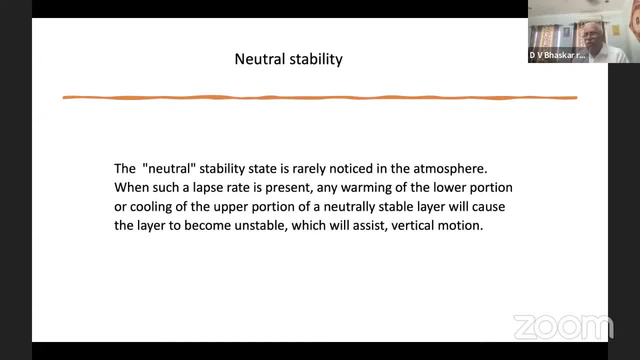 notice for a notice. it will be very for a very short time. so the vertical mixing takes place between two levels in a central layer and the vertical mixing takes place between two levels in a small layer. and even that neutral state would not stay longer because in the atmosphere 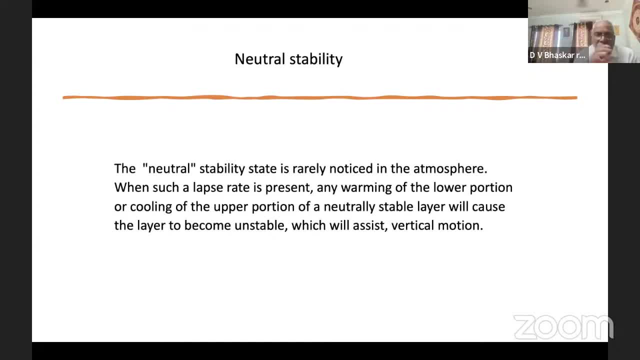 if there is any kind of warming at the lower levels or cooling at the upper levels will make it unstable, or vice versa. if there is a cooling at the lower levels, advection, some particular kind of state which brings in cold air at the lower, or the cooling and warming at the upper levels, then it becomes more stable. so neutral stability is one. 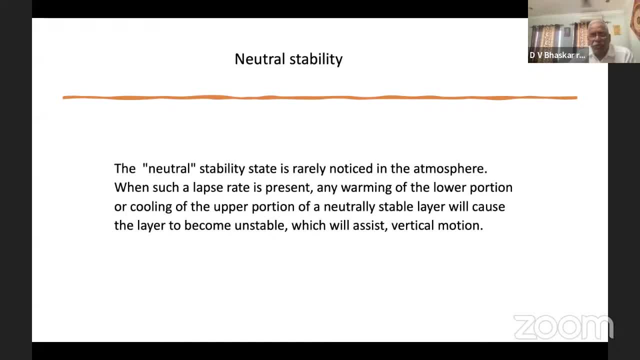 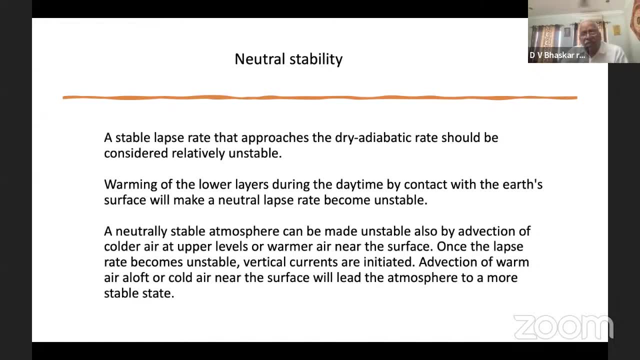 one particular condition which you need to be aware of, but normally very rarely it is observed. so a stable lapse rate that approaches the should be. we know i already explained this- warming of the low layer during the daytime because of the heating at the earth surface will make the neutral, because 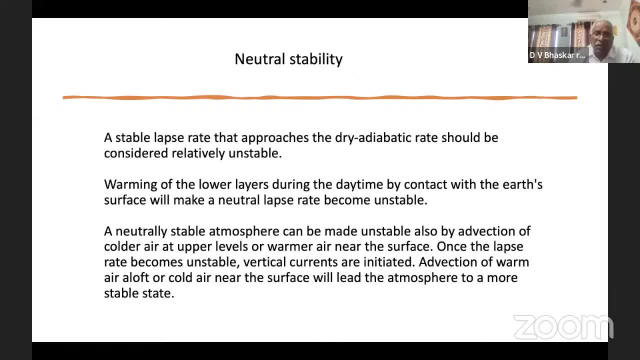 normally, even if you have a neutral state, what what happens is more heating at the surface will make it unstable, or even advection of the cold air at the upper levels or the warm air near the surface also will make it more unstable. okay, that's about a neutral instability. you need to. 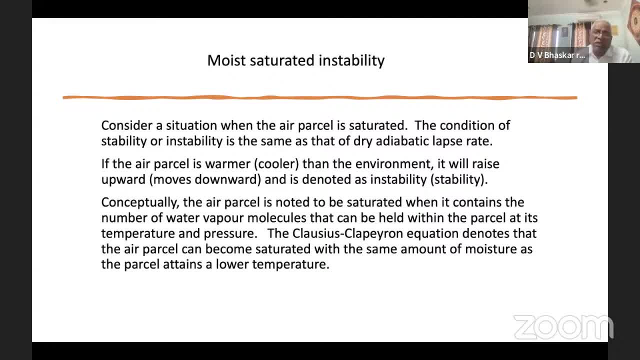 know only a few things: how neutral stability can can occur. and then how. what are its characteristics, how it can be dispersed very easily. so we will consider a moist saturated instability. moist saturated, that means the parcel is moist saturated. okay, so we consider a situation when the air parcel is 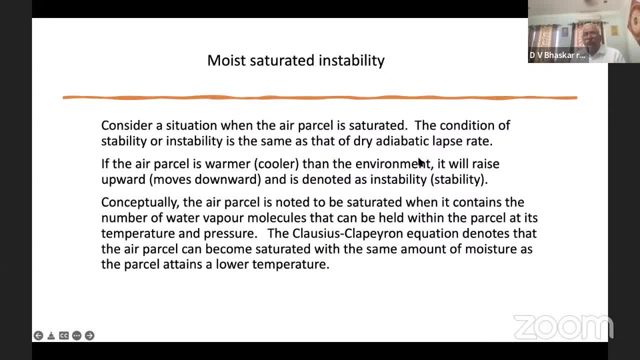 saturated and the conditions for stability or instability of the parcel is the same as the dry adiabatic state. that means if the fall, if the air parcel is warmer than the environment, it will rise upward, or if the air parcel is cooler than the environment, it will go, it will be displaced. 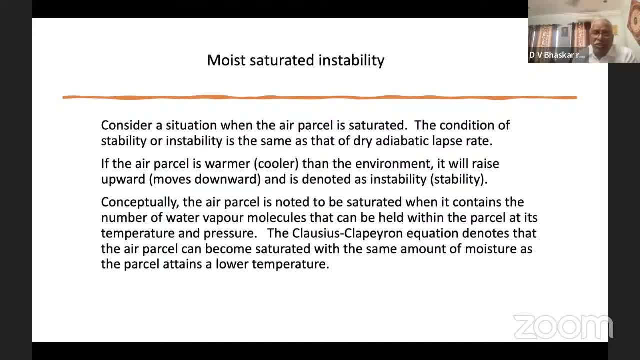 downward, otherwise it will move downward. so if it is warmer than the environment, it is unstable, it is called unstable. if it is coming down because it's cooler than the environment, it is called stable. so the concept of stability and instability is same as of the data bat, but now we'll see how it is. 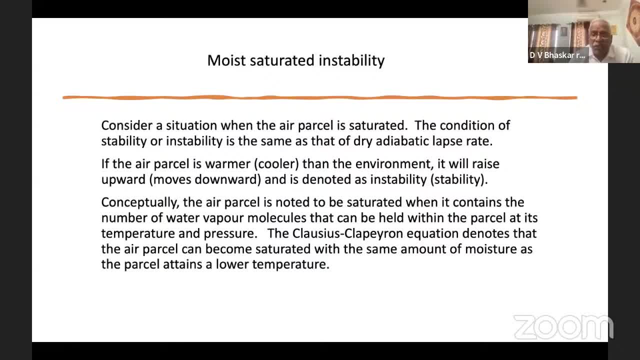 different from the draedabet because now the air parcel is saturated. we know that it can. it contains certain number of water vapor molecules. the condition of saturation means that whatever the number of water vapor molecules present in that air parcel are just enough and at that particular temperature and pressure, and no more water molecules can be added to that. 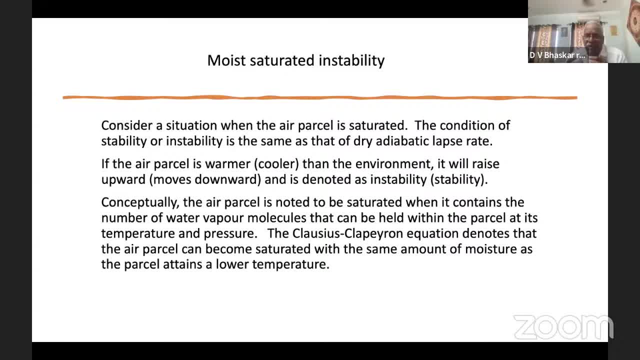 That means it has the because at every, the atmosphere can hold only a certain amount of water vapor, which is related to temperature and pressure, as we have seen with respect to the Clausius-Clapeyron equation. So the Clausius-Clapeyron equation denotes that the air parcel can become saturated with. 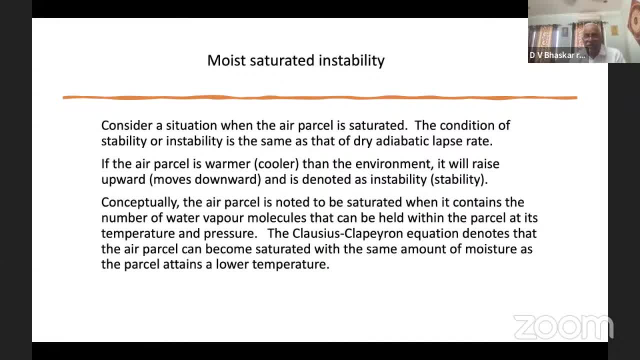 the same amount of moisture as the part of parcel attains a lower atmosphere. So because we know that the saturation is dependent on both the air and the atmosphere, both the temperature and the pressure. but here the pressure is getting adjusted at every level and so it is more dependent on the temperature and the water vapor molecules are same. 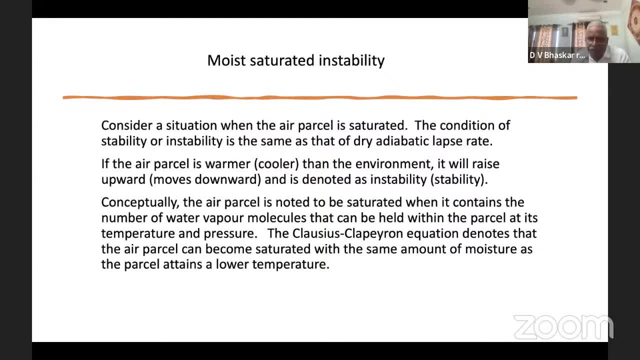 They are not going to be changed. We are not going to add any water vapor molecules into the parcel. but if the same air parcel, when it is lifted upward, as we have seen, the temperature decreases And at such a time the air is not saturated, 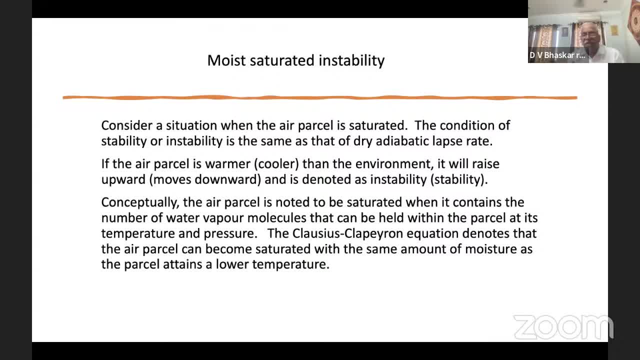 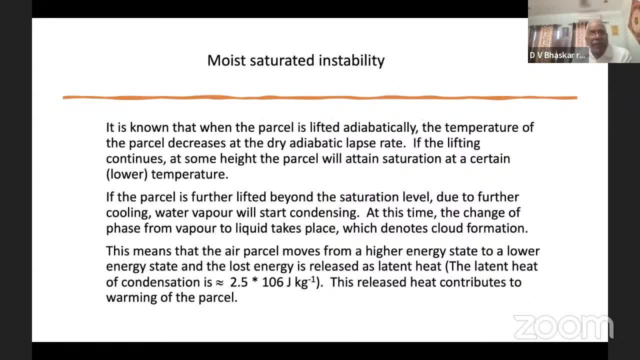 That is the concept we know And when the parcel is lifted adiabatically from the surface, we know that the temperature, because it is not saturated At the surface it is not saturated, So the parcel will decrease at a dry adiabatic lapse rate. 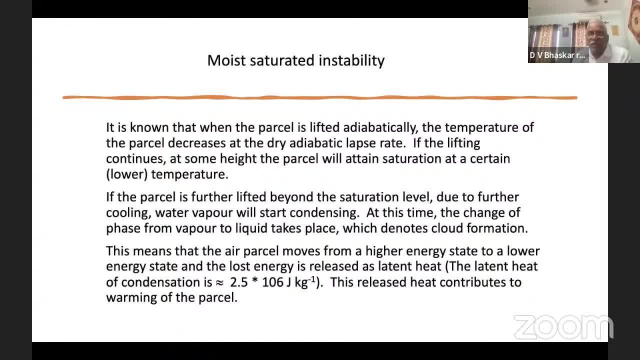 And as long as lifting is given at some particular level, the parcel will attain a temperature that will make the parcel saturated. That means at the surface when you have a parcel it is unsaturated, but it has certain water vapor content inside. but that is not enough for saturation. 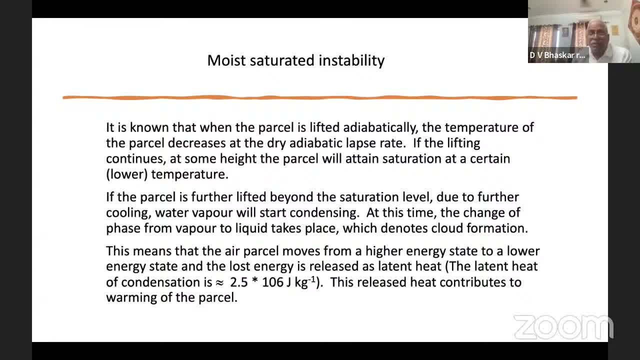 But when the parcel is lifted adiabatically, the temperature of the parcel decreases at the dry adiabatic lapse rate 9.8 degrees Kelvin per kilometer, And as the lifting continues the temperature will be coming down and down. 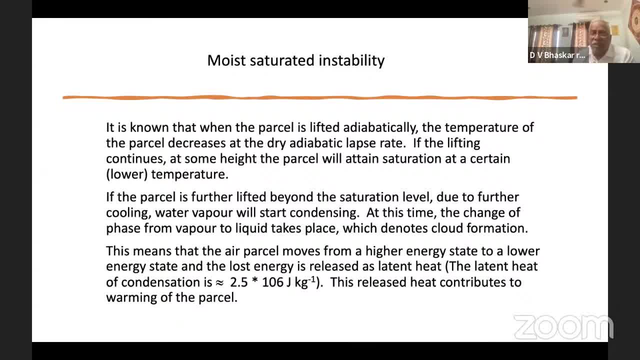 And at some particular temperature value the parcel will attain saturation. That is the important concept you should remember. So at dry adiabatic lapse rate the parcel will attain saturation. The dry parcel, that dry unsaturated parcel, dry unsaturated parcel at the beginning it. 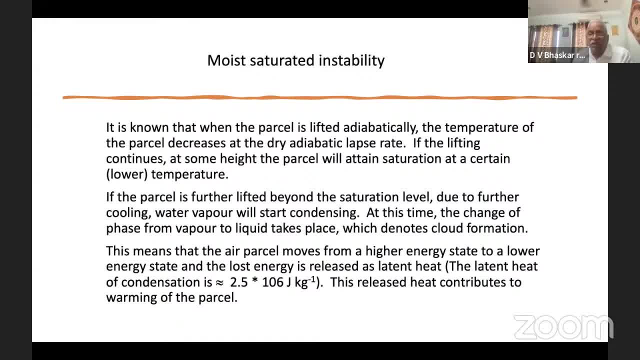 would decrease When lifted adiabatically. its temperature would decrease at the dry adiabatic lapse rate And at some particular level the parcel will attain a certain temperature at which the parcel will be known to be saturated. So, because I said this last one, 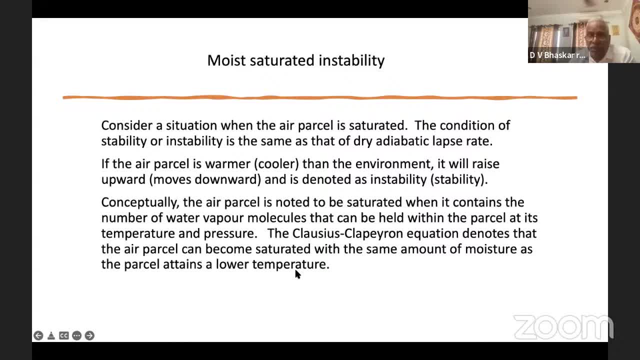 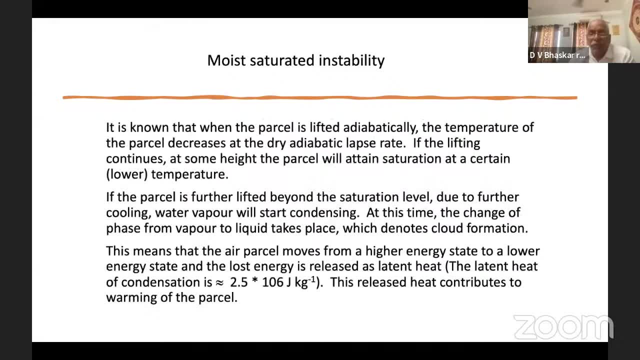 So with the same amount of moisture the parcel attains saturation at a lower temperature. So here at the beginning, when it is unsaturated, dry unsaturated, the parcel will have the decrease of the temperature at dry, adiabatic lapse rate. 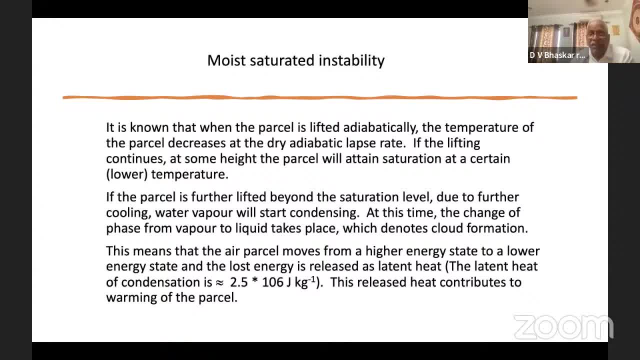 And so at certain temperature the parcel will attain a temperature value which actually corresponds to its saturation. So if you have understood up to this, so at some level, when the parcel is lifted adiabatically, the parcel, because it is dry, unsaturated, it will have the temperature decrease at the 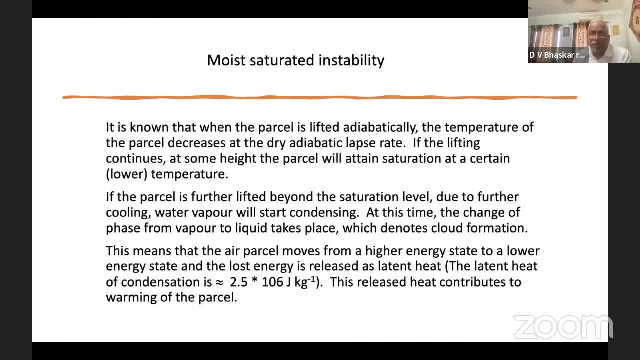 dry adiabatic lapse rate At some level it will have a temperature that will make the parcel completely saturated with the same amount of water vapor molecules. So if the parcel is further lifted above the adiabatic lapse rate, the parcel will attain. 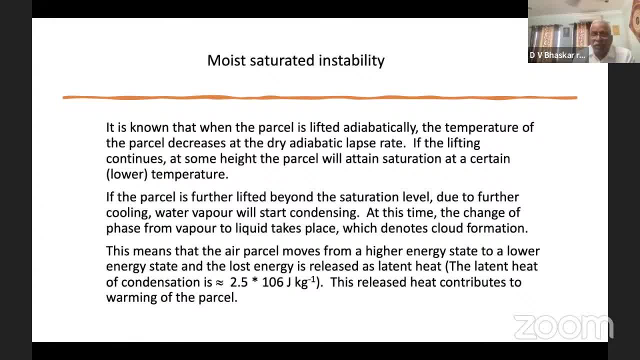 a certain temperature. So about the saturation level? if the parcel is further lifted due to further cooling, water vapor will start condensing. That means, if the temperature falls below the point of condensation, what happens is it's still a lower temperature. 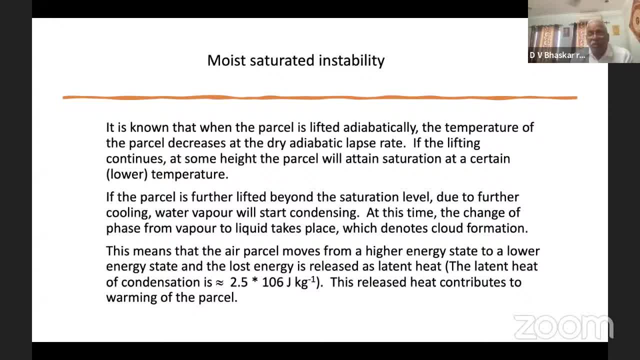 It cannot hold all those water vapor molecules that are present and some amount of water vapor molecules start getting converted into liquid water because the parcel, at that particular temperature where it attained the saturating, if it's further cools, not at the level of the saturation at the. 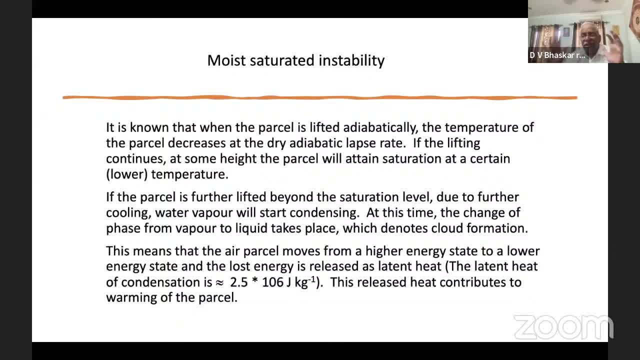 level of the saturation. it is just the temperature and the water vapor molecules are kind of an equilibrium- that it is saturated. but if the parcel is still further lifted, what happens is water vapor will start condensing because at still further lower temperatures the parcel cannot hold all those water vapor molecules present, and so the change of phase. 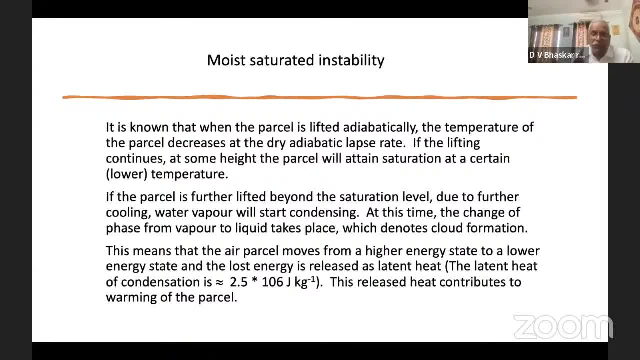 from vapor to liquid takes place and which actually denotes the start of the convection of the cloud formation and, because of the conversion of the water vapor to liquid, that that that means there's a phase change from vapor to liquid, there will be a release of the latent heat. 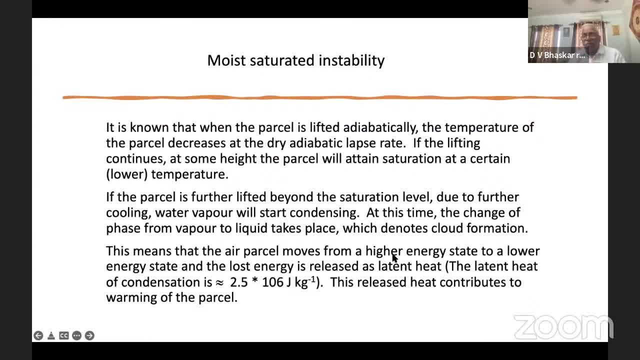 because the parcel is moving or being taken from a high energy state to a lower energy state and the loss of energy is is the latent heat that is released. so which is the latent heat of condensation? you know, 2.5 into 10 to the power of 6? i'm sorry this is not correctly placed here. 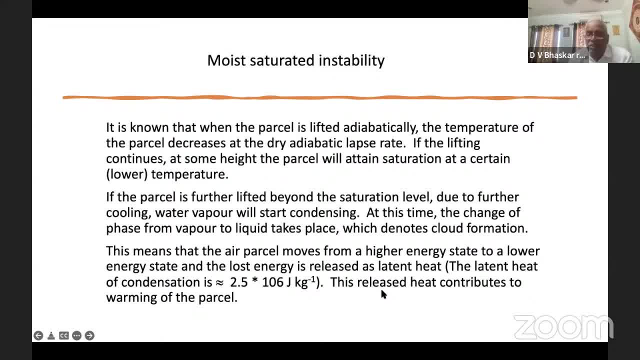 joles per kilogram and this release related this release. the heat contributes to warming of the parcel, this release, so there is a don't worry about this value, that is, i'm sorry about this small error. and so the air parcel, when it is taken upwards, even from its saturation point, where it guards, 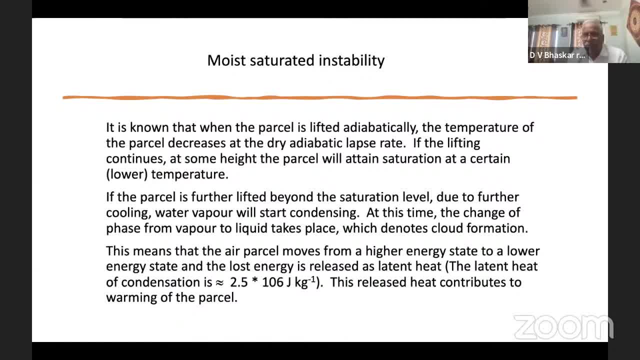 its temperature and and where it got saturated. if it is still made to move upward, what happens is the temperature further decreases and water vapor will start getting converted into liquid water, or condensation takes place And because of that, the latent heat is released. 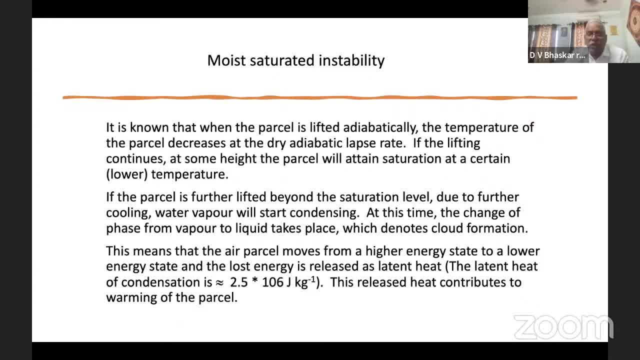 and we know at what latent heat release value is known. So this is very important. This release, the latent heat, contributes to warming of the parcel. Otherwise the parcel will be decreasing at the same rate as before, But because of the latent heat that is released, 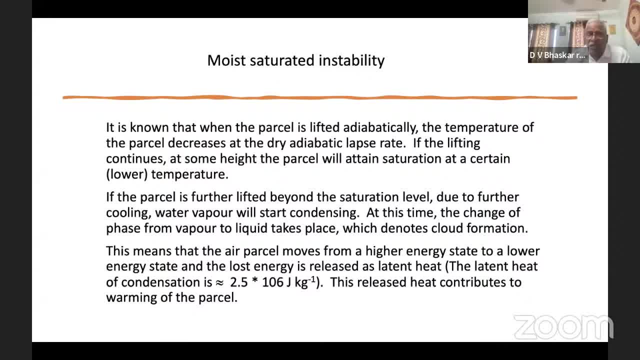 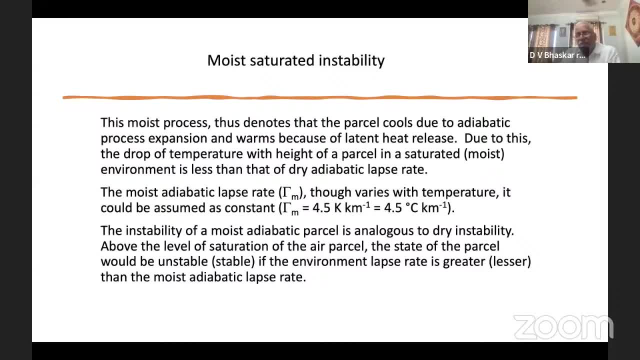 it will contribute to warming of the parcel. So that's the reason why the moist process- when the water vapor started getting. the water vapor started getting changed into liquid water due to the process of condensation. That means then the latent heat is released and this latent heat is used to warm the parcel. 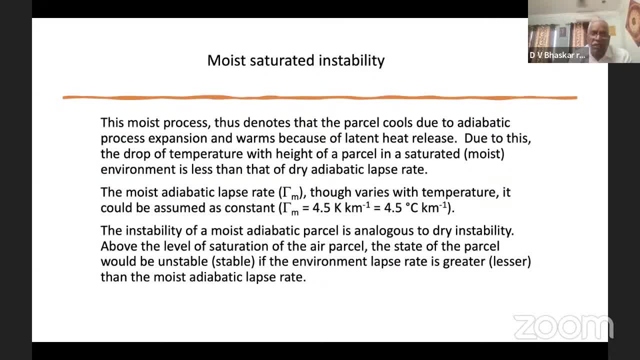 That's why the parcel is warmer, though there is a decrease at some rate. Now, the decrease of the temperature would not be at the same rate because the parcel is getting some additional heat within the air parcel. This is not the exchange of heat between the air parcel and the environment. 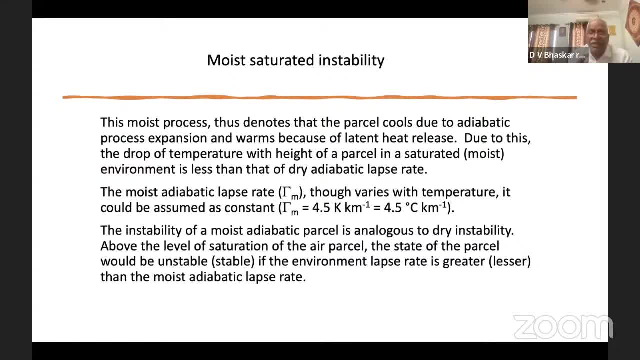 but within the air parcel there is a latent heat release. This latent heat release helps to warm the parcel, And so the drop of temperature with height in a saturated environment is less than the dry adiabatic lapse rate. So if you have understood the concept very clearly, 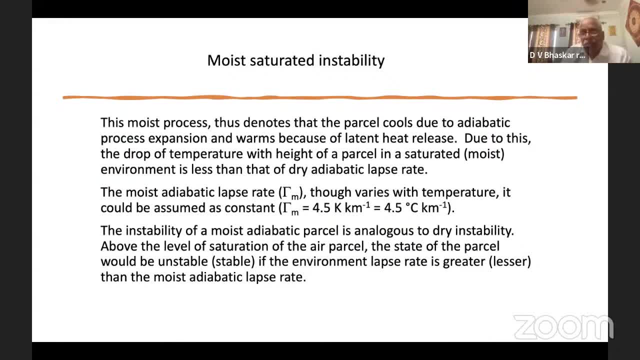 up to the level of saturation. what happens is the parcel is losing it or has it's temperature decreased at the dry adiabatic lapse rate, but above the dry adiabatic lapse rate, what happens is further, that is, if it is a little hot. 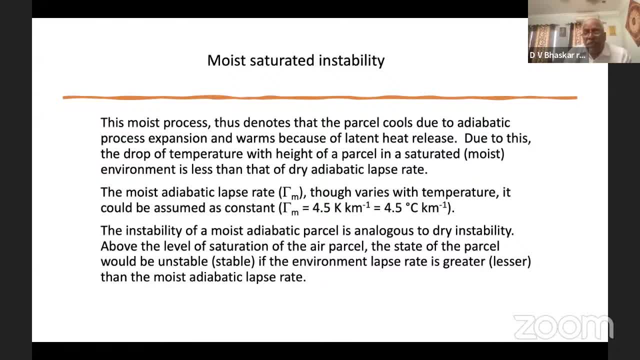 or if there is a decrease in temperature, the dry adiabatic lapse rate, but above the dry adiabatic lapse rate, what happens is further lifting up and then it is decreasing. And so the� lifting it up, the there is a process of condensation, slowly, at lower and lower temperatures, the 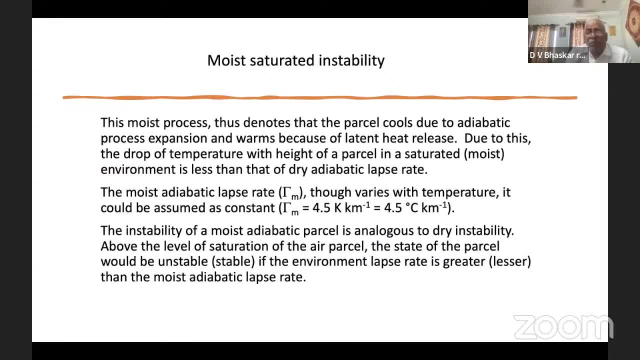 water vapor molecules get converted into liquid water and because of that latent heat is released. that latent heat is used to warm up the air parcel, so the parcel will be warmer than what it would have been otherwise. so so the saturated in a saturated environment, the lapse rate or the 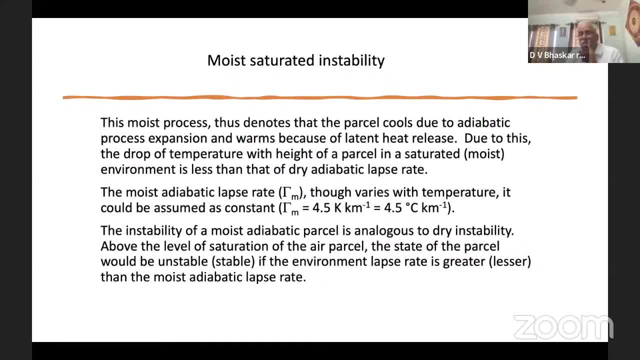 decrease of the temperature is much less than the dry adiabatic lapse rate. this is a very important concept and why the temperature decrease in the saturated environment is less than because of the condensation process. so the moist adiabatic lapse rate, though, varies with temperature. 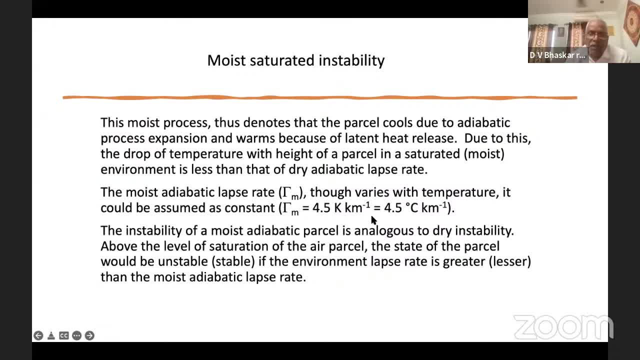 it varies with temperature but it could roughly be have some value like 4.5 degrees kelvin or centigrade per kilometer. so we know that the stability instability of a moist adiabatic parcel is also analogous to the dry instability. so after the saturation, if the air parcel is rising, if the, if the temperature, 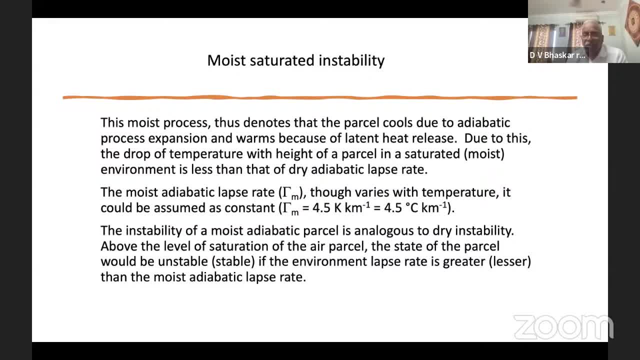 within the air parcel is higher than the environment, then the parcel will have a positive buoyancy, thermal buoyancy- due to rise up. otherwise it will not rise and so it will sink back. so again, it is a difference of the temperature within the air parcel and the environment at different levels that would matter, so the environmental lapse rate. 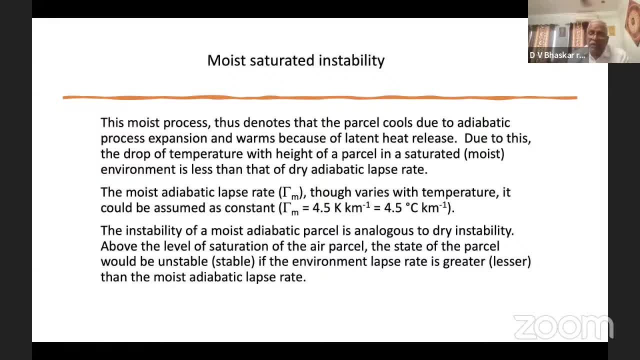 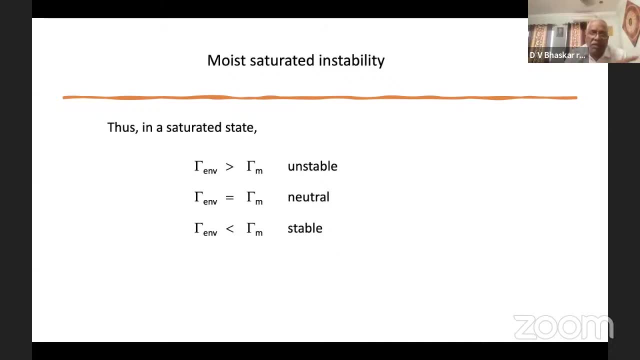 also is not constant. so although i said in the beginning it is greater than or something, we will see the different conditions. so in a saturated state we can very easily say same thing. environment lapse rate is greater than the moist adiabatic lapse rate. it is unstable, it is equal, it is. 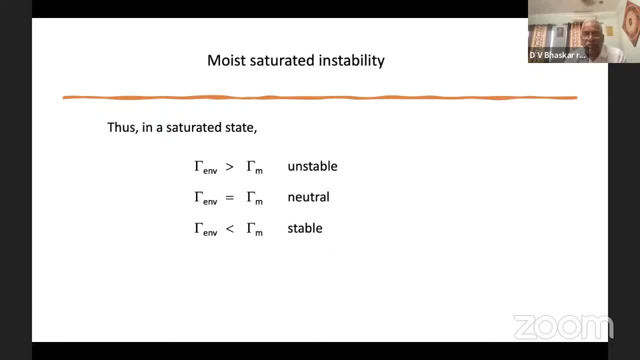 neutral. if the environment lapse rate is less than the tau l, it is stable. so we see that the same particular conditions as of the dry adiabatic condition holds good here also. so if, if, if, if, if. toy. if the saturated adiabatic lapse rate is greater than the environment, that means at 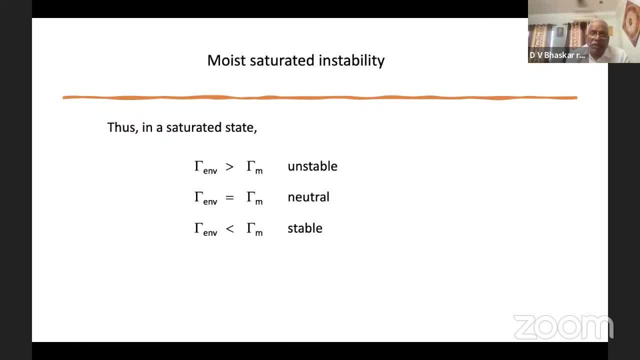 different levels between the level of saturation and above, then the parcel is cooler than the environment and so it's stable, and if the environment has a larger value than the moisture debate, then the parcel will be unstable. so it is easy to understand. so we, i will. i will explain you further. so we, i have explained to you the dry, unsaturated. 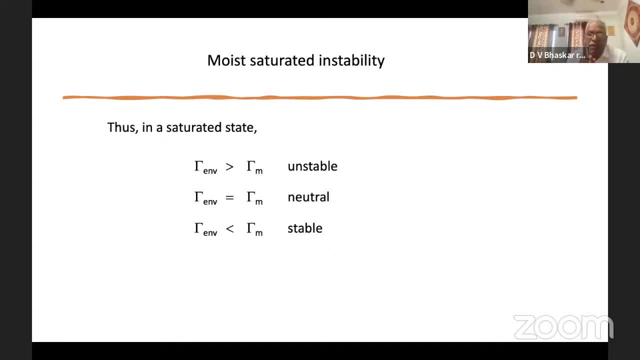 atmosphere, under what conditions, what we should do. and the lapse rate of the air parcel should be compared with the environmental lapse rate. if the environmental lapse rate is greater than the dry adiabatic lapse rate, then it is a dry parcel is unstable, and if the environmental lapse rate is, 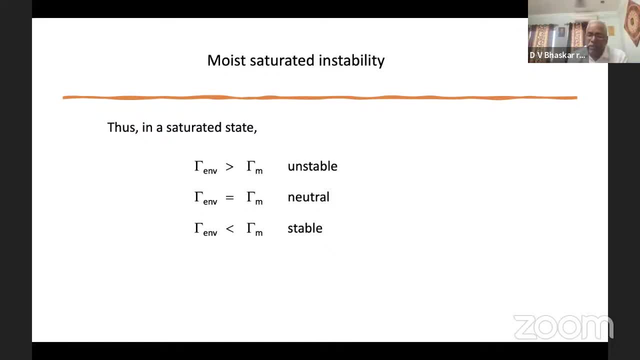 less than the dryed about a clap thread stable. similar is the case even when the air parcel is moist, saturated. then if the environment lapse rate is greater than the moisture debate collapse rate, it is still unstable. the parcel would be, and if the environmental absolute is less than the moisture at the particulars rate, it would be stable. 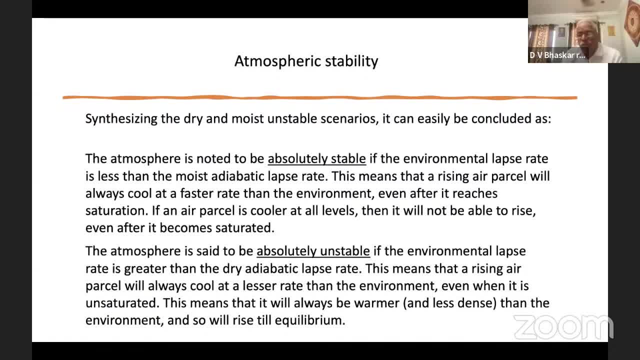 so, uh, so now after, if you have understood the scenarios of the dry, dry, stable and unstable scenario, and also the moist, unstable scenario, these two scenarios, if you have understood, now we can say or make some deduction: The atmosphere is noted to be absolutely stable. absolutely stable if the environmental lapse rate is less than. 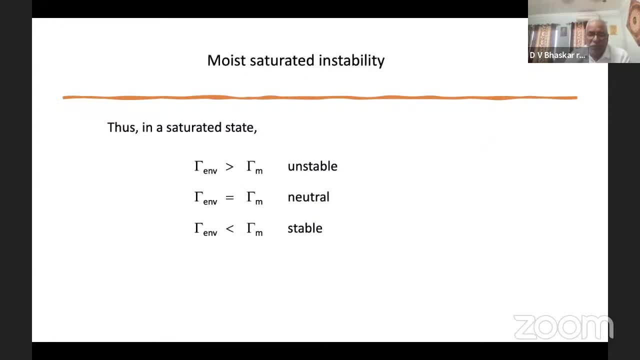 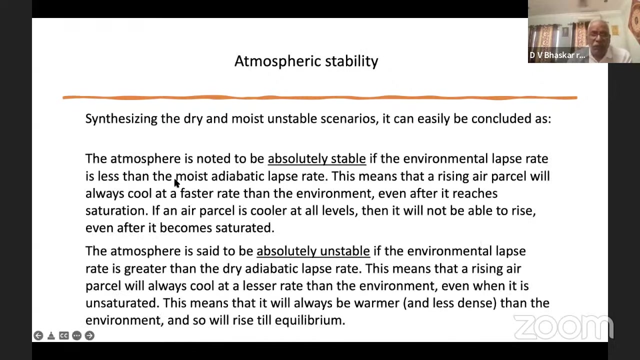 the moist adiabatic lapse rate, Because if the environment is less than the moist adiabatic lapse rate, as I said, the moist adiabatic lapse rate is less than the dry adiabatic lapse rate. So it obviously means the environment is less than the moist as well as the dry. 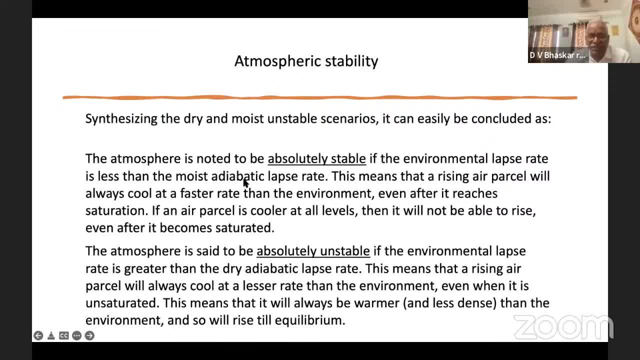 In which case, if the environmental lapse rate is less than the moist adiabatic lapse rate, then the moist adiabatic lapse rate is less than the dry adiabatic lapse rate. So it obviously means the environment is less than the moist adiabatic lapse rate. 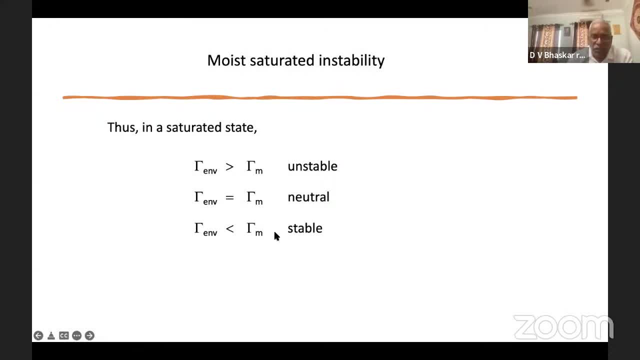 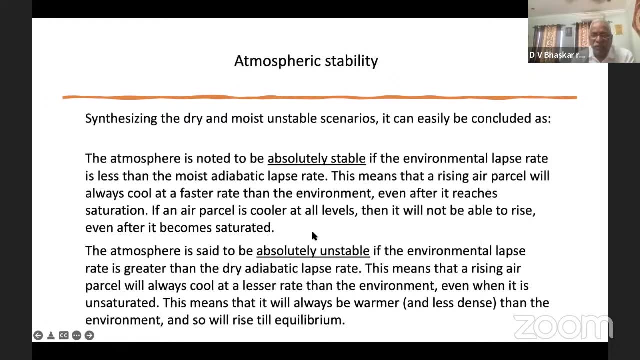 It is stable. So here also, if you write if it is less than tau m, it also means that it is less than tau d, and so it is absolutely stable. That means that that means an air parcel. when it is subjected to upward motion, it will always cool at a faster rate than 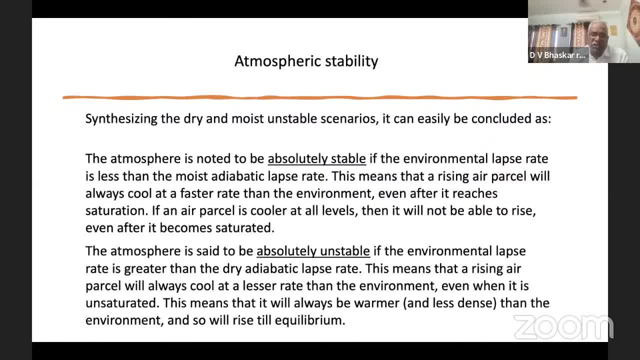 the environment. Even if you force it upwards, it reaches saturation at some level and still, even if you push it upwards, it will always cool at a faster rate than the environment. Even if you push it upwards, it will not be warmer than the environment, and so it is. 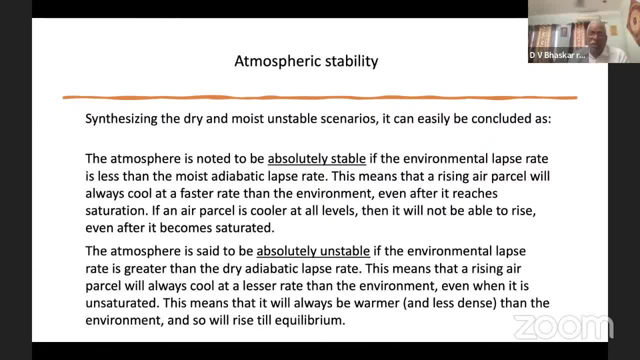 always has no thermal buoyancy, and so it is absolutely stable. That means it will come back to its original position at any particular time If the, if the, if the environmental lapse rate is less than the moist adiabatic lapse rate. it should be known that the atmosphere 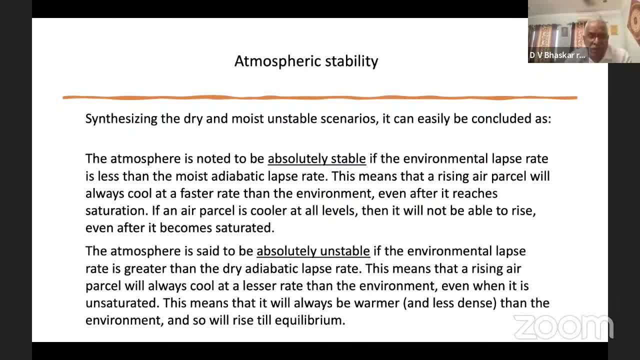 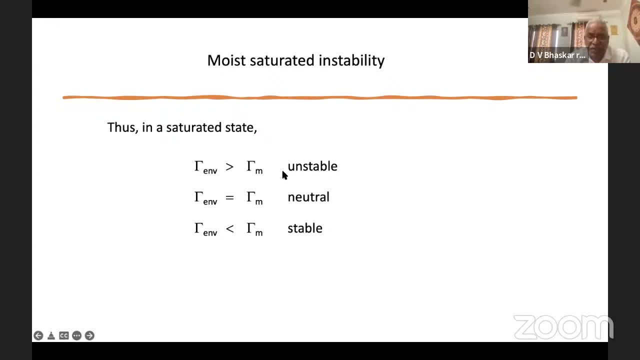 is absolutely stable. Similarly, or analogously, the atmosphere is said to be absolutely stable If the if the environment lapse rate is greater than the multiple adiabatic lapse rate. So we know it is the tau environment is greater than unstable, but tau m is less. 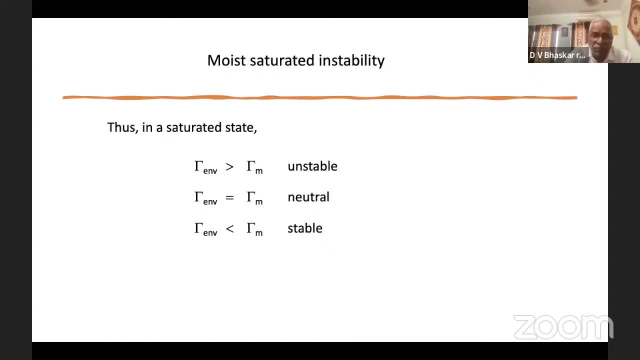 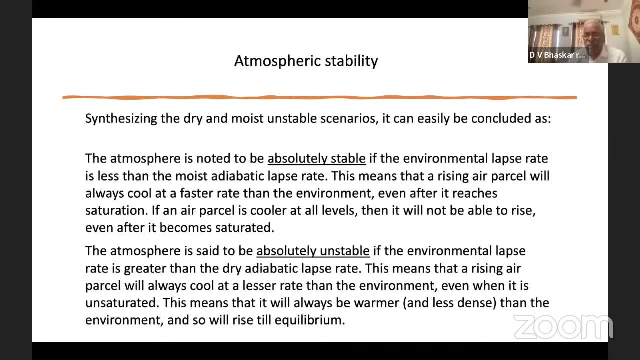 than the tau d, and so if the environment lapse rate is greater than the tau d, it obviously means it is also greater than tau m or the moist adiabatic lapse rate, in which case it is absolutely unstable. That means if the, if the environment lapse rate is greater than. 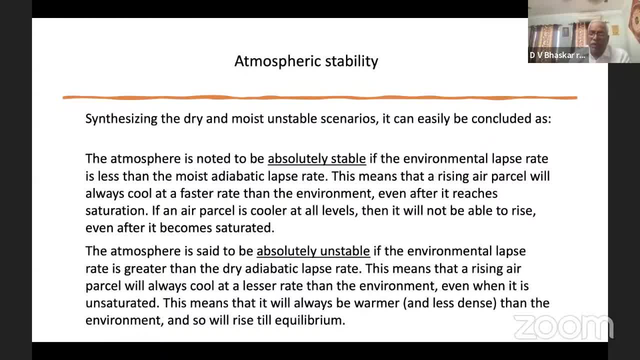 the graduate ar WO D al тут. reconciliation letter. if the environment lapse rate is greater rate immediately as you give a small lift to the parcel at the surface it will definitely go up and everywhere it is always be warmer than the environment, even after getting the a parcel get. 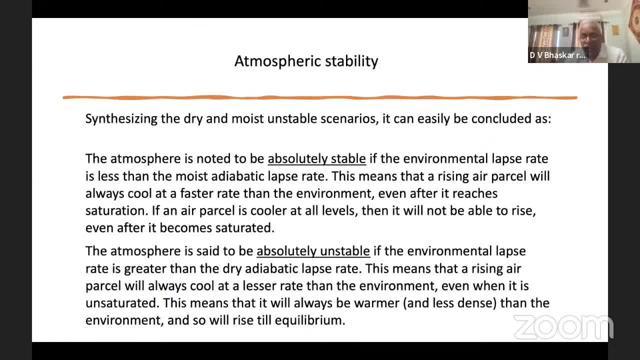 saturated, it is still be warmer at every time. so there is, there are two conditions: the atmosphere is in order to be absolutely stable if the environmental lapse rate is less than the moisture adiabatic lapse rate, and it is absolutely unstable if the environmental lapse rate is. 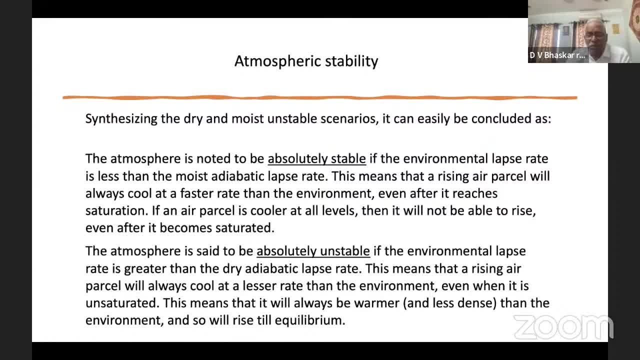 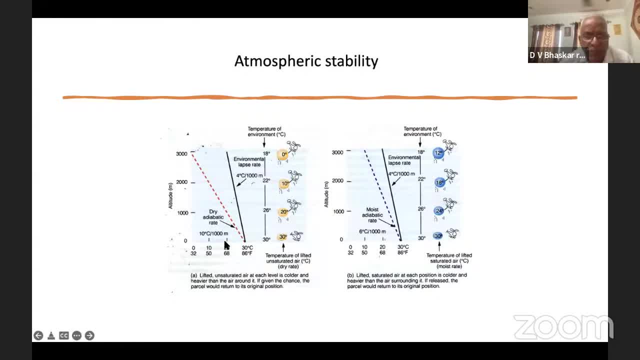 greater than the dry adiabatic lapse rate. so these two can be understood, understood very easily. so here we. we see that in this picture. this is the environmental lapse rate. the solid line, the red dash line, is dry adiabatic lapse rate. it is the environmental lapse rate is. 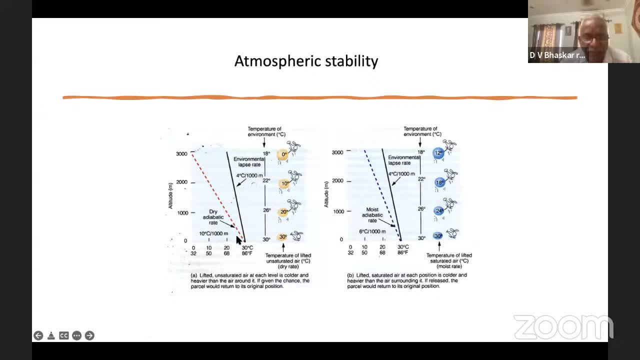 decreasing at four degrees centigrade per kilometer. drive adiabatic is 10 degrees centigrade per kilometer, so this is always cooler than this. so it is always stable here, here and here. the moist adiabatic lapse rate. it is four degrees centigrade environment, but even if the parcel is saturated, it will. 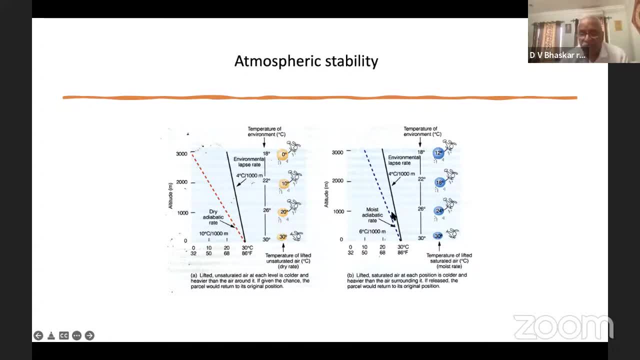 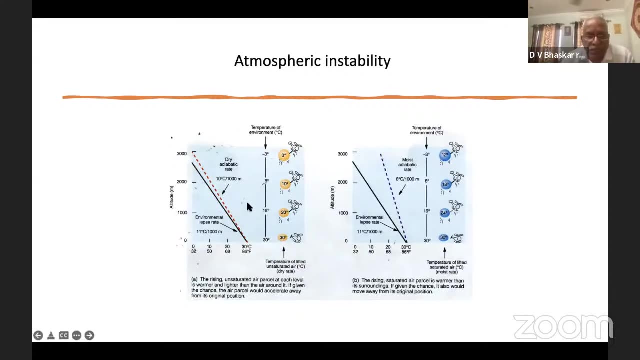 have a decrease at six degrees centigrade per kilometer. even in this particular case, this part, this parcel, will be cooler than environment, so it is absolutely stable. Similarly, if we see the instability, environmental lapse rate is 11 degrees centigrade. 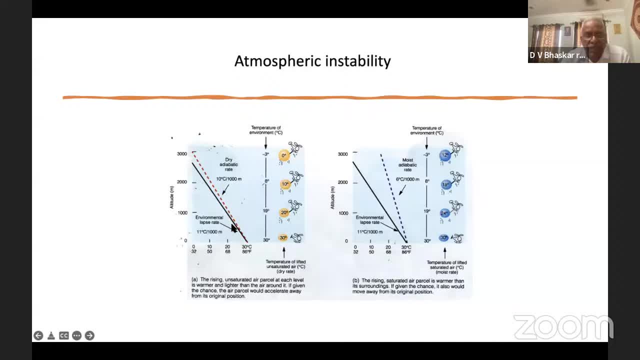 That means higher than the dry adiabatic lapse rate. So the parcel would be having a decrease of its temperature at 10 degrees centigrade per kilometer. So when it is, immediately it will be warmer than the environment and it will be rising continuously. 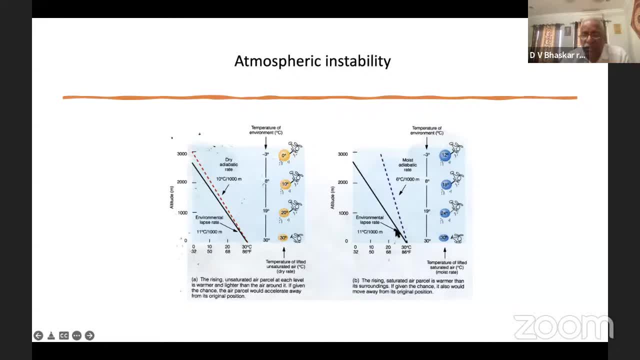 And similarly environmental lapse rate is 11 degrees centigrade and the moist adiabatic lapse rate is six degrees, So this will be cooling at a lesser rate than the environment, So saturated. also, it is warmer than the environment, So it is absolutely unstable. 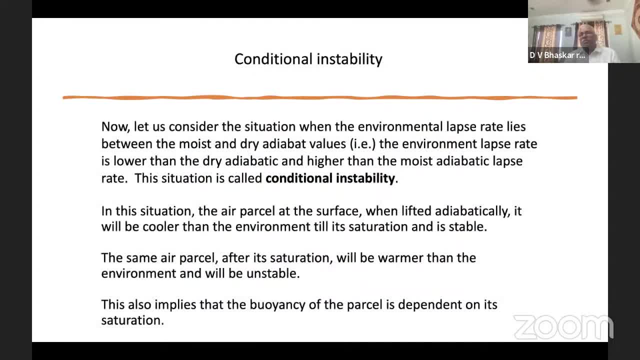 So between these two we have another important concept, because the atmosphere, if it is absolutely stable, we don't need to worry, And if it is absolutely unstable, immediately it will. something will happen to make it more neutral And normally the environment is known. 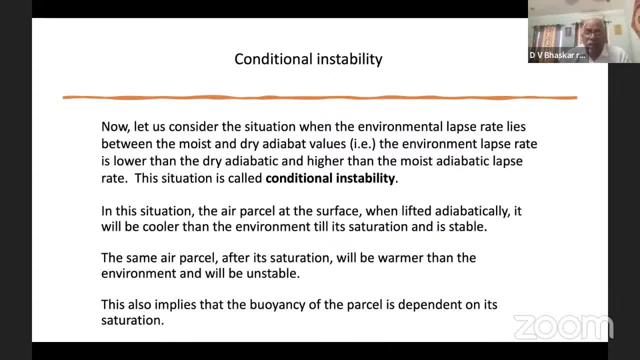 to be conditionally unstable. That means we now see a situation where the environmental lapse rate lies between the moist adiabatic and the dry adiabatic values. That means the environmental lapse rate lies between the moist and dry adiabatic. 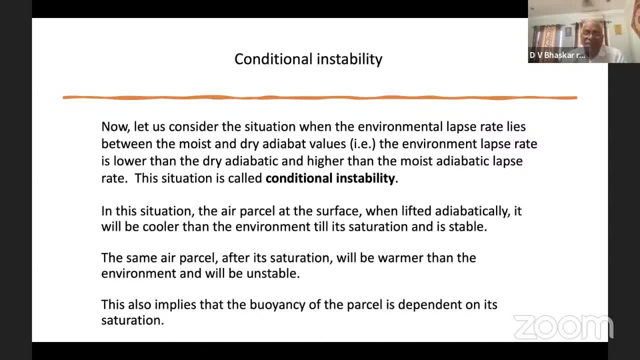 That means it is higher than the moist adiabatic lapse rate but less than the dry adiabatic. So if the environmental lapse rate is less than the dry adiabatic, but it is higher than the moist adiabatic, 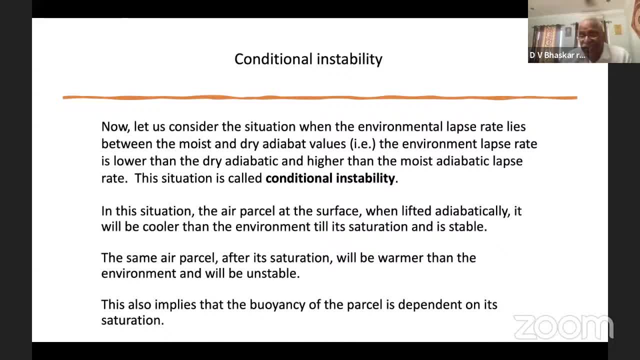 then we have a situation called conditional instability. This is a very important concept in meteorology in the tropical weather. Most of the tropical atmosphere is conditionally unstable most of the times. So this is a situation we experienced day in and day out when we have the radius on the sensor. 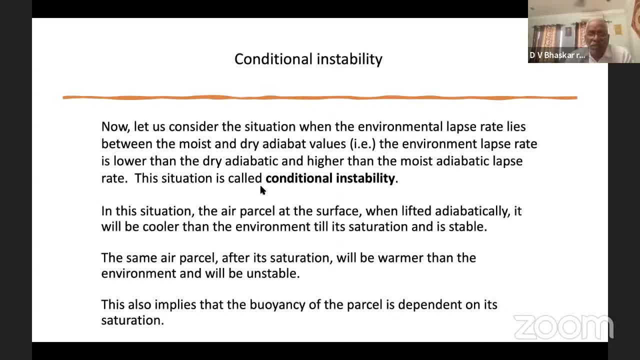 give us the environmental temperature profiles, we see that the environmental lapse rate is mostly less than the dry adiabatic but higher than the moist adiabatic lapse rate. Otherwise, even if it is greater than the dry adiabatic, 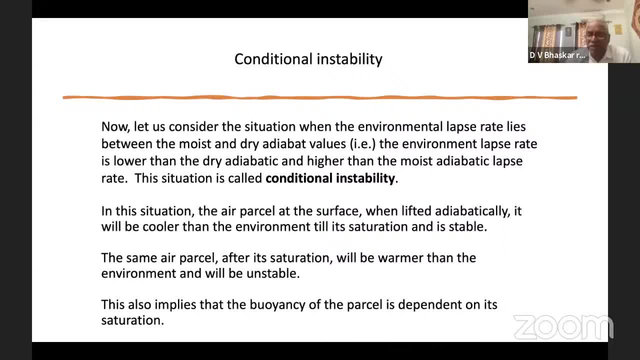 the environmental lapse rate is less than the moist adiabatic lapse rate. it's always higher, So if the temperature is unstable or stable, we don't need to worry. but conditional instability is a very important condition we need to understand In this situation, for example. 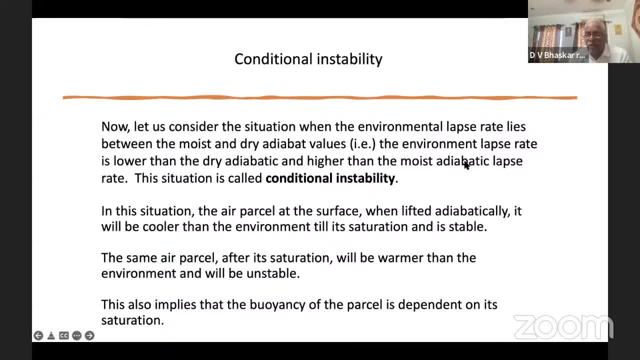 we have an environmental curve temperature profile where the environmental lapse rate is less than the dry adiabatic but higher than the moist adiabatic, then what happens is if we have the air parcel at the surface, same as before, same, considering the same. 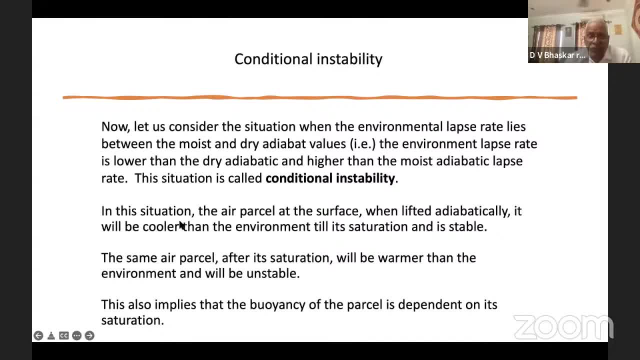 but in this situation, as before, if it is lifted adiabatically, it will be cooler than the environment. till saturation is till it's saturation. That means the parcel will have the temperature decreasing at the dry adiabatic lapse rate. 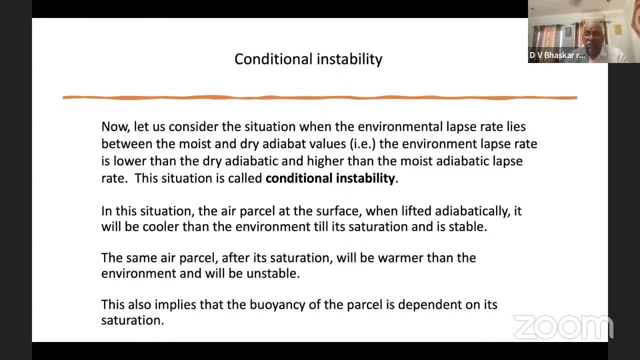 whereas the environmental lapse rate is lower than the dry adiabatic. So the parcel will always be cooler than the environmental value, and up to saturation. So up to saturation we say: see that it is stable, we see that it is stable till it is saturated, till it attains. 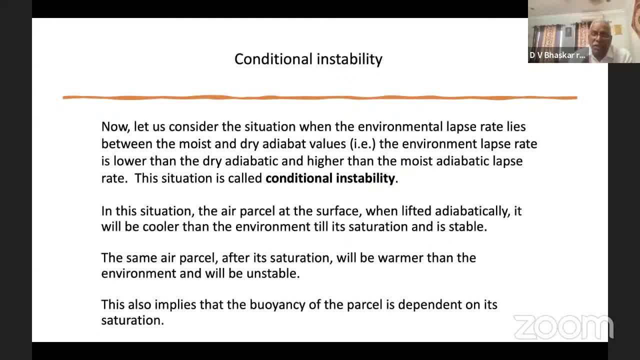 saturation. why? because the parcel is having its decrease of temperature at the dry adiabatic lapse rate, whereas the environmental lapse rate is lower than the dry adiabatic lapse rate. so it's the environment is always warmer, but when the parcel, the same parcel, when it. 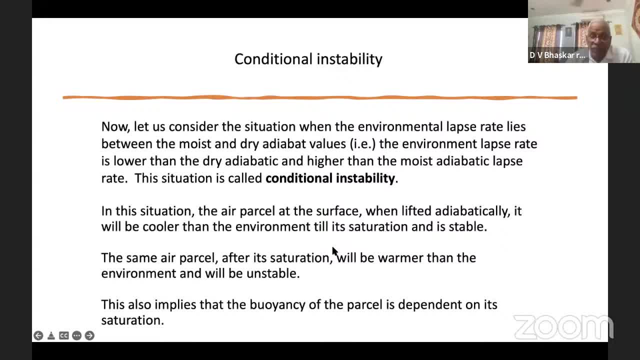 attains the saturation. what should happen when it becomes saturation? we have seen the condition before moist adiabatic instability or instability. what happens is the same parcel. after its saturation it will have its temperature decreasing at the saturated adiabatic lapse rate. so we see that the environmental lapse rate is higher than the moist adiabatic lapse rate. 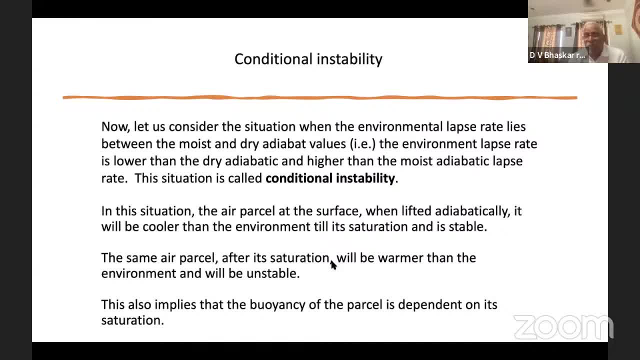 so above the saturation level. what happens is the parcel will be decreasing at the saturated adiabatic value, but the environment will be will be cooling. that means it is having a lapse rate higher than the moist adiabatic lapse rate. so what happens is the atmosphere is environment is cooler than the parcel above the level where the 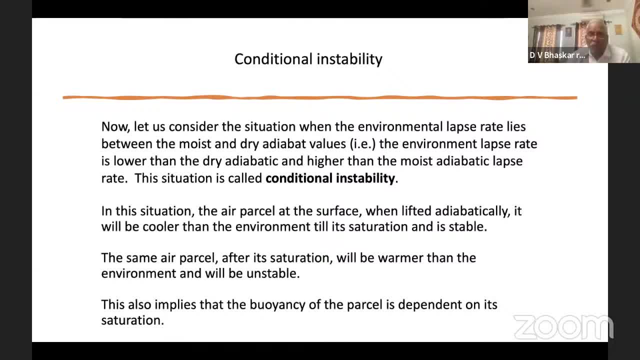 parcel got its saturation. so the same parcel after it gets saturation, because from then saturation it will have its temperature decreasing at the saturated adiabatic value from that particular point onwards, not at that, we will see, it will be warmer than the environment and will be unstable. this also means that the buoyancy of the parcel is very important. 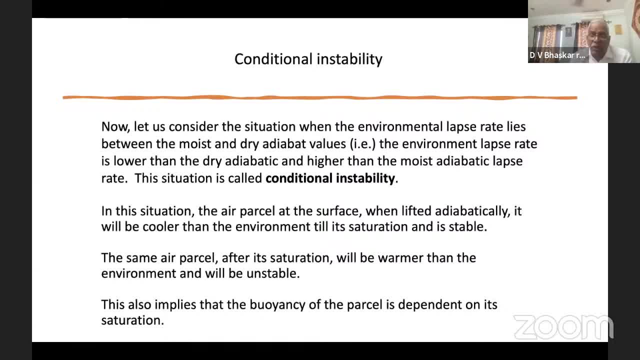 now, under these conditions, on its saturation. so now we see that the same parcel, before it attains saturation, it is, it is stable, but one once it's one. once it attains saturation it is noted to be unstable. so here the stability or instability of the parcel is very much dependent. 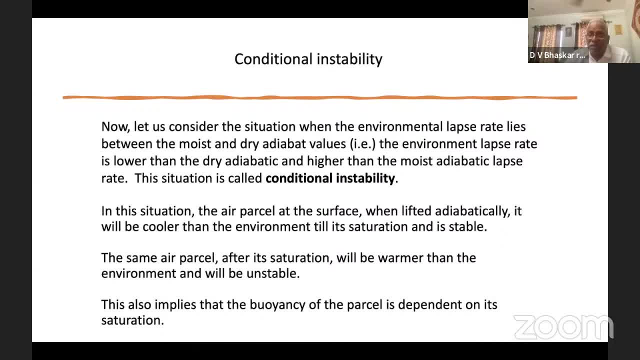 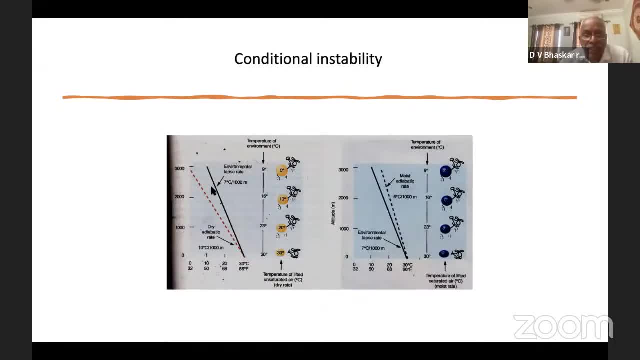 on its saturation in a conditionally unstable environment. so here, so here we see. the environmental lapse rate is seven degrees. so dry adiabatic condition: it decreases at 10 degrees centigrade, so it is always cooler than this but one once. it decreases at 10 degrees centigrade, so it is always cooler than this but one once it is. 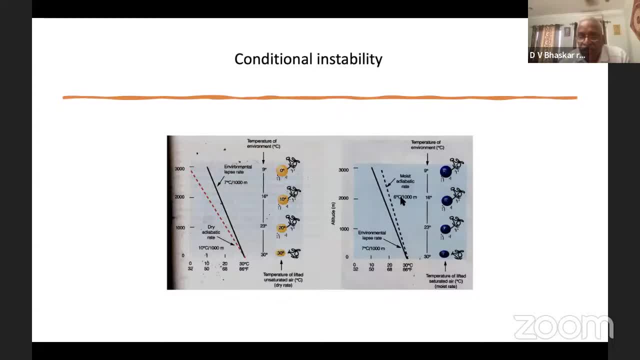 it decreases at 10 degrees centigrade, so it is always cooler than this, but one once it is. attains saturation. uh, the saturated adiabatic lapse rate is six degrees if we imagine environmental lapse rate is seven degrees. so moist adiabatic, the air parcel is always warmer. 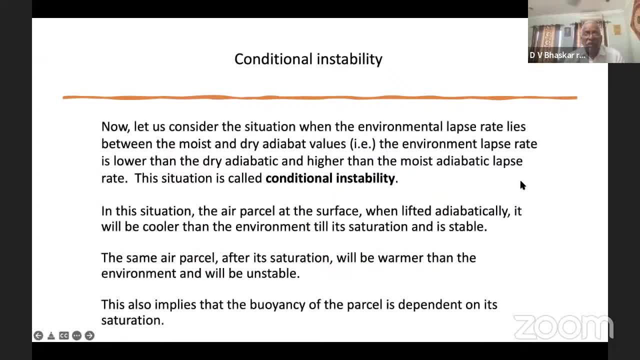 so conditional instability is very much uh is a very important uh situation where the air parcel is stable till it attains saturation. so if it, if it is given sufficient energy to be lifted up to its, is given sufficient energy to be lifted up to, its is given sufficient energy to be lifted up to its. 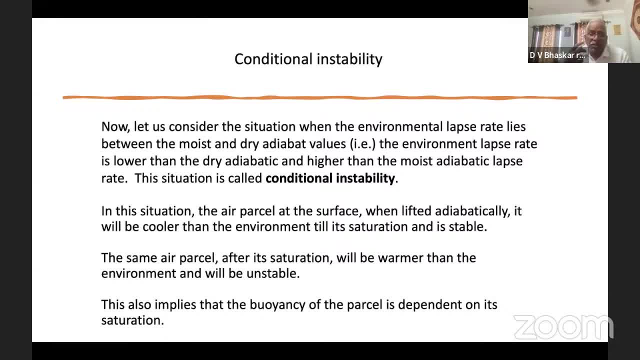 saturation, then from then, after the saturation, it will become warmer than the environment further push upwards. i will also explain to it a little, just a little more. so the, the, the buoyance of the parcel, is very much dependent on saturation. so i explained you: dry instability, moist instability. 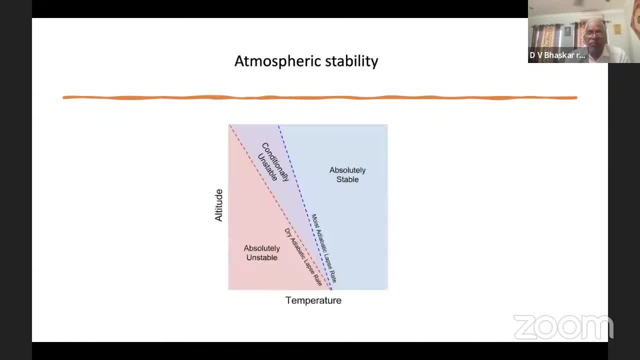 conditional instability. these are the three concepts which are very important. so we see that the dry instability, moist instability, conditional instability, these are the three concepts which are very important. so we see that, if this, if the absolutely unstable, if, if the dry adiabatic lapse rate, 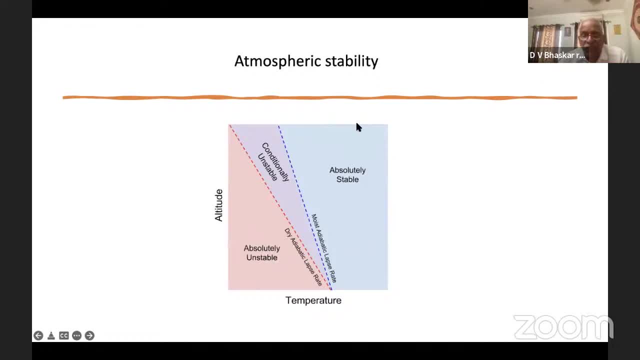 if this, if the absolutely unstable, if. if the dry adiabatic lapse rate, if this, if the absolutely unstable, if. if the dry adiabatic lapse rate. environment lies here. environment lies here. environment lies here if the environmental curve lies in this area. if the environmental curve lies in this area. 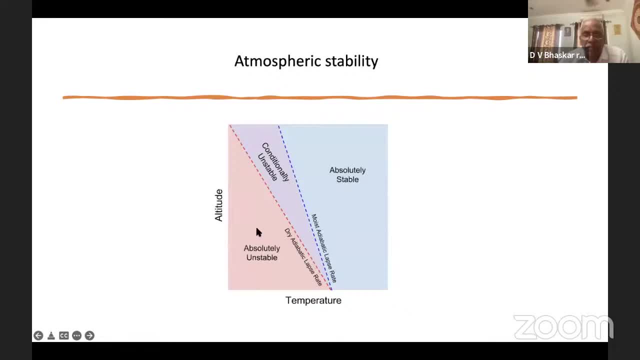 if the environmental curve lies in this area, it is absolutely stable. if the environmental curve, it is absolutely stable. if the environmental curve, it is absolutely stable. if the environmental curve lies between these two, it is conditionally lies between these two. it is conditionally lies between these two. it is conditionally unstable. so the decrease of the temperature. 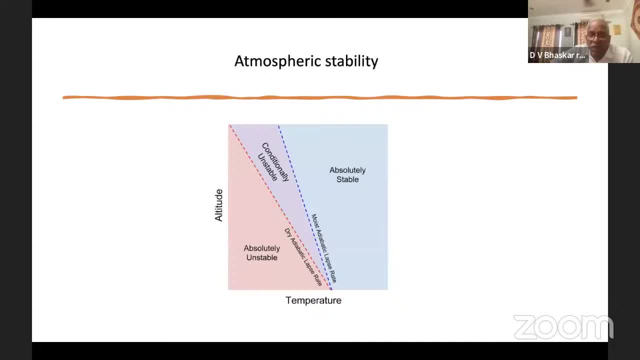 unstable, so the decrease of the temperature. unstable, so the decrease of the temperature. how the temperature decreases in the observed, how the temperature decreases in the observed, how the temperature decreases in the observed atmosphere or the environment, atmosphere or the environment, atmosphere or the environment will give us a clue whether it is. 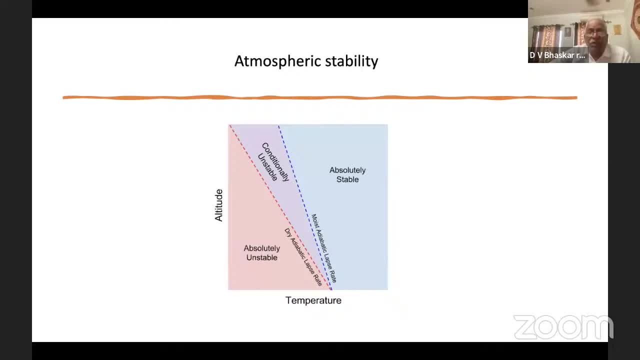 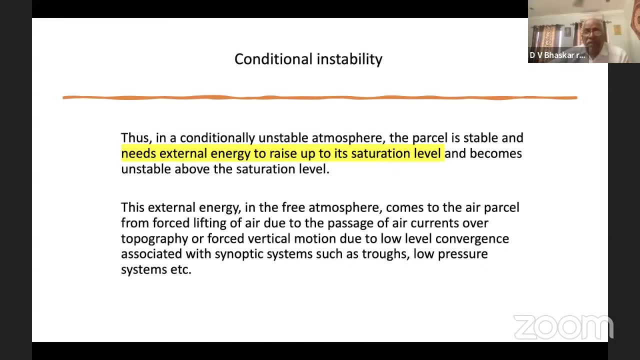 will give us a clue whether it is will give us a clue whether it is conditionally unstable, conditionally unstable, conditionally unstable, absolutely unstable or absolutely stable. and here we know, and here we know, and here we know, as i said, the parcel needs some energy. as i said, the parcel needs some energy. 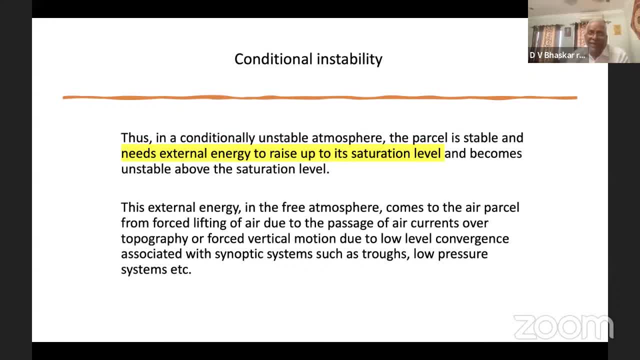 as i said, the parcel needs some energy, some external energy to rise up to its, some external energy to rise up to its, some external energy to rise up to its saturation level. saturation level, saturation level: then it becomes unstable above the. then it becomes unstable above the. then it becomes unstable above the saturation level. so that is what we have. 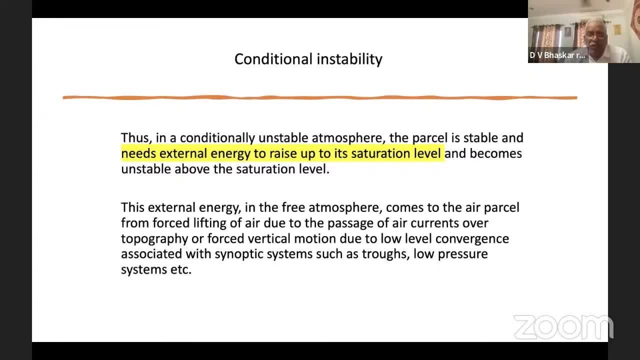 saturation level. so that is what we have. saturation level. so that is what we have seen before, seen before, seen before. so in the free atmosphere, normally the. so in the free atmosphere, normally the. so in the free atmosphere, normally the air parcel. we have seen the observations. air parcel. we have seen the observations. 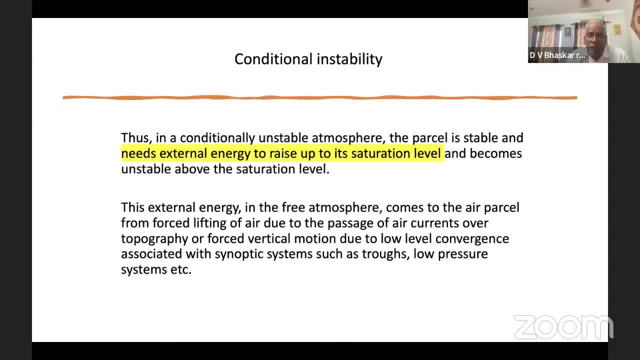 air parcel. we have seen the observations: get some force lifting because of get some force lifting because of get some force lifting because of the movement of the airs over mountains, the movement of the airs over mountains, the movement of the airs over mountains, or or or low-level convergence or friends frontal. 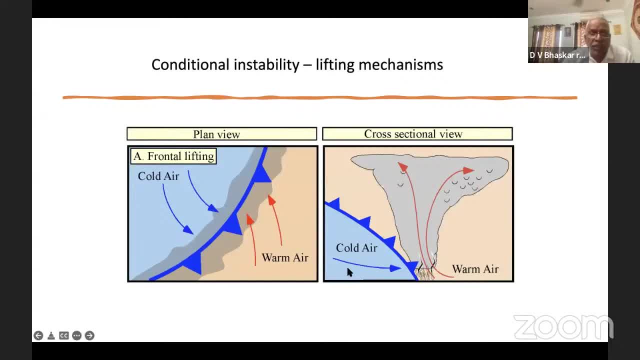 low-level convergence, or friends frontal low-level convergence or friends frontal systems, etc. systems, etc, systems, etc. so i will just show some mechanisms. so if so, i will just show some mechanisms. so if so, i will just show some mechanisms. so if there is a front, cold air and warm air- 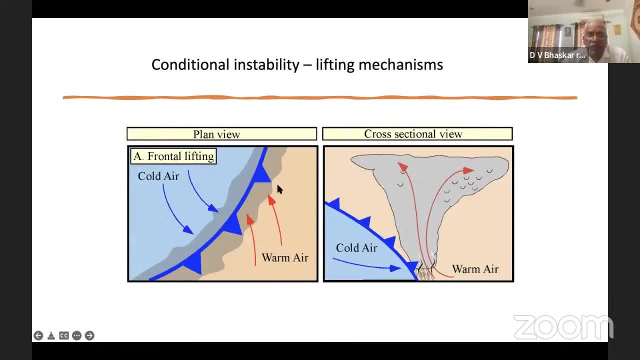 there is a front cold air and warm air. there is a front cold air and warm air. this is a plane view and this is a plane view and this is a plane view. and cold air, warm air, the warm air is forced. cold air, warm air, the warm air is forced. 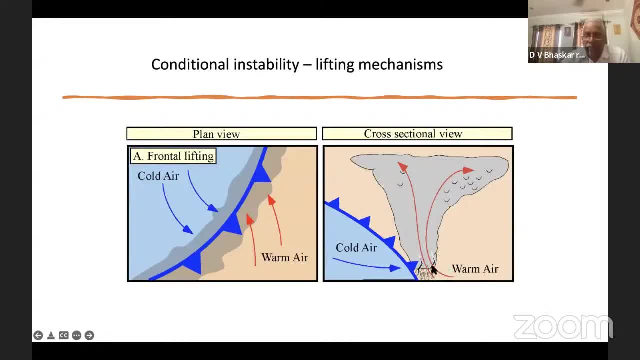 cold air, warm air, the warm air is forced to go up and we will have the force to go up. and we will have the force to go up, and we will have the force lifting up to certain particular point, lifting up to certain particular point, lifting up to certain particular point because cold air is coming down and 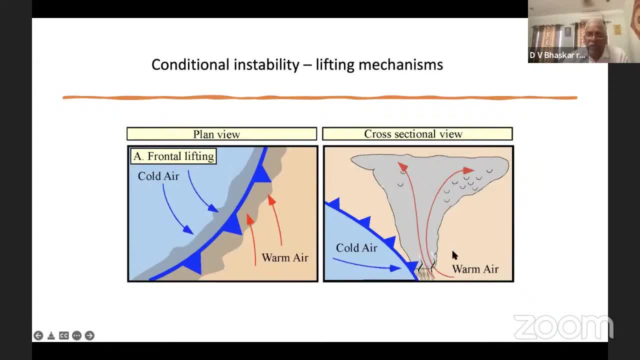 because cold air is coming down, and because cold air is coming down and warm air has to go up, and in this warm air has to go up, and in this warm air has to go up, and in this particular case, you will have a force, particular case, you will have a force. 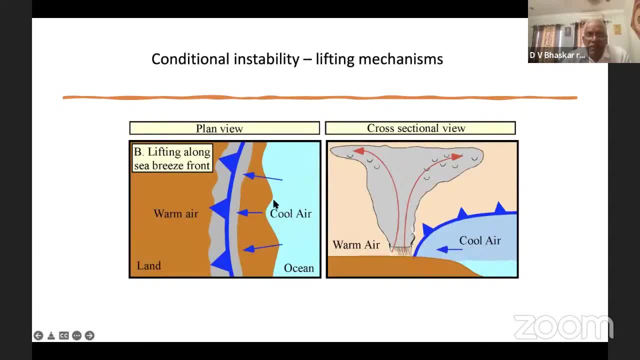 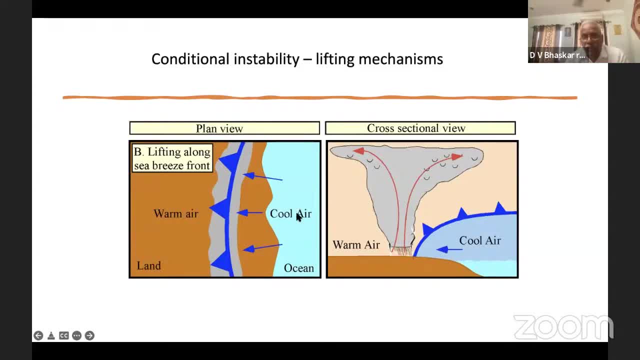 land and then ocean. here it is not land, land and then ocean. here it is not land, ocean, ocean, ocean, land. there's a warm air. there's a cool land. there's a warm air. there's a cool land. there's a warm air. there's a cool, rare during the daytime cooler air from. 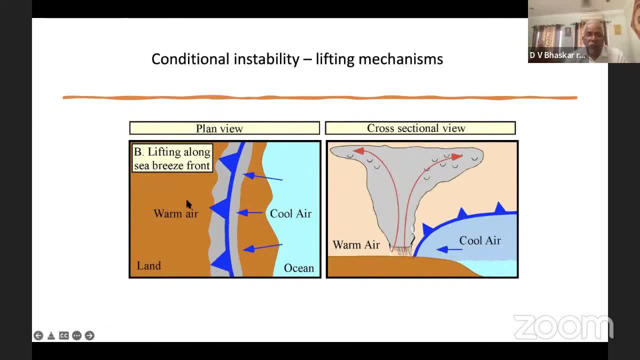 rare during the daytime. cooler air from. rare during the daytime. cooler air from the ocean goes on to the. the ocean goes on to the. the ocean goes on to the. the land because we know land and sea. the land because we know land and sea. the land because we know land and sea breeze. 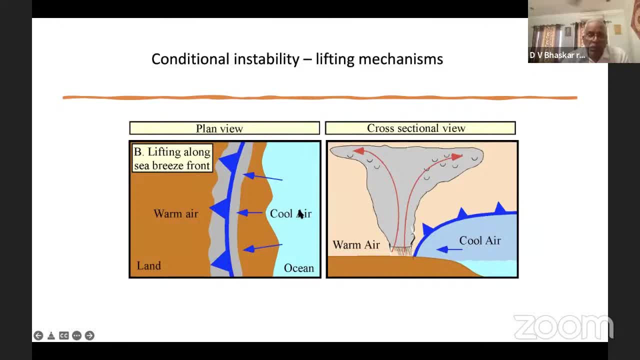 breeze, breeze. and so during the daytime, what happens? and so during the daytime, what happens? and so during the daytime, what happens is the cooler air from the ocean goes, is the cooler air from the ocean goes, is the cooler air from the ocean goes onto this, and then normally this one. 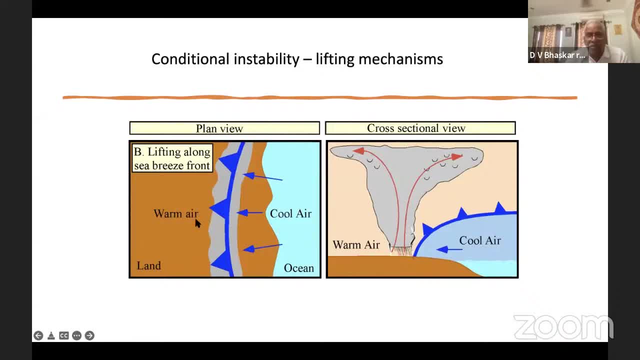 onto this, and then normally, this one onto this, and then normally this one: uh forces the warm air to rise because uh forces the warm air to rise, because uh forces the warm air to rise because the cold air stays at the bottom and the cold air stays at the bottom, and 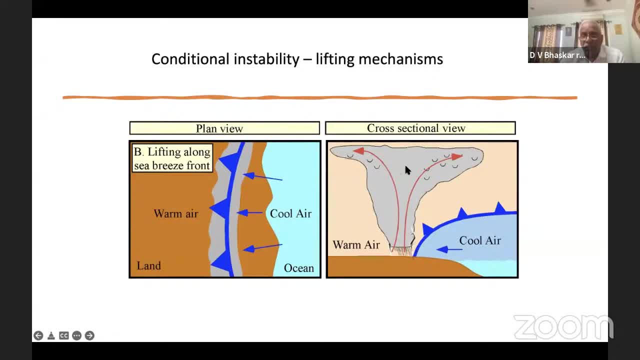 the cold air stays at the bottom and the cross-sectional view, the cold air, the cross-sectional view, the cold air, the cross-sectional view, the cold air forces and the warm air has to go up forces and the warm air has to go up forces and the warm air has to go up. there's one mechanism. this is mountains. 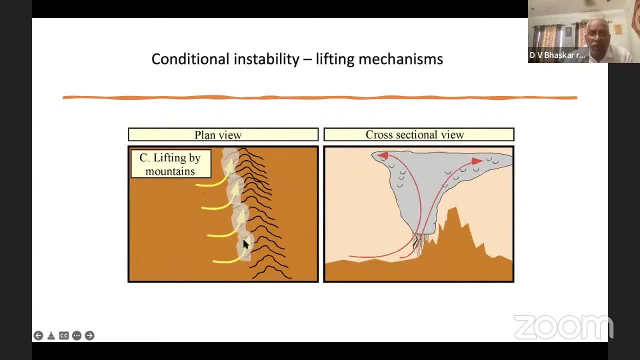 there's one mechanism: this is mountains. there's one mechanism: this is mountains. so you have a mountain straight out, the. so you have a mountain straight out, the. so you have a mountain straight out, the air has to. air has to air has to pass over the mountain. so when it goes up, 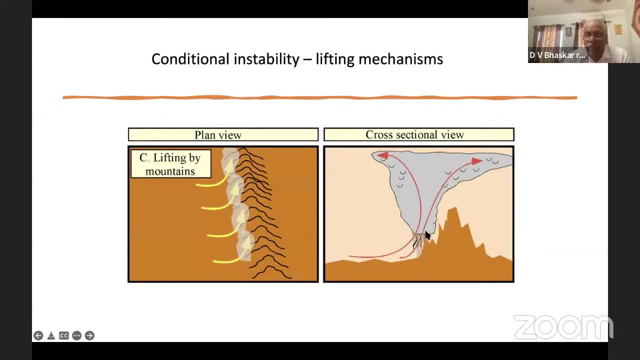 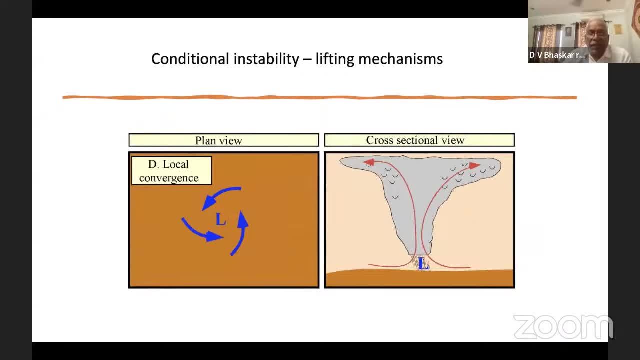 pass over the mountain. so, when it goes up, pass over the mountain. so when it goes up, the air has to go up to some level, the air has to go up to some level, the air has to go up to some level. and, and and another important thing is, you have 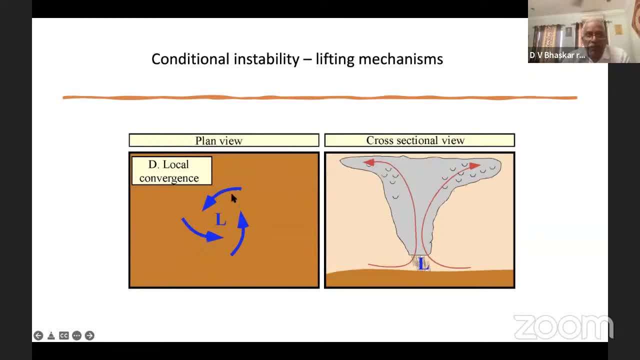 another important thing is you have. another important thing is you have the, the the low level convergence, low level, low level convergence, low level, low level convergence, low level convergence, convergence, convergence. you have a low pressure, you have a low pressure, you have a low pressure, dynamical reasons. there is a convergence. 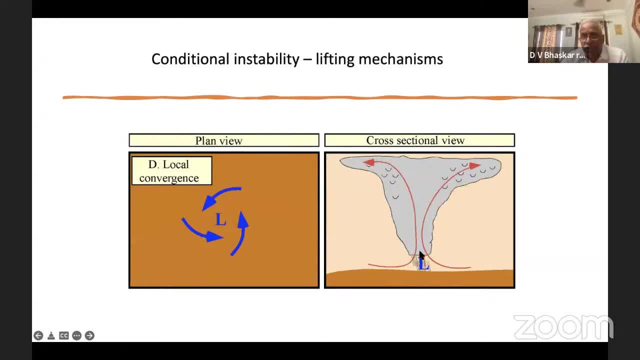 dynamical reasons there is a convergence. dynamical reasons there is a convergence at the lower levels. and this low level at the lower levels and this low level at the lower levels and this low level forced convergence will make the parcel forced. convergence will make the parcel forced. convergence will make the parcel go up. so this is a force lifting that. 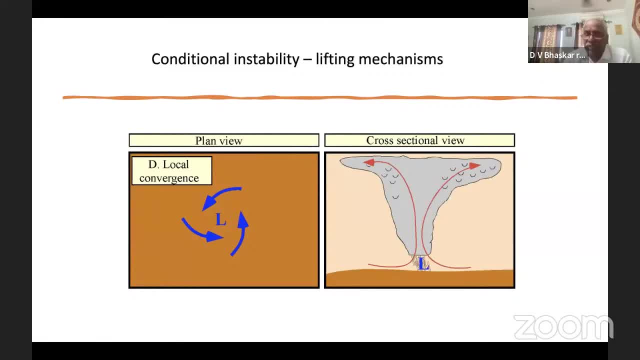 go up. so this is a force lifting that go up. so this is a force lifting that will help the parcel to go up to some will help the parcel to go up to some will help the parcel to go up to some level, level, level, till it, till it gets saturation. so these 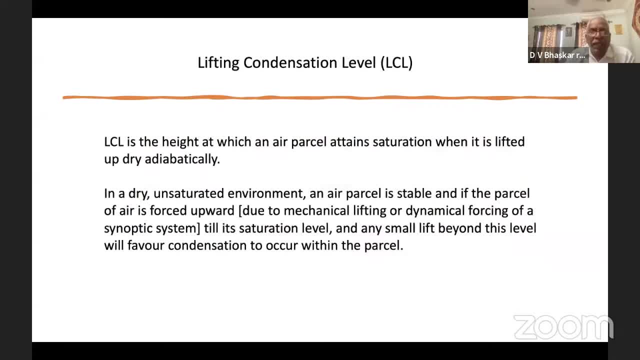 till it till it gets saturation. so these: till it till it gets saturation. so these are some lifting mechanisms which i are some lifting mechanisms which i are some lifting mechanisms which i wanted to show, wanted to show, wanted to show, and and and now we will. i will just take few more. 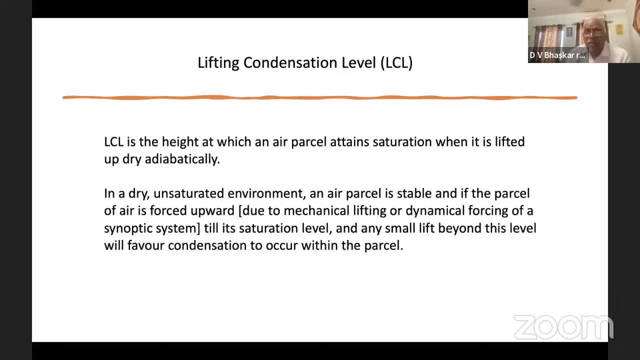 now we will. i will just take few more now we will. i will just take few more minutes, minutes, minutes to finish, but we have some to finish, but we have some to finish. but we have some important concepts like lifting, important concepts like lifting, important concepts like lifting, condensation level. 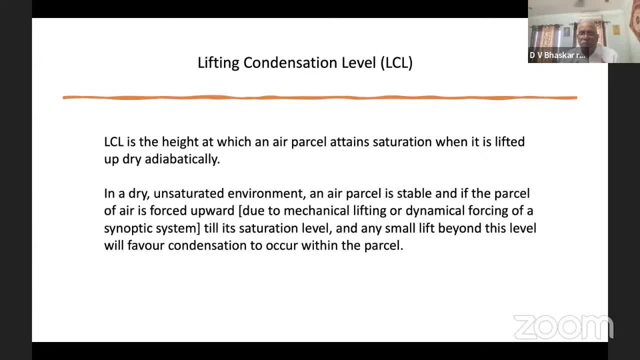 condensation level. condensation level. so though i have explained to you uh the, so though i have explained to you uh the, so though i have explained to you, uh the point of saturation, point of saturation. point of saturation, the, the convection where the latent heat, the the convection where the latent heat. 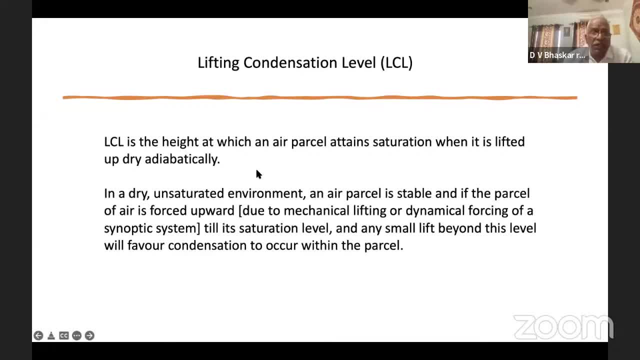 the, the convection where the latent heat release, release, release starts happening. but we see, here starts happening. but we see, here starts happening. but we see here i define the level, a level that is called: i define the level, a level that is called: i define the level, a level that is called lifting condensation level. 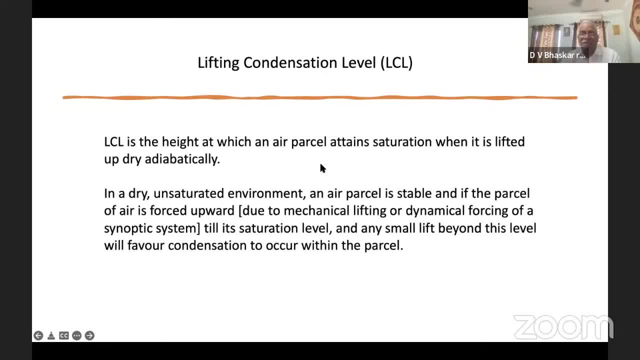 lifting condensation level. lifting condensation level is the height at which the air parcel is. the height at which the air parcel is the height at which the air parcel attains saturation when it is lifted. attains saturation when it is lifted. attains saturation when it is lifted dry adiabatically. 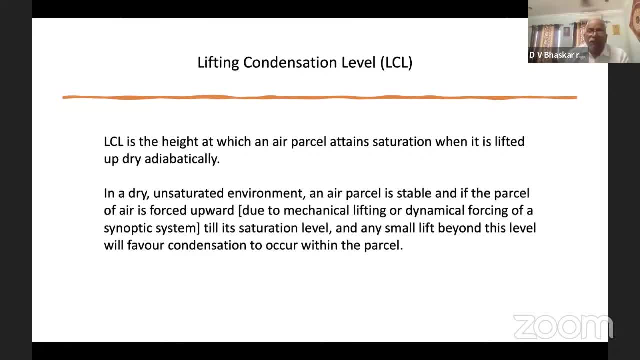 dry adiabatically, dry adiabatically. so i explained to when the air parcel, so i explained to when the air parcel. so i explained to when the air parcel from the surface. when it is given some from the surface, when it is given some from the surface, when it is given some energy, it goes up and it gets. 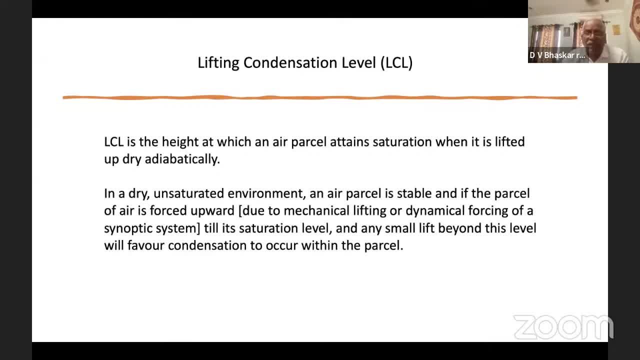 energy, it goes up and it gets energy, it goes up and it gets saturation at one point. so that saturation at one point, so that saturation at one point, so that particular level, where the parcel particular level, where the parcel particular level, where the parcel attains saturation, is called the lifting. 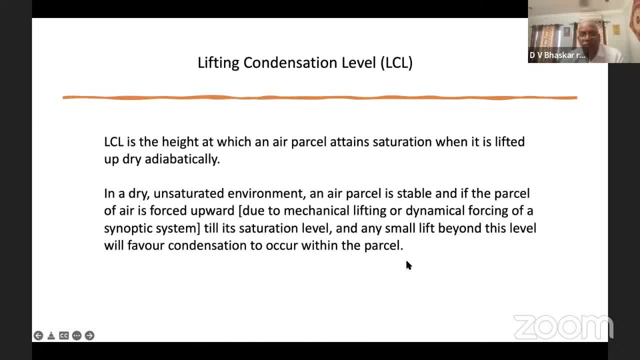 attains saturation is called the lifting attains saturation is called the lifting condensation level, as i said again the. in the dry unsaturated, as i said again the. in the dry unsaturated, as i said again the in the dry unsaturated environment. the parcel, air parcel. 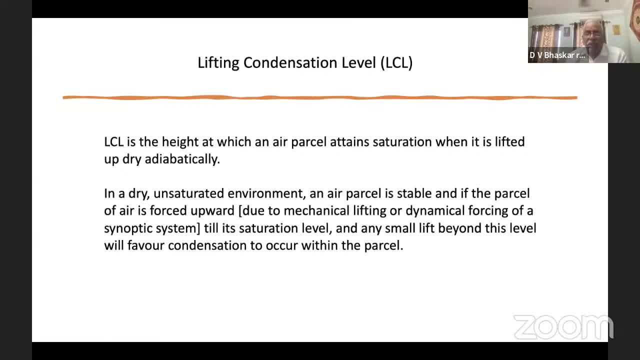 environment, the parcel air parcel environment, the parcel air parcel is stable and if the air parcel is is stable and if the air parcel is is stable and if the air parcel is forced upward due to some mechanical forced upward, due to some mechanical forced upward, due to some mechanical lifting or dynamical lifting, mechanical 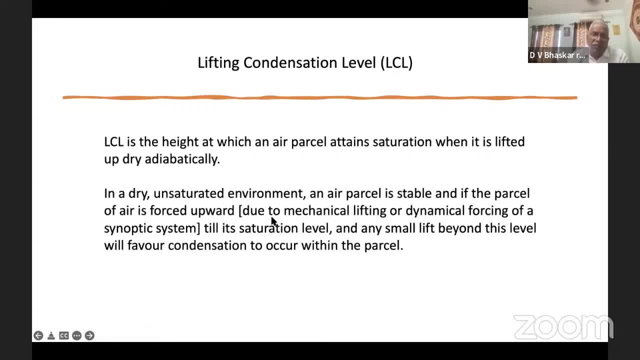 lifting or dynamical lifting, mechanical lifting or dynamical lifting. mechanical means some topography, or dynamical means some topography, or dynamical means some topography, or dynamical lifting means some low level, lifting means some low level lifting means some low level convergence, etc. till its saturation and 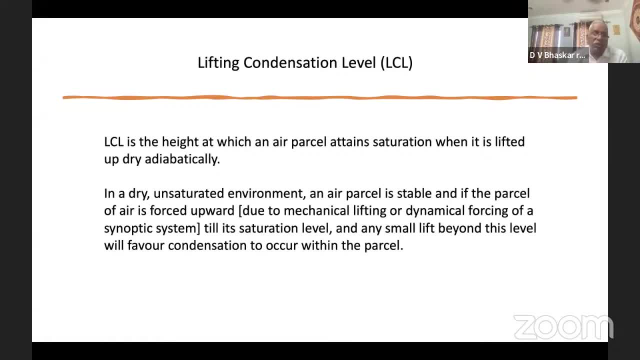 convergence etc till its saturation, and convergence etc till its saturation, and any small lift beyond this level will any small lift beyond this level, will any small lift beyond this level will favor condensation. so lifting favor condensation. so lifting favor condensation. so lifting condensation is the level. 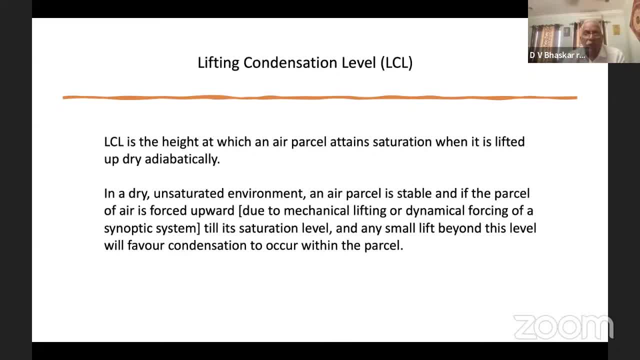 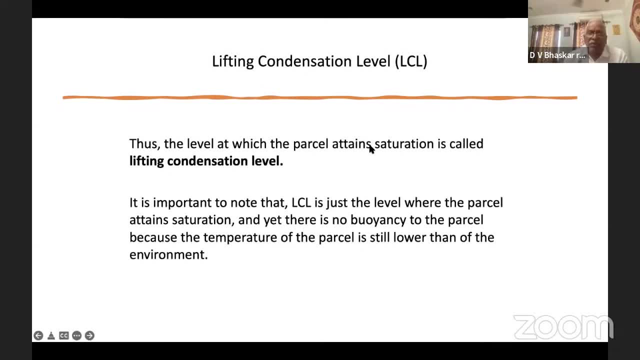 condensation is the level. condensation is the level. parcel attains saturation. it is very. parcel attains saturation. it is very, parcel attains saturation. it is very important to remember that, important to remember that, important to remember that and so and so and so again, it is the same one: the parcel. 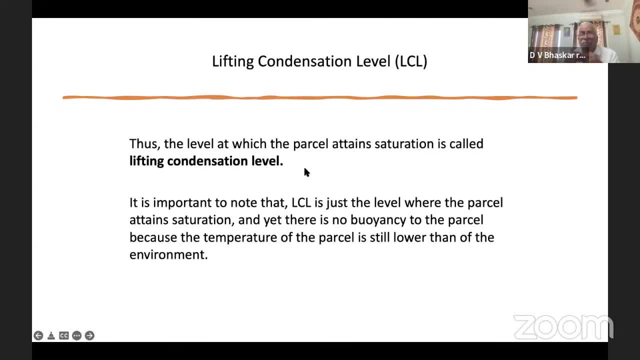 again, it is the same one. the parcel: again, it is the same one. the parcel attains saturation. it is the lifting attains saturation. it is the lifting attains saturation. it is the lifting condensation level, condensation level, condensation level it has. it is very important for you to 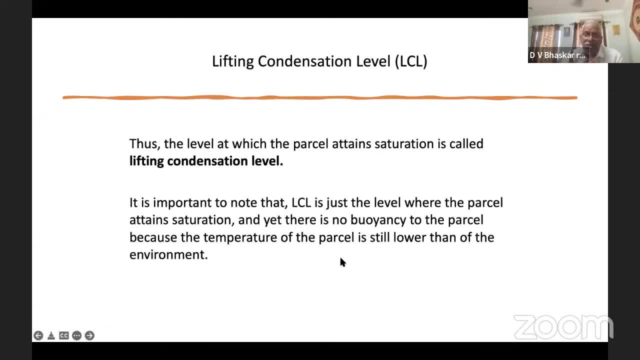 it has. it is very important for you to it has. it is very important for you to note here, note here, note here, that that that the lifting condensation is level, the lifting condensation is level, the lifting condensation is level, is just, is the level at which the parcel. 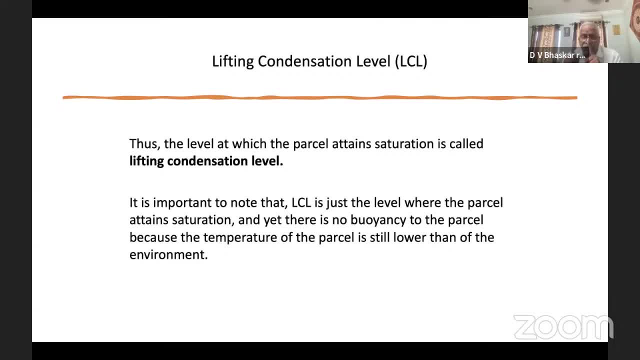 is just is the level at which the parcel is. just is the level at which the parcel gets saturation, but that there is no gets saturation, but that there is no gets saturation but that there is no buoyancy to the parcel is very important. buoyancy to the parcel is very important. it it just got saturated. the 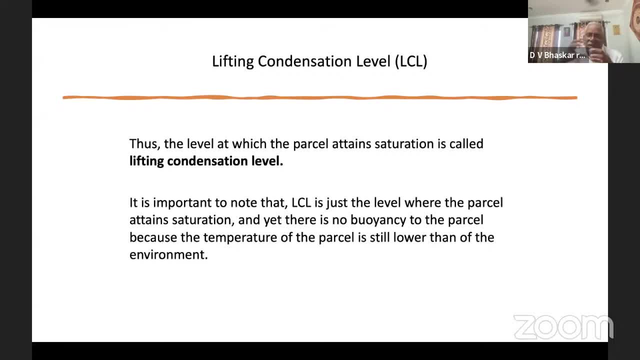 it. it just got saturated. the it it just got saturated. the temperature attained by the parcel is. temperature attained by the parcel is temperature attained by the parcel is. just meets the requirement of the just meets the requirement of the just meets the requirement of the air parcel to be saturated. that means 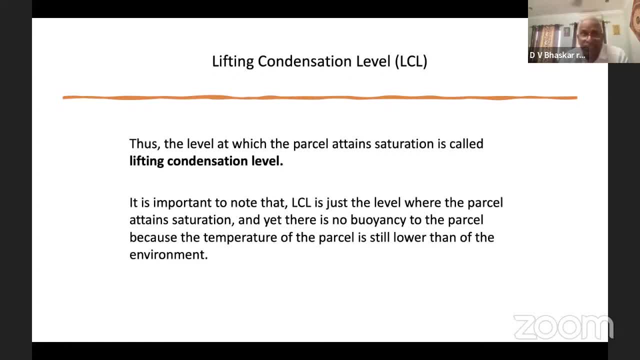 air parcel to be saturated. that means air parcel to be saturated. that means it can hold only the number of water. it can hold only the number of water. it can hold only the number of water vapor molecules. it had inside vapor molecules. it had inside vapor molecules, it had inside. so it is only the level at which the 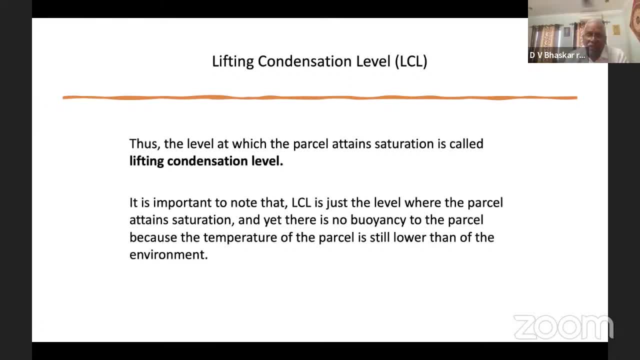 so it is only the level at which the so it is only the level at which the parcel attains saturation, yet at this parcel attains saturation, yet at this parcel attains saturation. yet at this level, there is no buoyancy. the level there is no buoyancy, the 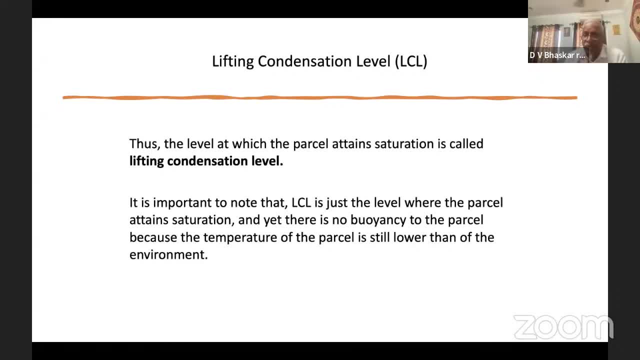 level. there is no buoyancy. the temperature inside the parcel is still. temperature inside the parcel is still. temperature inside the parcel is still lower than the environment. this is very lower than the environment. this is very lower than the environment. this is very important for you to note. 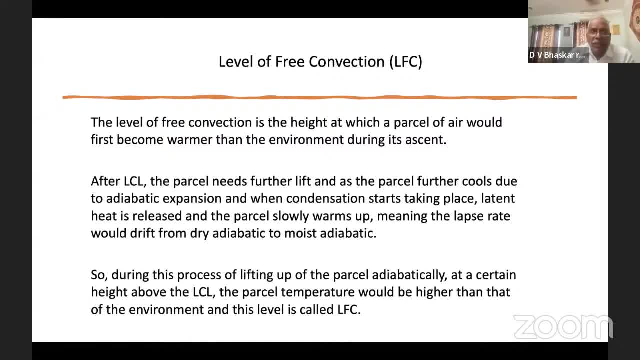 important for you to note, important for you to note, and and, and we see a level of free convection. we see a level of free convection. we see a level of free convection that means that means, that means if, if, if, if, the, if the parcel is still 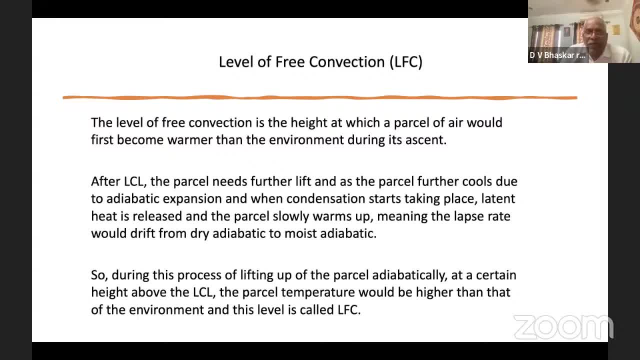 if the, if the parcel is still, if the, if the parcel is still lifted upward, lifted upward, lifted upward, beyond, beyond, beyond the lifting condensation level, because at the lifting condensation level, because at the lifting condensation level, because at the lifting condensation level the parcel. 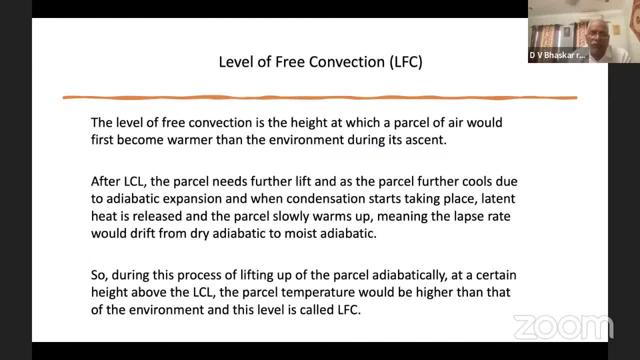 the lifting condensation level, the parcel, the lifting condensation level, the parcel has become saturated still. if you give a has become saturated still. if you give a has become saturated still. if you give a small lift, the parcel is moving up. and small lift, the parcel is moving up. and 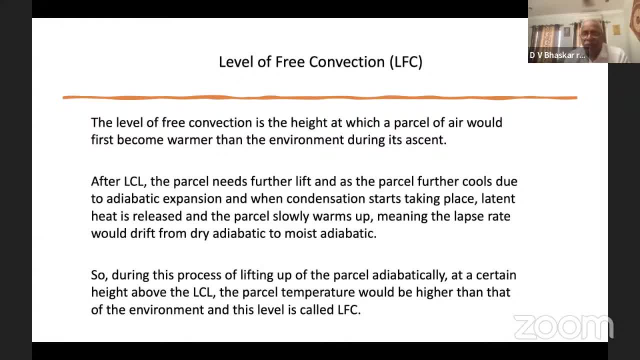 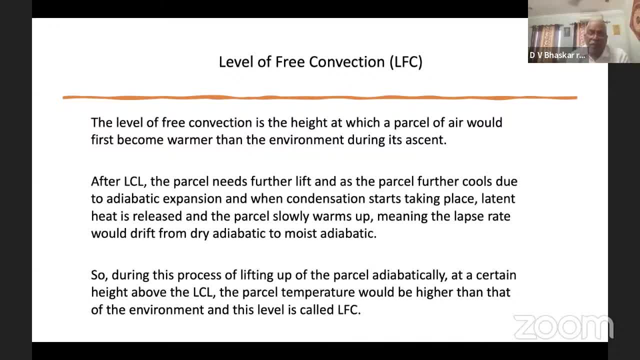 reduces further. at the lcl, the temperature was just enough to make it. temperature was just enough to make it. temperature was just enough to make it saturated. but if it still gets lower saturated, but if it still gets lower saturated, but if it still gets lower, if the temperature decreases further due 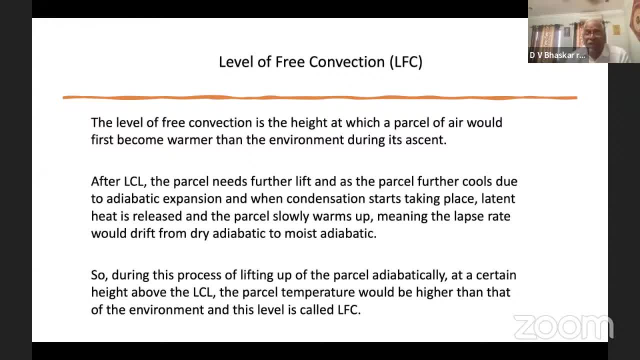 if the temperature decreases further due. if the temperature decreases further due to the further lift upwards from the to the further lift upwards from the to the further lift upwards from the lcl, what happens is the temperature lcl. what happens is the temperature lcl. what happens is the temperature decreases a little more and then at that. 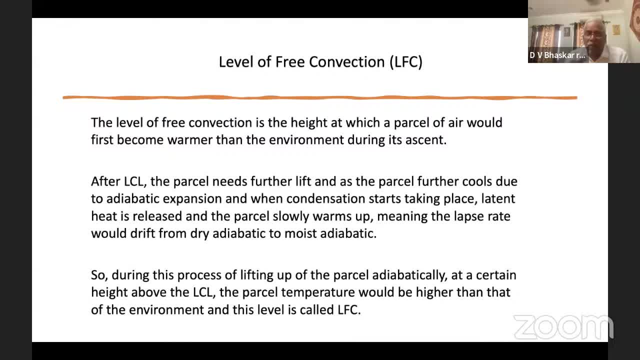 decreases a little more, and then at that decreases a little more, and then at that particular point, particular point, particular point, there is no, it cannot hold the water. there is no, it cannot hold the water. there is no, it cannot hold the water, water vapor molecules it had inside and 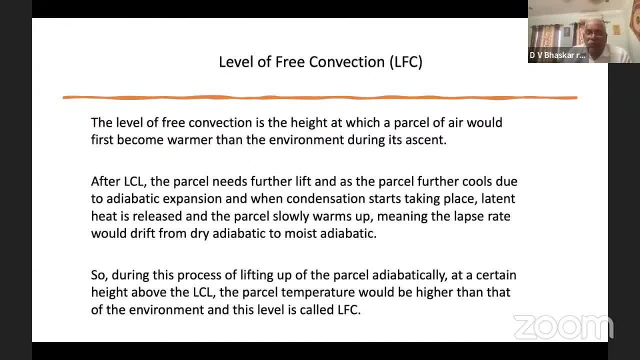 water vapor molecules it had inside, and water vapor molecules it had inside, and the latent heat, the latent heat, the latent heat, the condensation takes place. that means the condensation takes place. that means the condensation takes place. that means water vapor start getting converted into water vapor start getting converted into 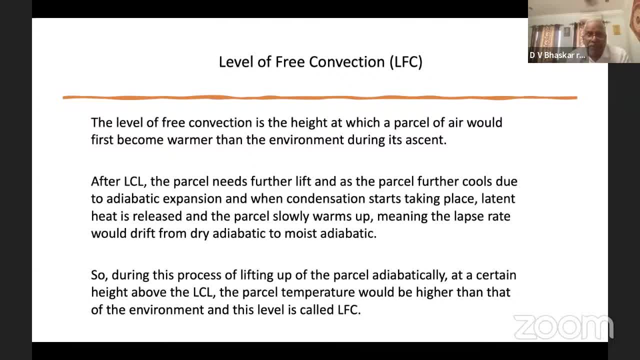 water vapor start getting converted into liquid water and latent heat is released. liquid water and latent heat is released. liquid water and latent heat is released. this is the point at which this is the point at which this is the point at which the the heating of the parcel, really. 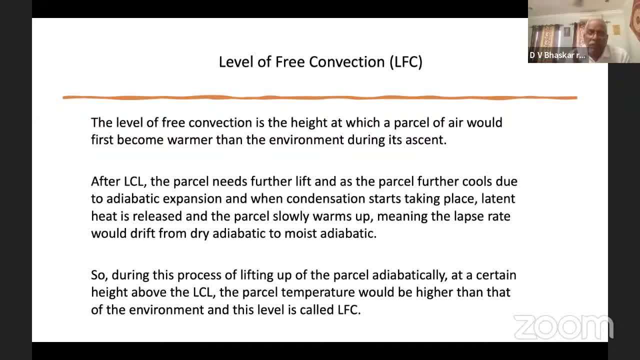 the, the heating of the parcel, really the. the heating of the parcel. really really up to that? the parcel is only really up to that. the parcel is only really up to that. the parcel is only subjected to cooling, subjected to cooling, subjected to cooling, expansion and cooling. and here also 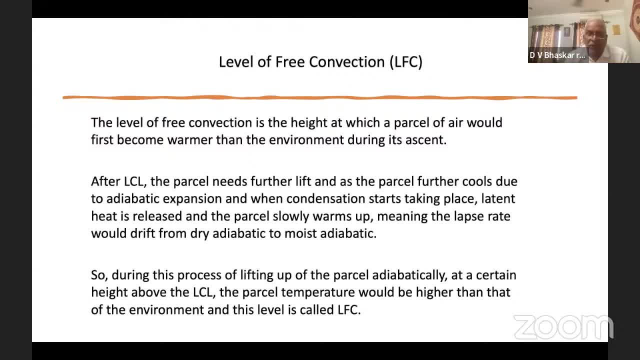 expansion and cooling, and here also expansion and cooling. and here also even the parcel gets lifted up, the even the parcel gets lifted up, the even the parcel gets lifted up. the pressure pressure pressure with the environment is still lower, the with the environment is still lower, the with the environment is still lower, the and it is subjected to expansion, the 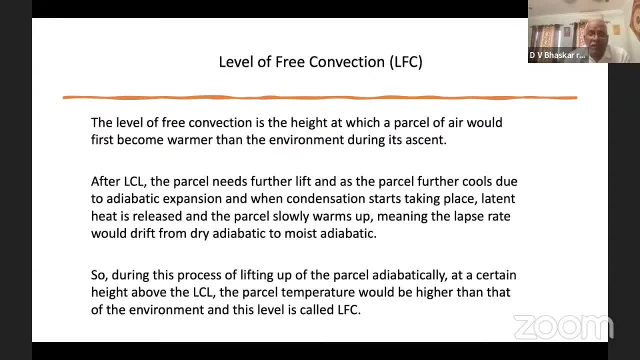 and it is subjected to expansion. the and it is subjected to expansion. the parcel has to parcel has to. parcel has to be cooler. it gets cooler, but not at the. be cooler, it gets cooler, but not at the. be cooler, it gets cooler, but not at the dry adiabatic. 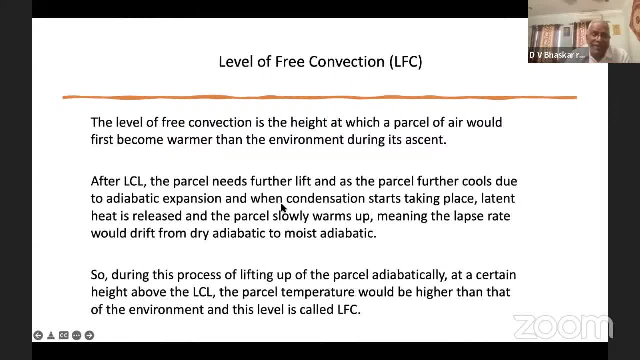 dry adiabatic. dry adiabatic rate because when condensation takes rate, because when condensation takes rate, because when condensation takes place, latent heat is released. that will place latent heat is released. that will place latent heat is released. that will help the parcel. 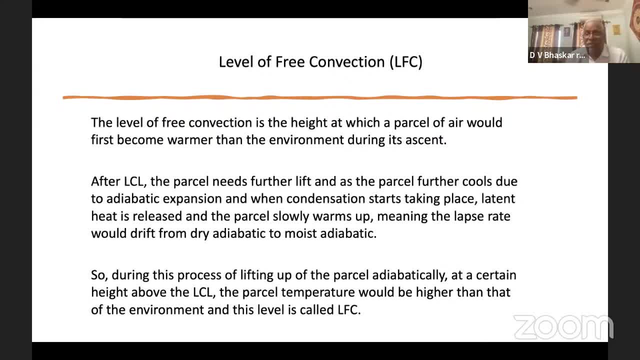 help the parcel, help the parcel warm up, warm up, warm up then then, then then that means the temperature decrease, then that means the temperature decrease, then that means the temperature decrease from this particular point where the from this particular point, where the from this particular point where the condensation takes place, lifting. 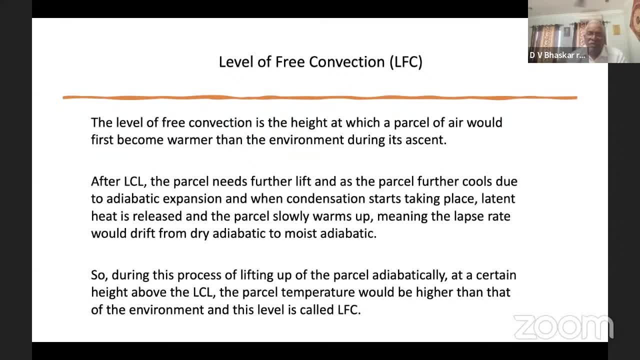 condensation takes place. lifting condensation takes place. lifting condensation level is not the level where condensation level is not the level where condensation level is not the level where the condensation takes place. it is the the condensation takes place. it is the the condensation takes place. it is the level where the parcel gets saturated. 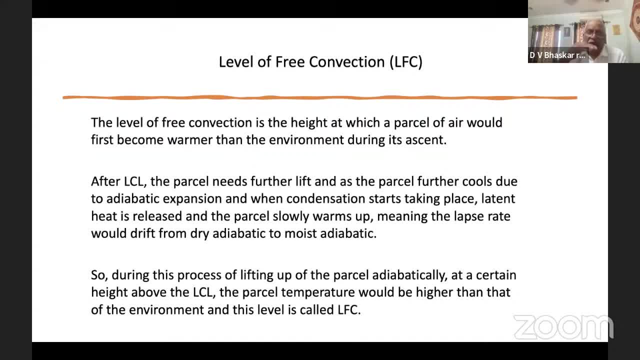 level where the parcel gets saturated, level where the parcel gets saturated, but still from that particular point a, but still from that particular point a, but still from that particular point. a little more of upward lift is necessary. little more of upward lift is necessary. little more of upward lift is necessary for the parcel to get a little more. 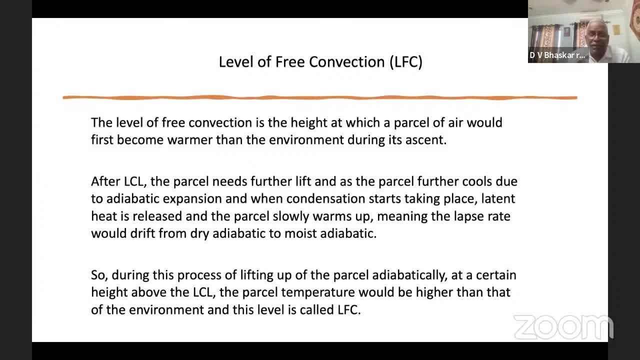 for the parcel to get a little more, for the parcel to get a little more cooled up water vapor to get condensed, cooled up water vapor to get condensed, cooled up water vapor to get condensed, and that condensation process and that condensation process and that condensation process will release latent heat. that release 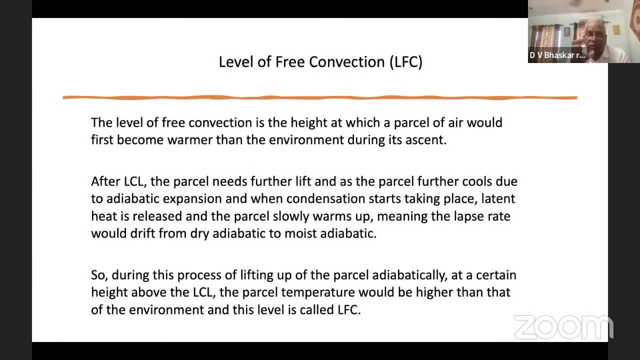 will release latent heat. that release will release latent heat. that release latent heat will warm up the parcel. so latent heat will warm up the parcel. so latent heat will warm up the parcel. so the rate of the parcel from dry adamant: the rate of the parcel from dry adamant. 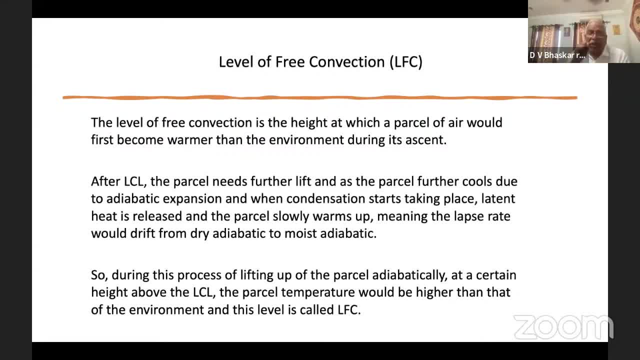 the rate of the parcel from dry adamant to moisture debate. so this concept is to moisture debate. so this concept is to moisture debate. so this concept is very important. so lcl is different level very important. so lcl is different level, very important. so lcl is different. level of free convection is different, it is. 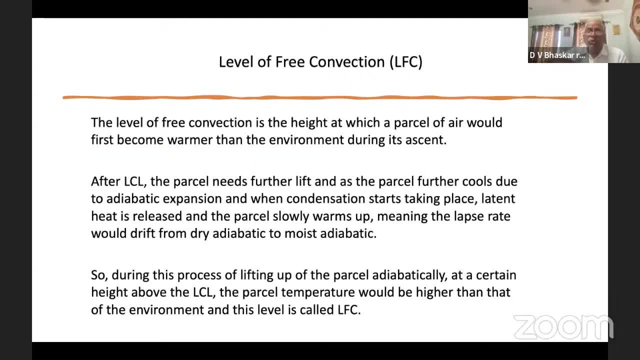 of free convection is different. it is of free convection is different. it is the level of the free convection. from the level of the free convection, from the level of the free convection from which the convection would start taking, which the convection would start taking. 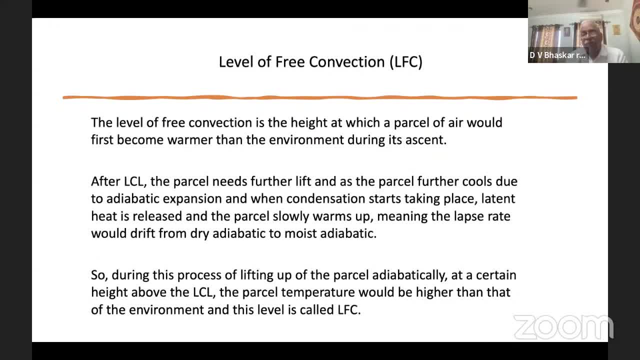 which the convection would start taking place. that means that is the point of place. that means that is the point of place. that means that is the point of the level at which water vapor starts. the level at which water vapor starts, the level at which water vapor starts getting condensed. water vapor got, gets. 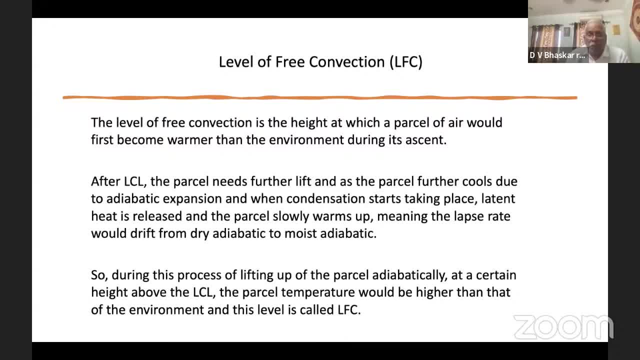 getting condensed. water vapor got gets getting condensed. water vapor got gets converted into liquid water. this is very converted into liquid water. this is very converted into liquid water. this is very important, important, important, so. so so, during the, during the lifting of the, during the, during the lifting of the, 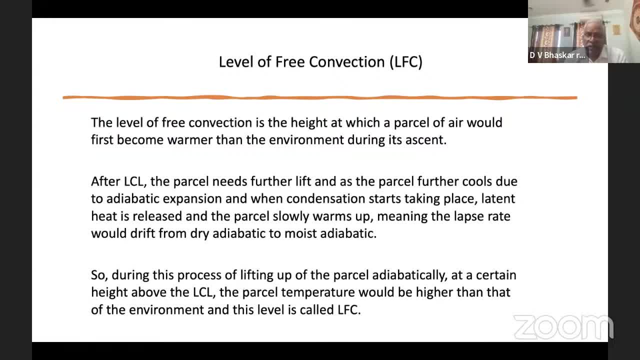 during the during the lifting of the parcel, parcel parcel adiabatically first up to the lcl. it adiabatically first up to the lcl. it adiabatically first up to the lcl it needs, needs, needs some lift and then it will. 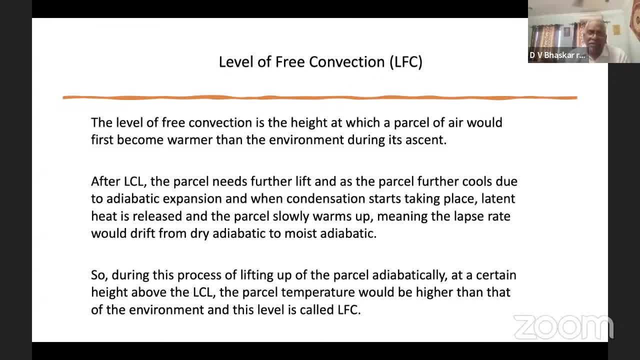 some lift and then it will some lift, and then it will reach a saturation, but reach a saturation, but reach a saturation, but still it needs a small lift further up. still it needs a small lift further up. still it needs a small lift further up, then only the parcel. 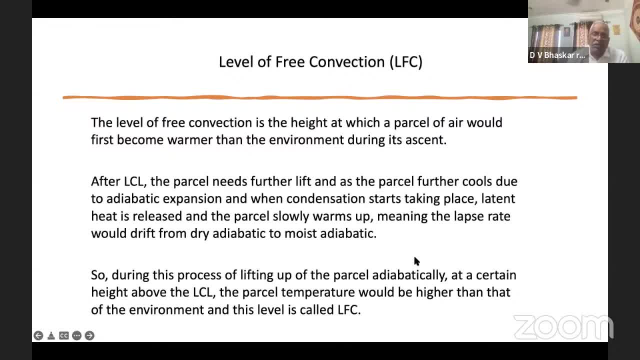 then only the parcel still a little more cooler temperatures and the parcel temperature would be higher from that particular point of the LFC level of free convection. the parcel is warmer than the environment, so the buoyancy would start from the level of free convection, so above. 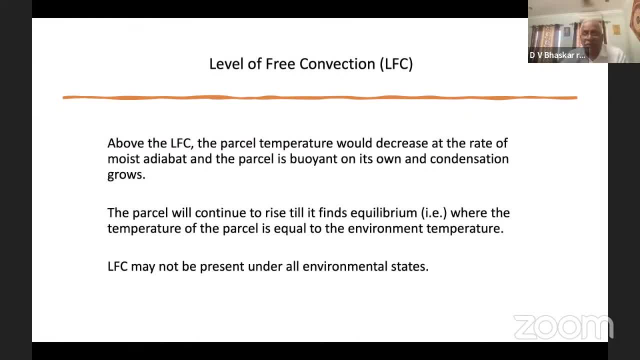 the LFC lifting level of free convection. the parcel temperature would decrease at the rate of moisture deborah and the parcel is buoyant on its own and condensation grows and this parcel will rise until it finds equilibrium. that means the rise will continue again till the parcel will 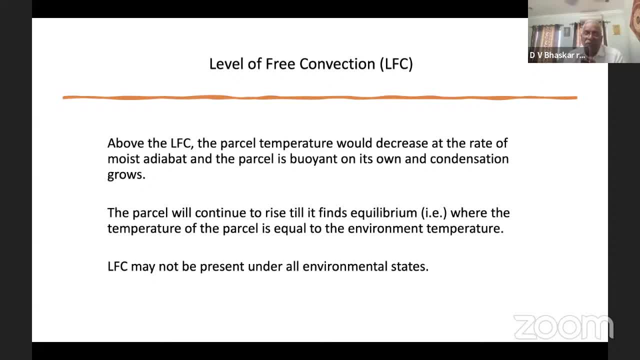 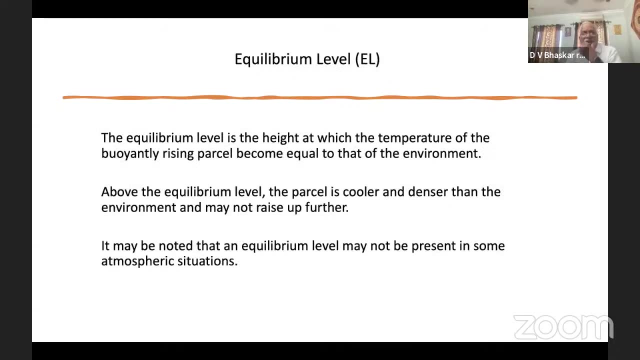 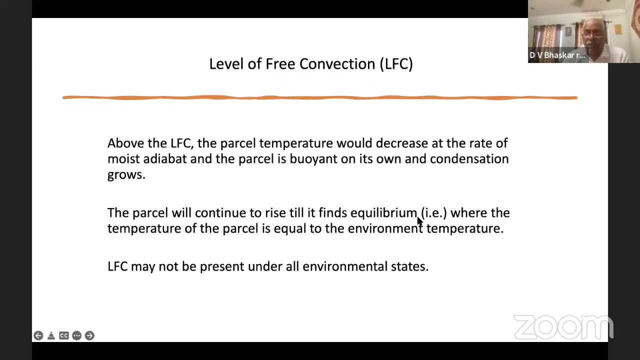 have its temperature equaling the environmental temperature value. sometimes LFC may not be present. all at under all. equilibrium level may not be present. LFC may not be present under all environment states. so I also explained this equilibrium level because I said the parcel will continue to rise until it finds equilibrium. so the equilibrium level is the height at which the 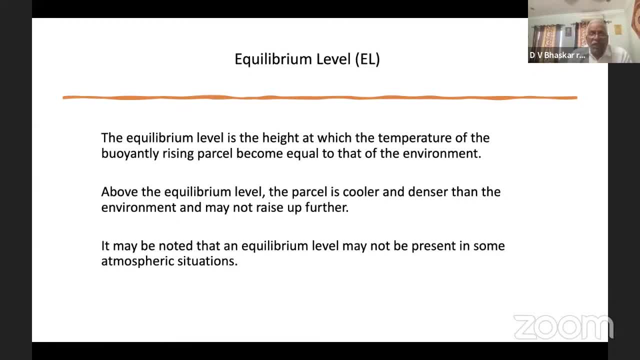 temperature of the parcel, which is rising from the LFC level of free convection. it rises up because it is thermally buoyant and then it goes up and goes up. the temperature gets decreased at the saturated adiabatic level and at some particular height where it, where the, where the temperature in the of the parcel. 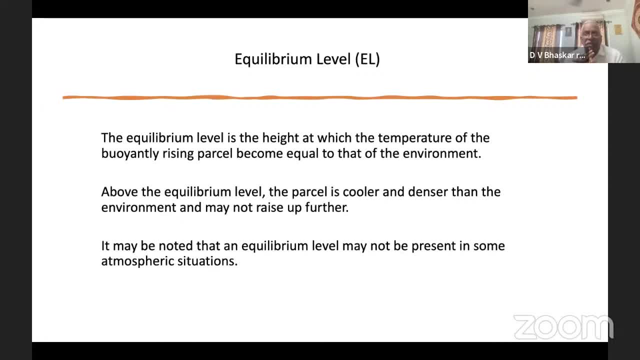 is equal to that of the environment, then that is defined as the equilibrium level, above which, above which normally the parcel will be cooler than the environment and would not raise further. so equilibrium level is the level at which the environment, air, parcel temperature would be, would become equal to the temperature of the parcel and the temperature of the parcel would. 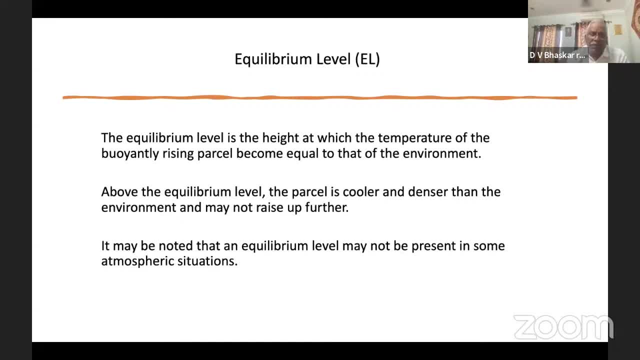 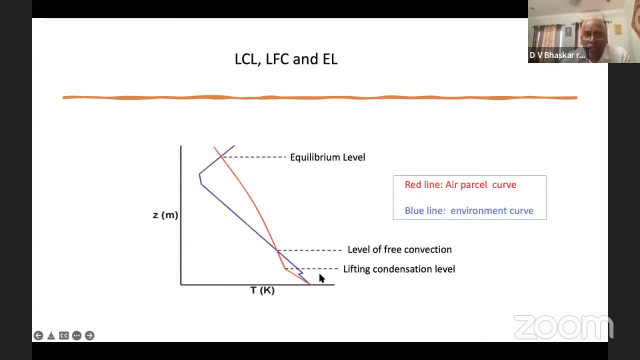 not be equal to the environment temperature. but equilibrium level may not be present under all atmospheric conditions. so here I would show this blue curve is the environment observed temperature profile and at this surface we have the air parcel. it is being lifted. when it is being lifted, it is lifted up to this. and at the lifting condensation level. these atmosphere conditions may not be present here. within all this atmospheric conditions and on the taken, lihat up to this figure, this is every possible condition on the stadium And at the lifting condensation level it gets saturated. 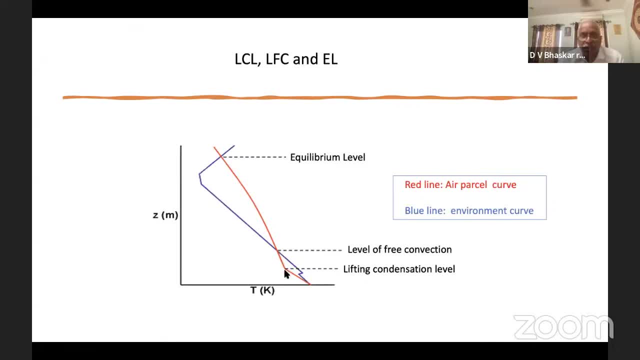 Okay, Up to this level the parcel is saturated And above this level the parcel is having its temperature decreased. at the saturated adiabatic collapse rate, But at the level of the free convection, the temperature, the water vapor inside the parcel starts getting condensed. 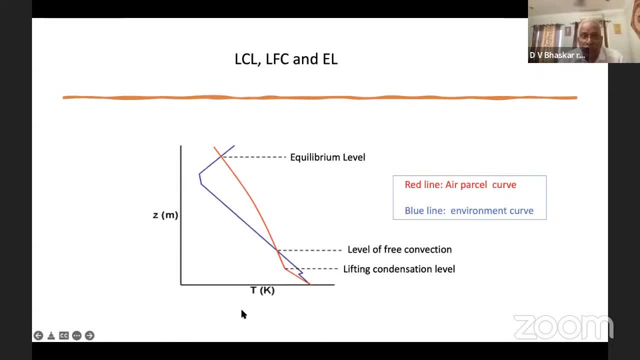 So this is the point at which, from the lifting condensation level, the temperature decreases at the saturation level, but there is no condensation, as said. But at this particular point, which is denoted as the level of free convection, And from this particular point onwards, what happens is water vapor to liquid water, condensation process takes place. 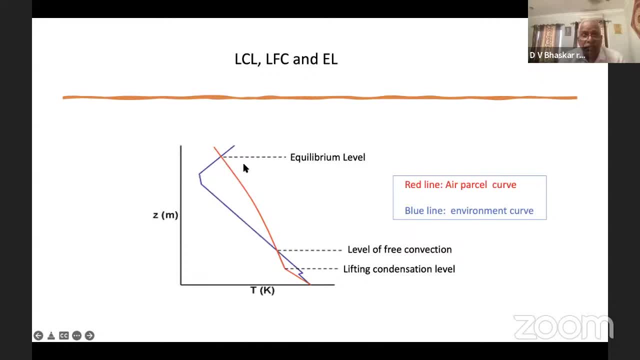 And from here it is thermally buoyant And as it goes up along the saturated adiabatic, the environmental curve, if it crosses the environment curve at some level, it is called equilibrium, And above that particular level this parcel is cooler than the environment. 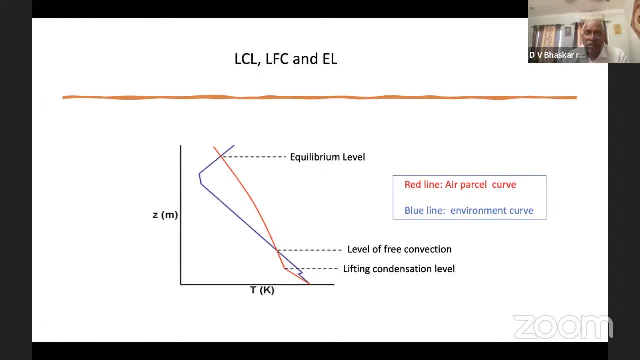 And so it would be stable. It's not buoyant anymore. So, for an example, I have shown you the environment curve and how the air parcel would have its temperature getting controlled as a dry adiabat, saturated adiabat, first attaining the saturation level that is called the lifting condensation level. 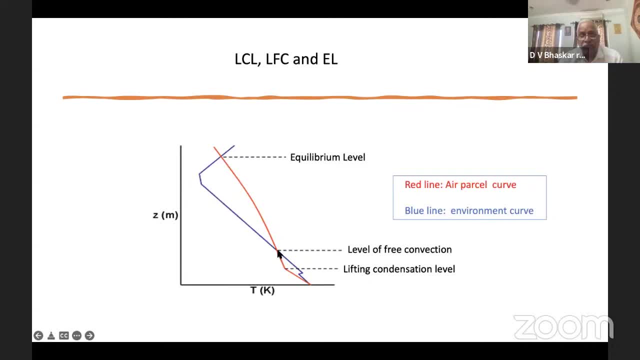 And above that, the level of free convection where exactly the air parcel is. So the air parcel would have its change of the phase: water vapor getting converted, liquid water starts taking place, And from that one the parcel would be completely buoyant. 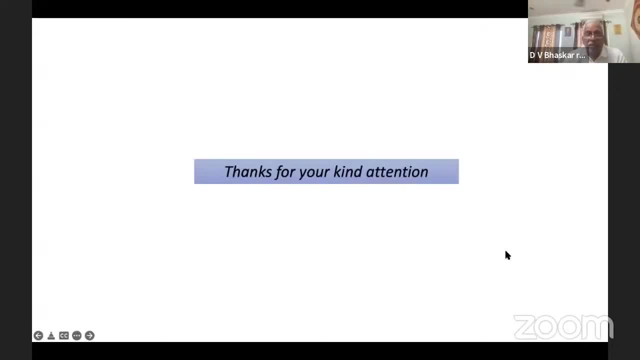 I think I have explained to you whatever I wanted to tell first about the dry adiabatic lapse rate, moist adiabatic lapse rate, mathematical expressions for that. Then I have explained to you what is stability, what is instability in the atmosphere, how the air 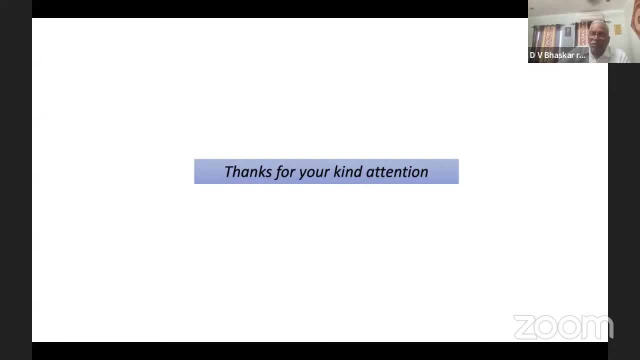 And what is how the thermal buoyancy plays an important role. I have explained to the conditions in a dry atmosphere, comparing the dry adiabatic lapse rate and the moist environment. with the moist adiabatic lapse rate, What is absolute stability? what is absolute instability? 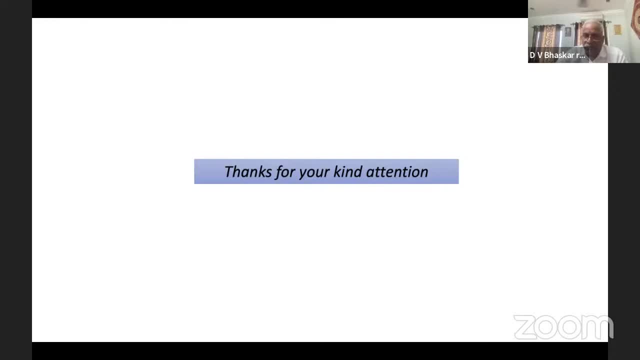 Then the three important points: lifting condensation level, level of free convection and the equilibrium level. I think that is what I wanted to say today. Thank you very much for your kind attention And I would be very happy to give any clarifications that the students want. 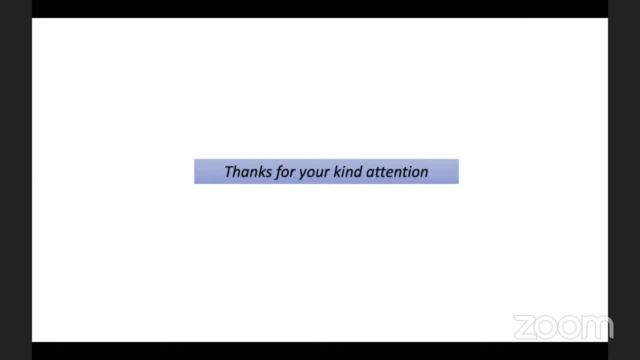 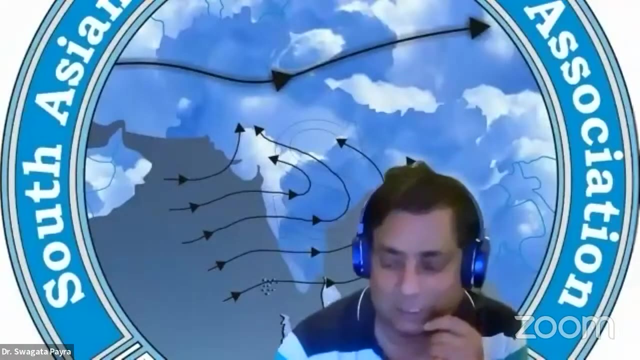 Thank you sir. Yeah, thank you sir. It was very detailed and nice lecture. I would invite Dr Swagata to take the question answer session. Yeah, thanks a lot, Dr Rohini. And thanks a lot, sir, for all the details about the stability class. 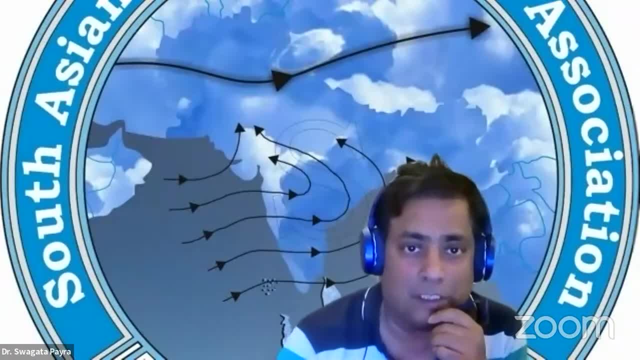 Because there are a lot of things. It depends on the details whether actually happens due to different stabilises class, Like I need fall stable condition or cyclone, I don't need a stable conditions, All these things. So there are a few questions related to that. I start with a question: Bad weather conditions happen under unstable or stable conditions? Mostly it was He wanted to write: Bad weather conditions happen under unstable or stable conditions, But conditions- unstable bad weather means you have the cloud formation, you have the rain occurring. 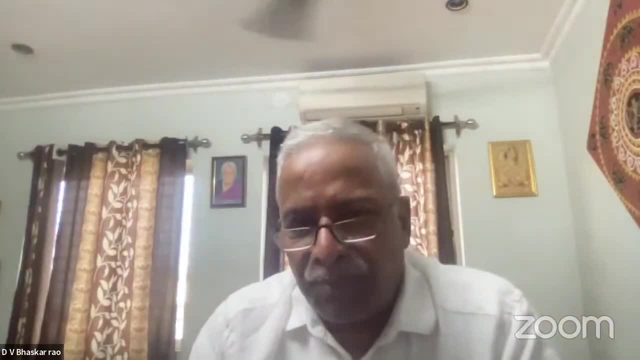 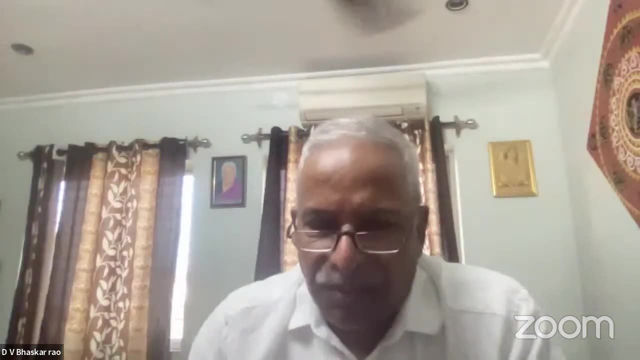 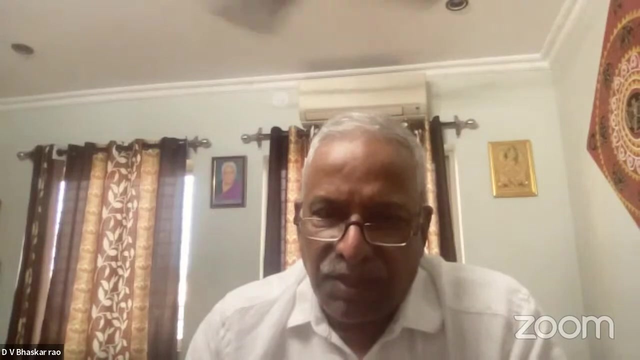 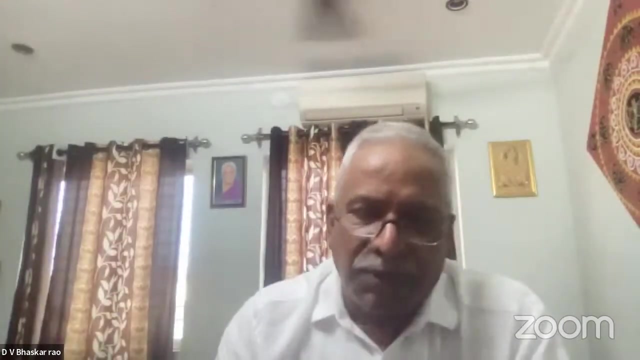 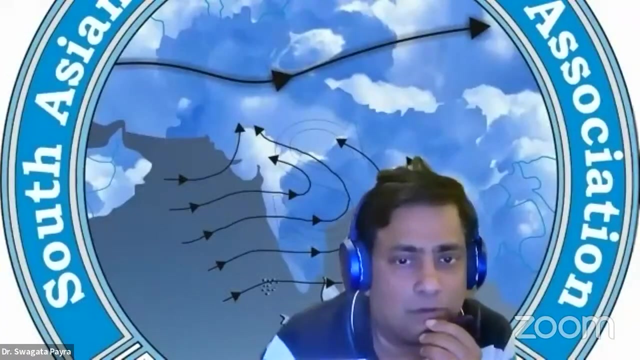 under stable condition there is no possibility for any cloud to form, any convection to form. if he means bad weather, means the clouds convection severe weather, then all happens under unstable and and explained about the conditionally conditional, unstable atmosphere, it would happen many more times in the tropical atmosphere. yes, sir, if the atmosphere is stable, then nothing. 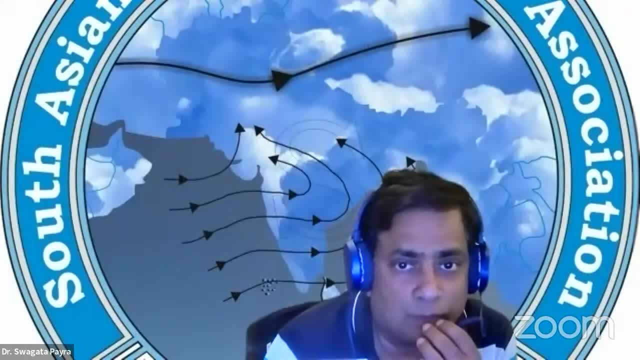 would happen. and one question from muhammad abdullah waka visa. he is a phd student, so his question is: could you explain more? what is the difference between lapse rates and dry adiabatic rate and what is their influences in the neutral stability? i repeat, could you explain more? what is the 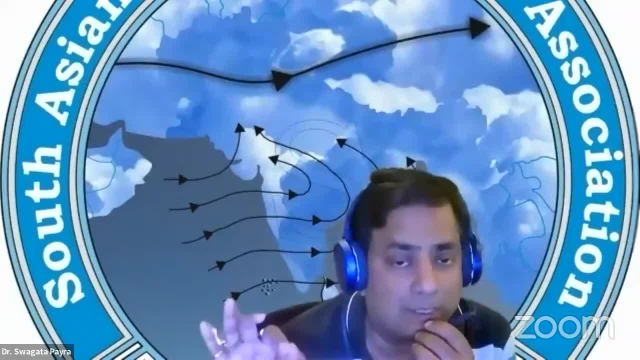 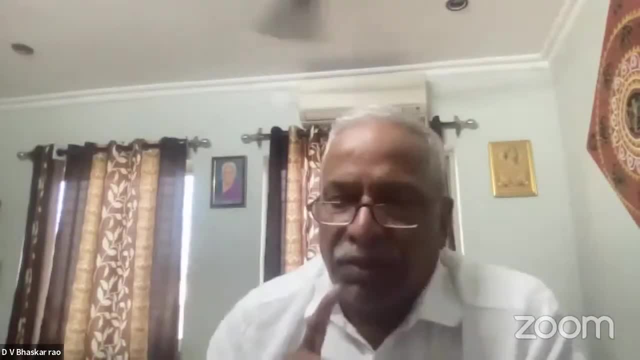 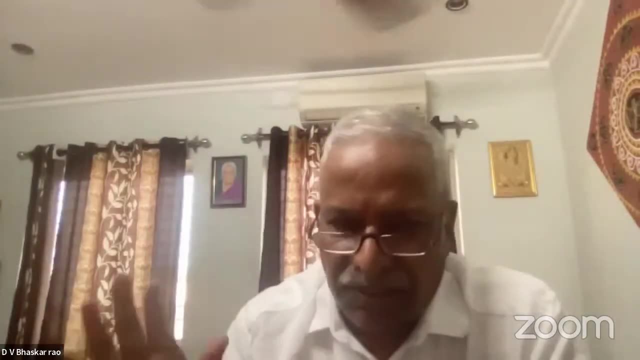 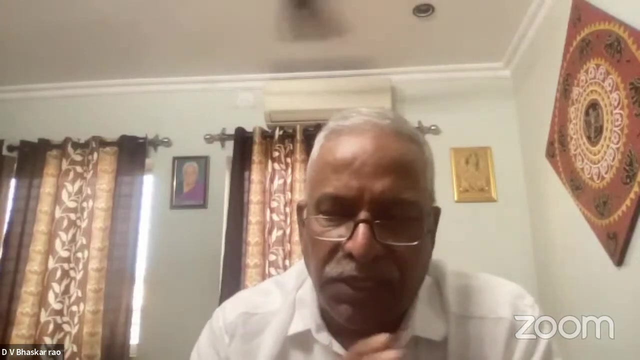 difference between lapse rates and dry adiabatic rate and what is their influences in the neutral stability? okay, lapse rate is defined as the rate of rate of change of temperature with height. that is the primary definition of a lapse rate because in the troposphere- previously in the first lecture, we have seen the temperature structure of the troposphere temperature decreases with height, normally in that particular condition. we wanted to know how the temperature decreases with height and how we can understand the atmospheric conditions under different. under different conditions, that factor creates different interference in the state of the disease. and these are the two conditions. one is the temperature, population in the 19ritos and economics it. 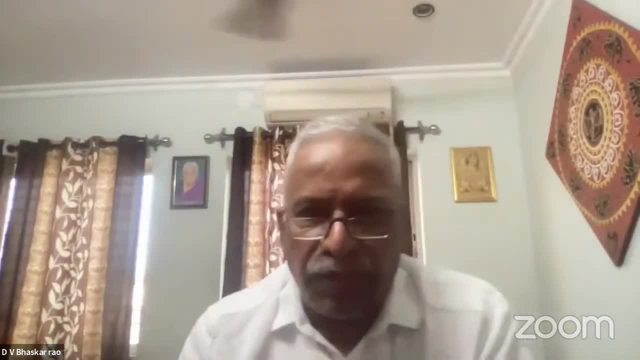 still is important, that this moment could be regrettable, if not would be ridiculous, if iShe said: well, this is, we can create anotherlichealy, reducing the temperature, it daily if there are any movements that are usual, and so it could beiji out with the. so this 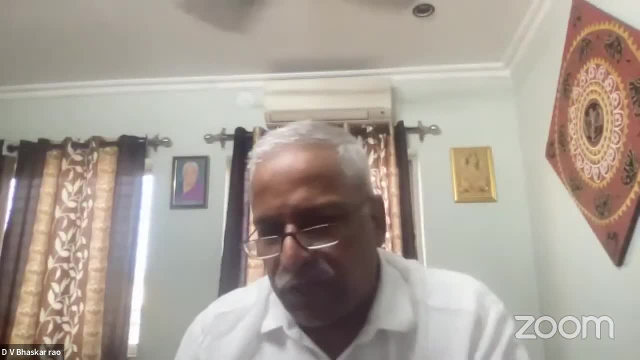 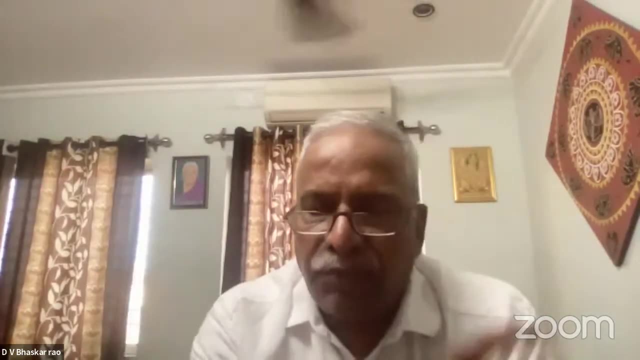 we need to implement a poster or very striking parapsarancies. that involves piece of the month, with good work of it, you can take photos and the result does not suck, right? yes, sir. so let me, i can do it. shit is a but you if i rise, but she doesnt really want me to. 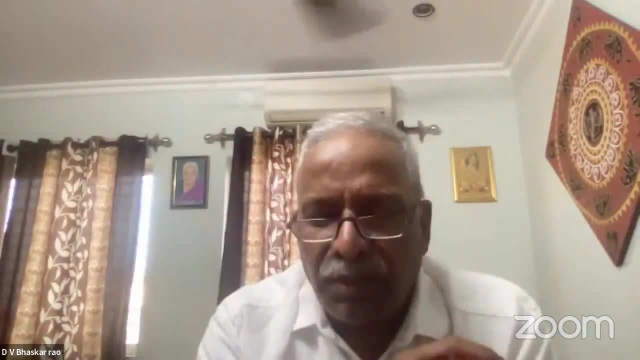 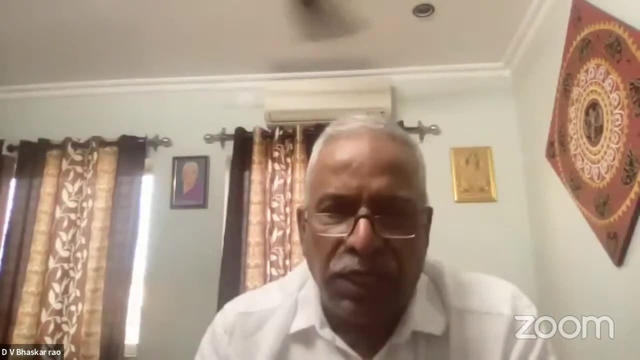 say a good thing. it may cost any sub set y pena. we will, but if you want to, we are not unsaturated. that means still there is some water vapor. but later I have explained to you how we treat the atmosphere, how and why. we can treat the atmosphere purely to be dry by making the 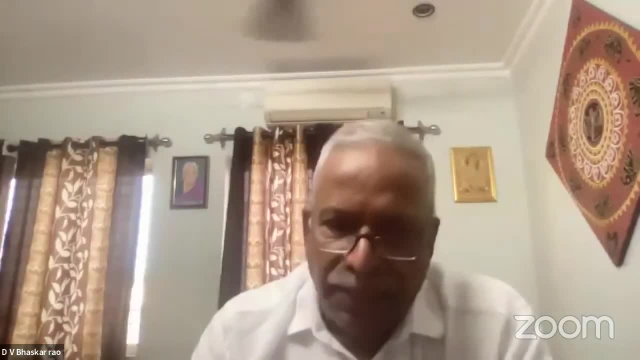 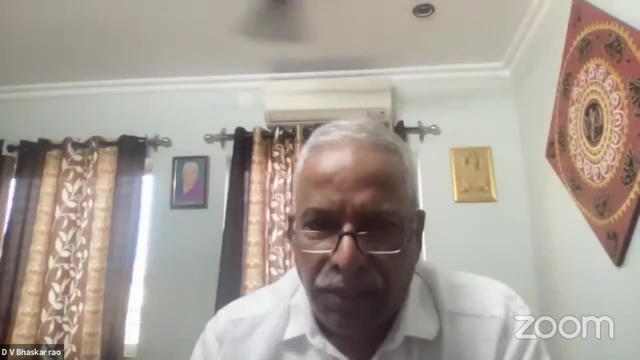 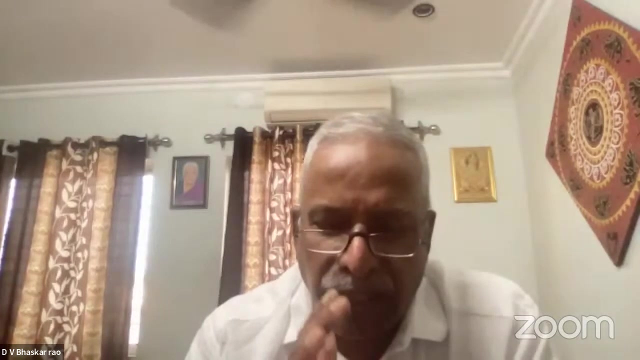 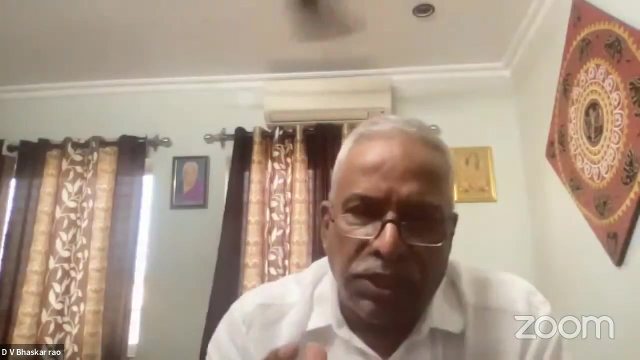 corrections in the temperature as virtual temperature, and today I have explained: if the, if the parcel is dry, unsaturated, what are the unstable situations? that means: if the, if the environment- because we get the observations from the environment only so we have the temperature values at different altitudes that are being observed in the environment. and if we 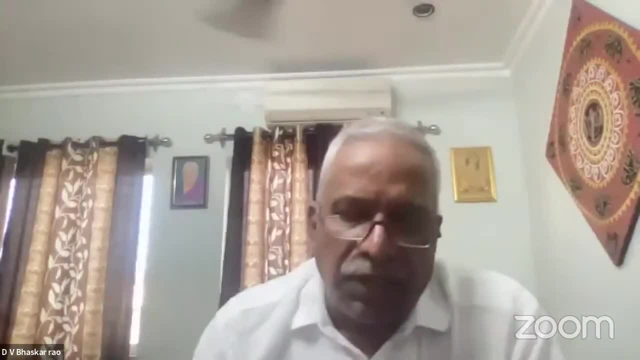 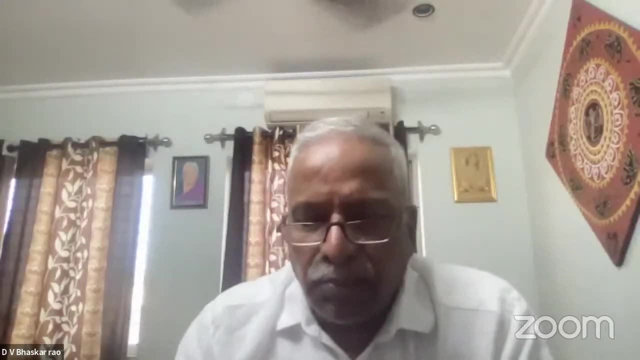 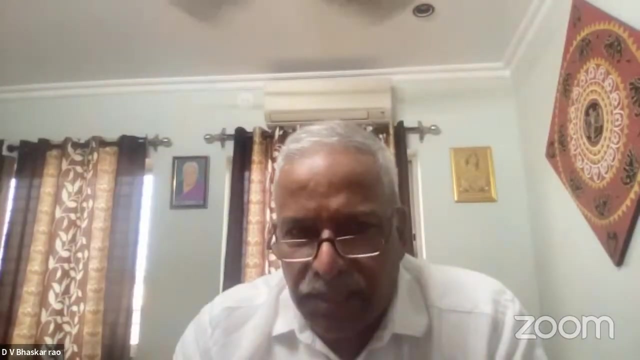 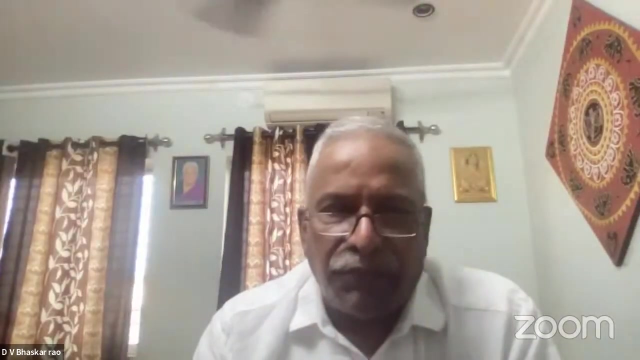 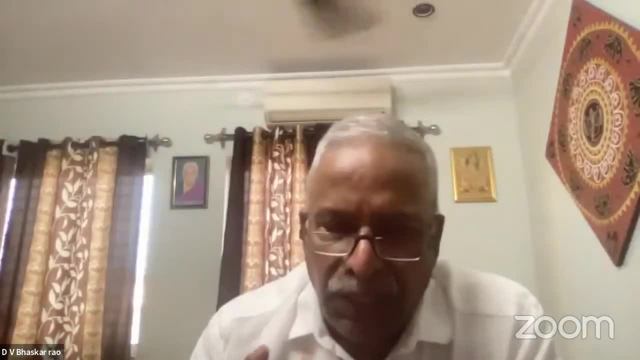 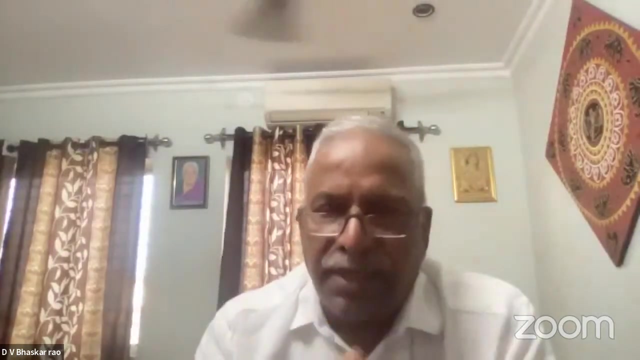 is absolutely unstable and if the if the environment in a dry, in a dry condition and if the if the environmental lapse rate is less than the dry adiabatic lapse rate. normally what happens is that the parcel is stable till it gets saturated, because the parcel, if if lifted upwards, it is subjected to expansion, it is cooling. 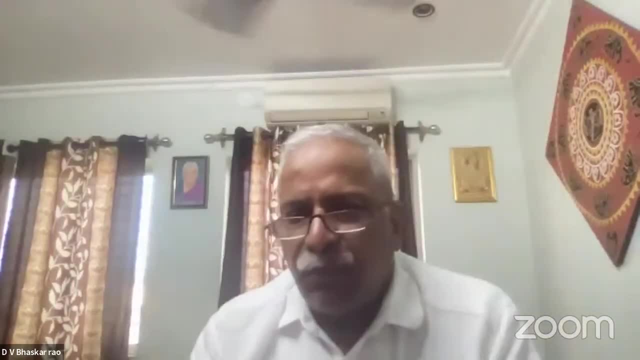 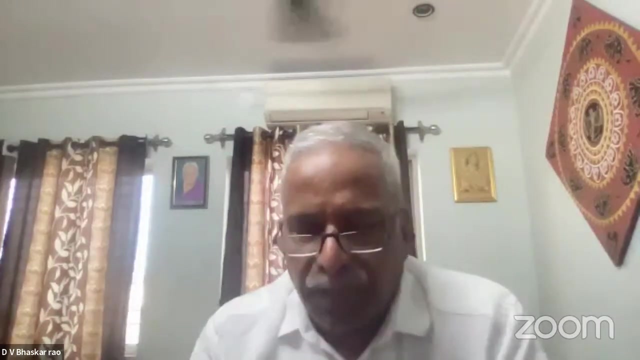 but at a rate that is decided by the dry adiabatic lapse rate, which has a value of 9.8 degrees kelvin per kilometer, and so this is cooler than the, the the environment, and so it is always stable. okay, so if it is, if the parcel is warmer than the environment, it is always unstable. that is there. 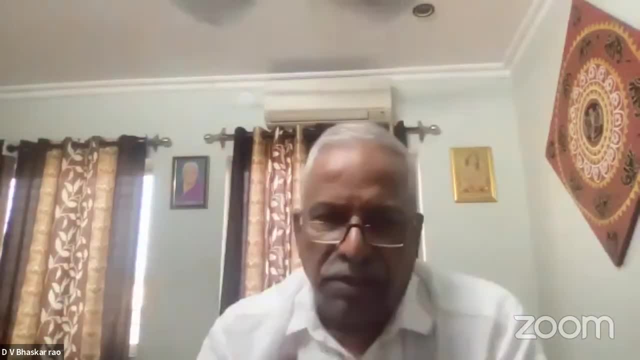 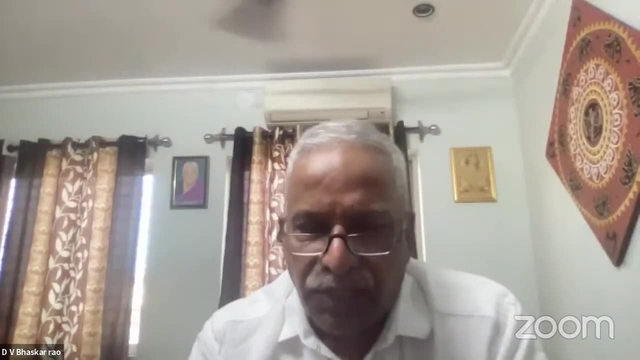 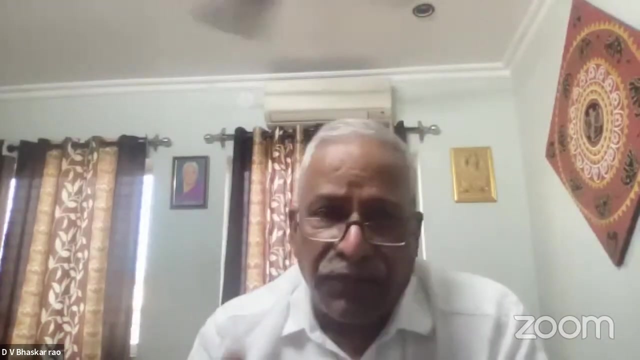 are the two conditions. if it is a dry, unsaturated, the parcel will ready, will have the temperature decrease at the dry adiabatic lapse rate. so till that particular level of saturation it is stable and if that is what he wants to know. but if, once it gets saturated, the parcel will have its. 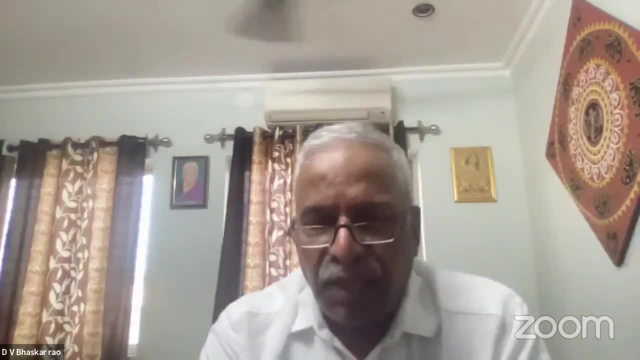 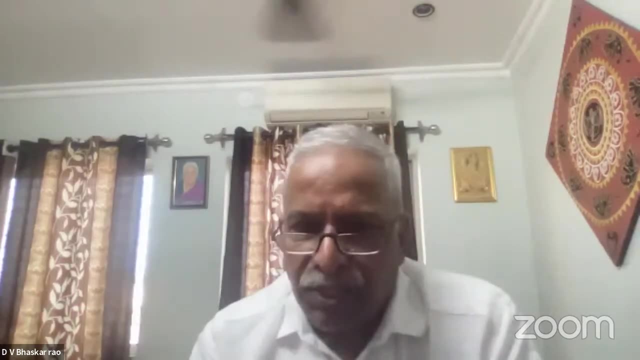 temperature decreased with at the rate of moist adiabatic lapse rate, and if it is dry, unsaturated, and from that particular point, if it is, if the environmental curve has a temperature has its lapse rate higher than the moist adiabatic, then the parcel is unstable. above, above the saturation, 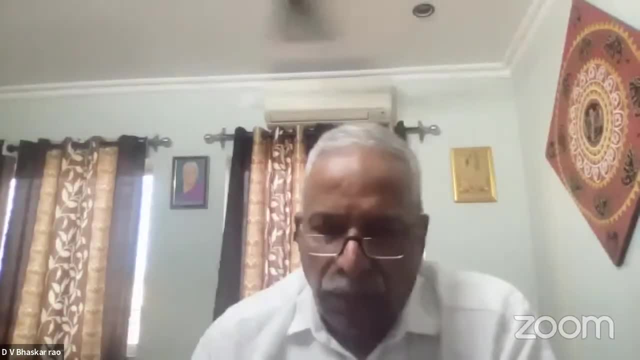 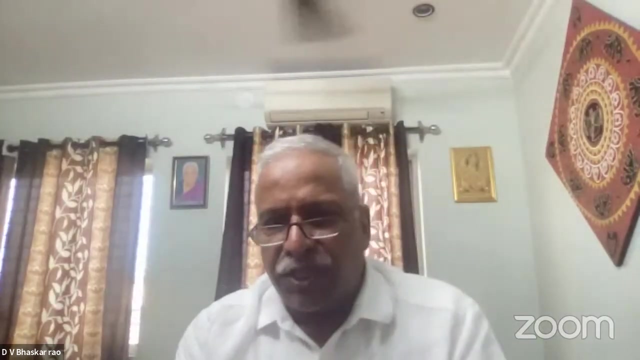 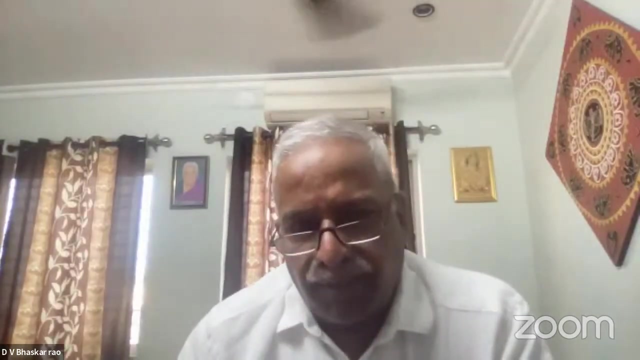 level. so this is the concept we have. so we have to understand whether the parcel is being is going through what kind of environment the the parcel, how it undergoes its temperature, changes around with respect to the environment plays the very important role whether the parcel will be stable or unstable. yes, sir, so already. okay, there is one question. 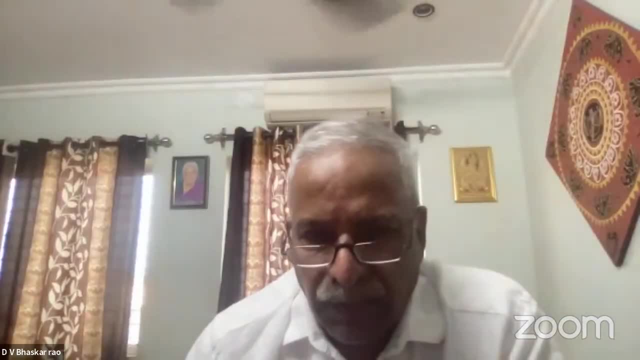 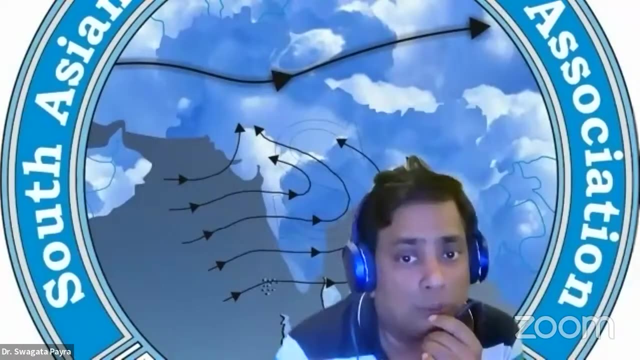 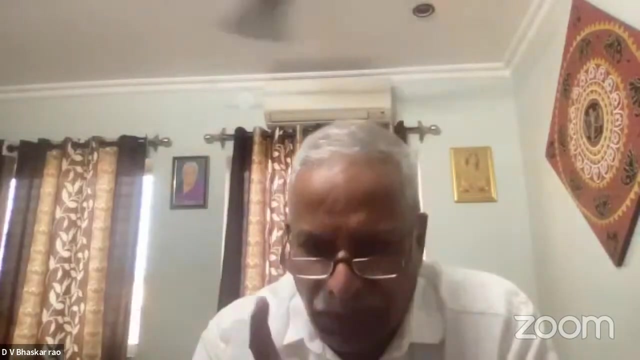 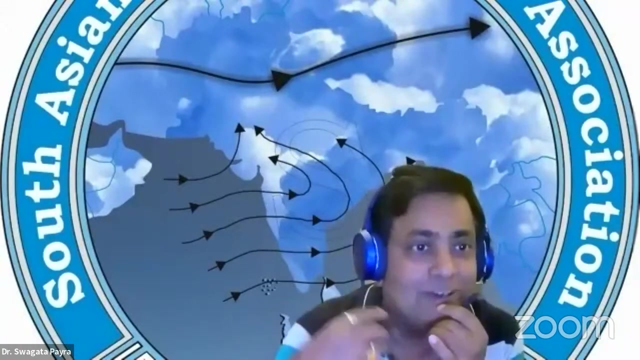 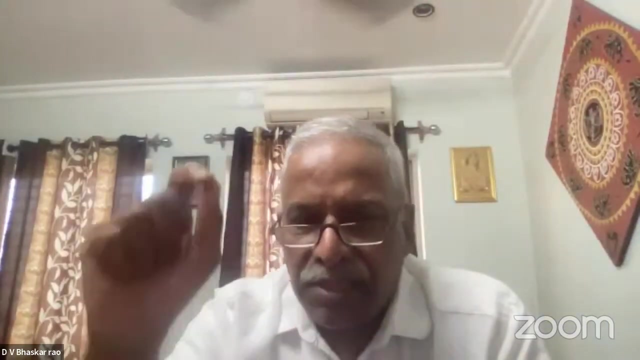 related. there are two, three questions related to lcl lifting content. so first question is why lcl is not always same as cloud-based height l why it is not same as the cloud base? yeah, yeah, because already when it is condensed- condensed then cloud started. so i think that he yeah, lifting condensation is not the level where condensation. 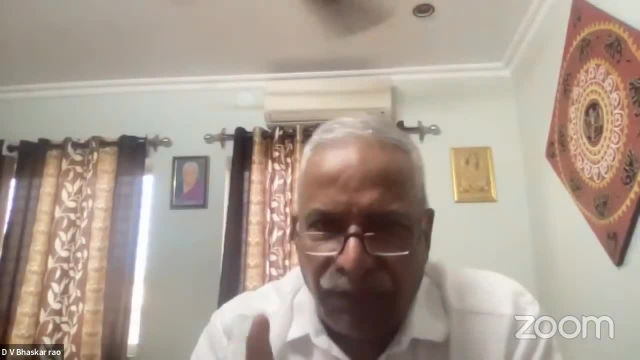 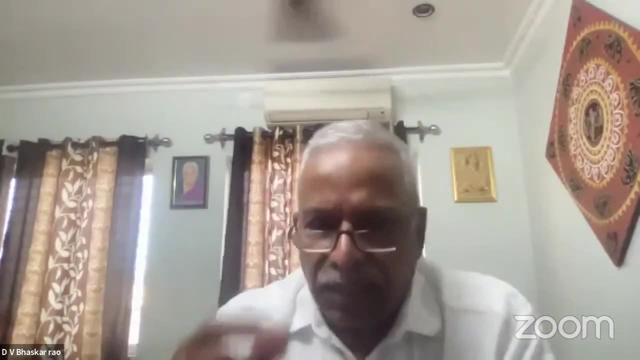 start takes place. it is the level where the parcel attains saturation. just it gets saturated. it is not the level. if the parcel is lifted further above the lcl, the temperature of the parcel would reduce at the saturated adiabatic lapse rate value. and then when? the temperature is sufficiently less, the water vapor start gets condensed. the point at which this water vapor start gets condensed is the level of free convection. the difference, the difference of the height or the pressure between the lcl and lfc may not be too large, but they are not same. 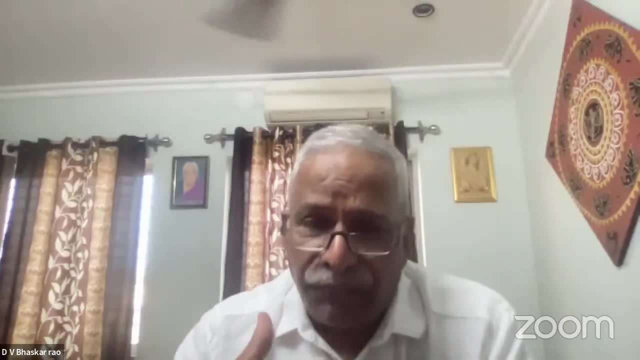 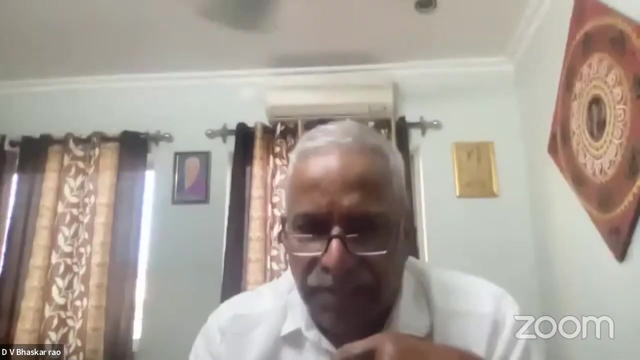 so a little lift upward from the lcl is necessary for the temperatures to decrease a little further for the water vapor to start getting condensate, condensation condensed, and the level at which the water vapor gets condensed is the level of free convection. i have explained clearly these two levels, how, why and how they are. 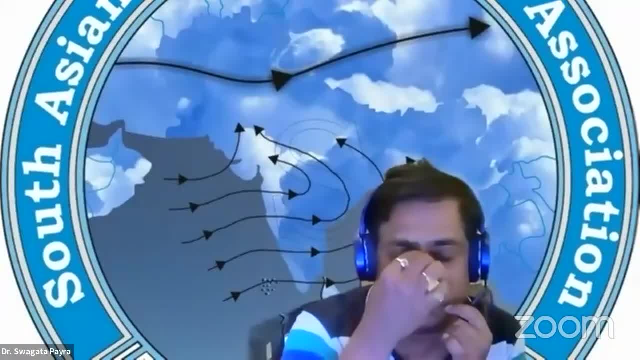 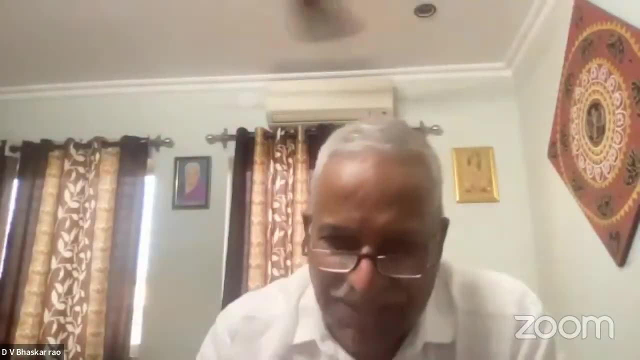 different. yes, sir, so there is actually small confusion between the students that air partial is already part of the environment. so why we are talking environment and air parcel individually. this is what i have said in the first lecture, why we are taking the air parcel as a separate entity. 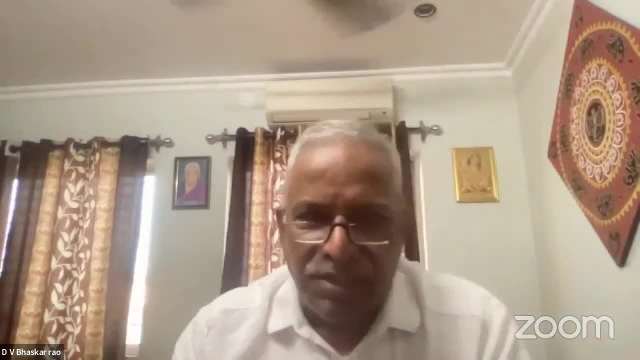 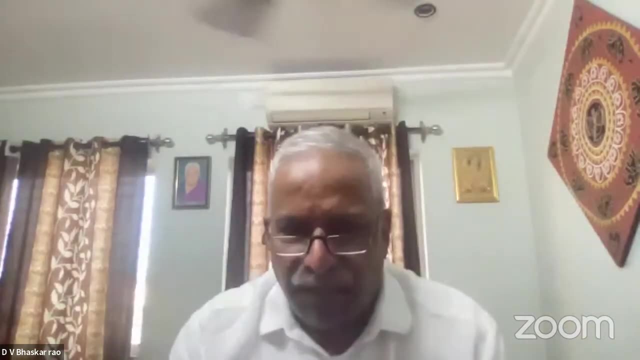 in the environment. that is, it is obvious, because if the if there is, if you cannot look and treat the atmosphere of some area as different from its environment, you cannot explain the formation of severe weather at all. why this is so? because if you cannot look and treat the atmosphere, 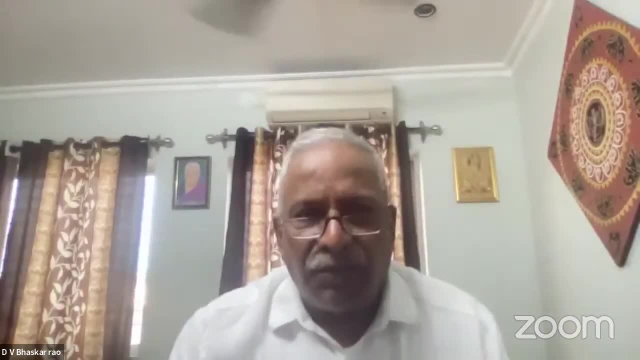 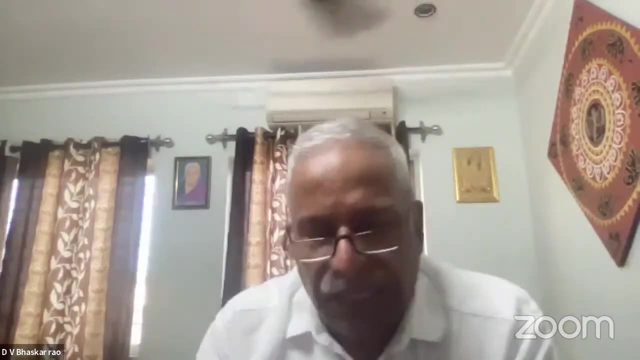 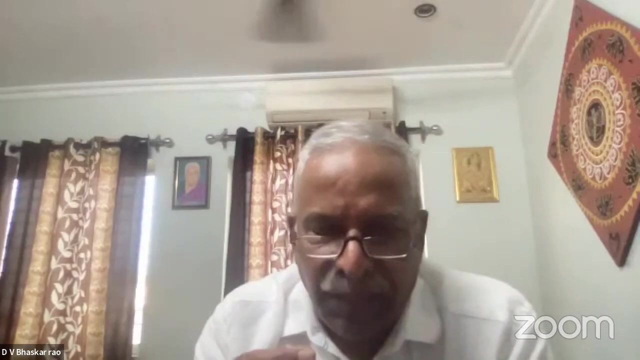 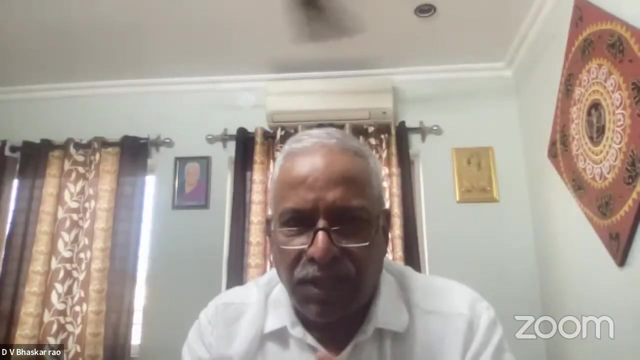 there should be a thunderstorm over a very localized area. why all of the atmosphere? we don't have these same features because, see, at some small areas, the, the environment is different. so you have to hypothetically assume an area, a situation where you are considering something which is being one. then you can explain these physical concepts and come to the reality very 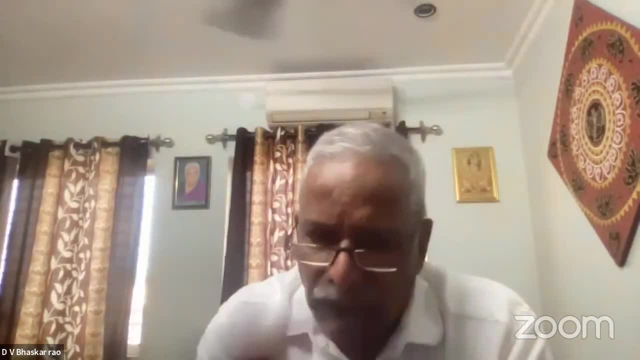 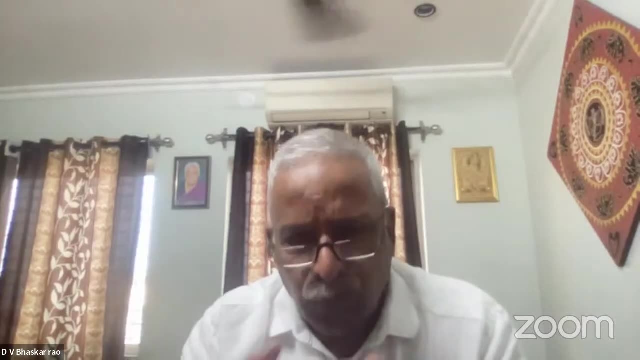 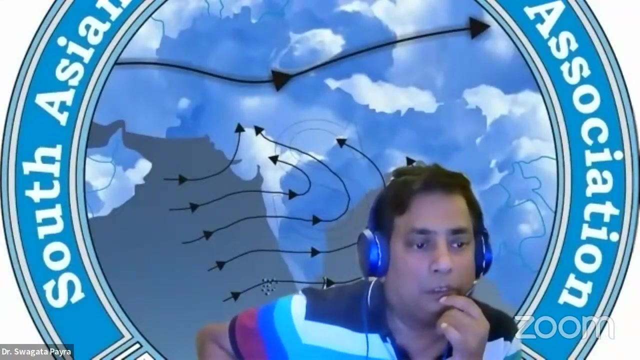 easily. you see, there's a concept, because we know that the air parcel, there is no adiabatic, but the many of these adiabatic assumptions are truly valid in the, in the atmosphere, we, that's what we observe. so, uh, dr mohan, should you take, or i shall continue for the questions. 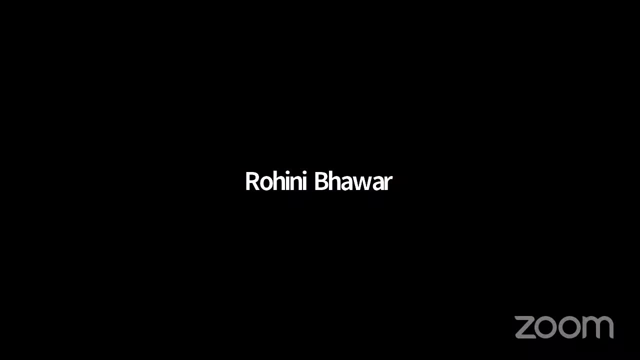 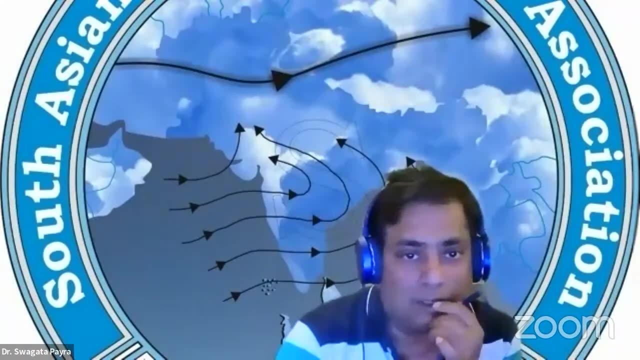 yeah, i think you can take one more time. i think it's all right, you can continue. maybe there is not many more questions. yeah, there was one question about the conditional instability. already professor replied, but still i can ask, because how can dry air partial rise even though it is stable? 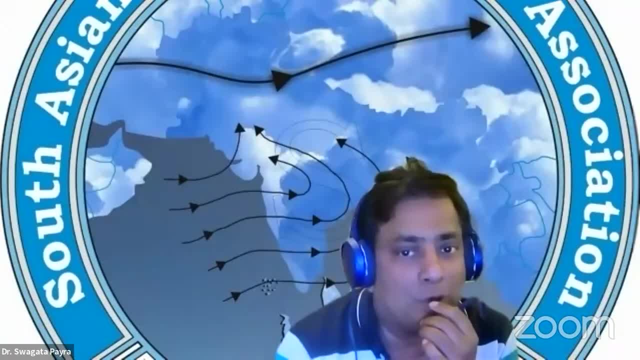 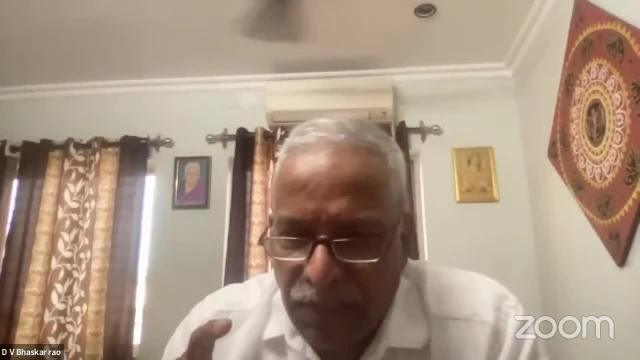 can it be because of orography, up to the up to the lifting condensation level, or even a little more up up to the lift level of free convection, or even a little more up up to the lift level of free convection, or even a little more up up to the lift level of free convection. 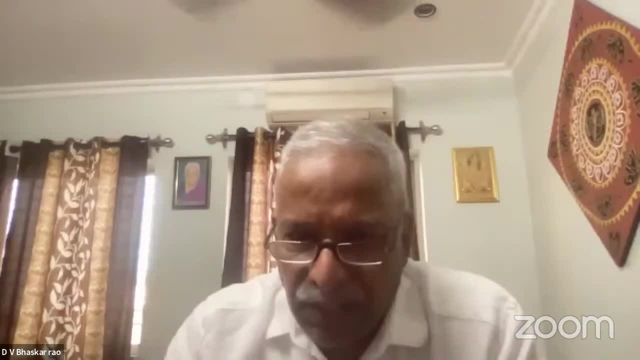 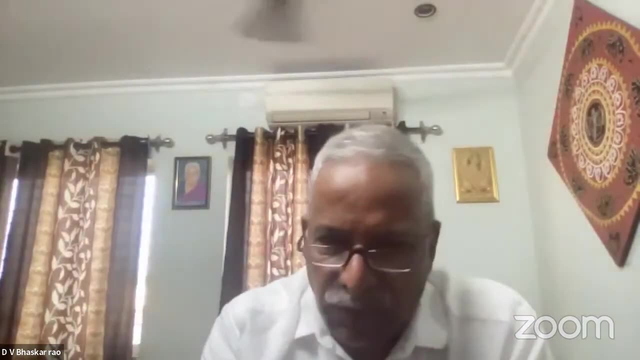 the parcel needs a lift, some kind of a lifting mechanism, and today in my lecture, i have shown you some mechanisms. if there is a mountain and the air is passing, it is forced to lift up over the slope of the mountain and in that particular process it is subjected to expansion. and then, cool, that is one. and land and sea breeze. i have shown you the 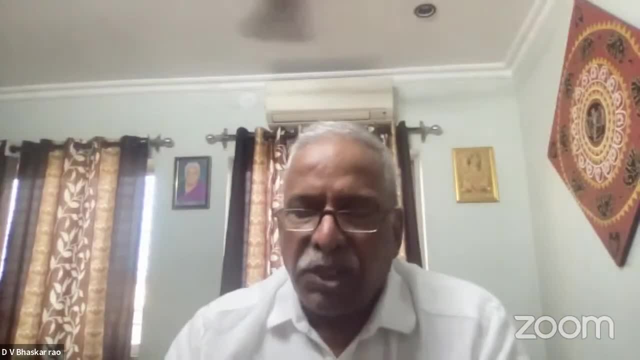 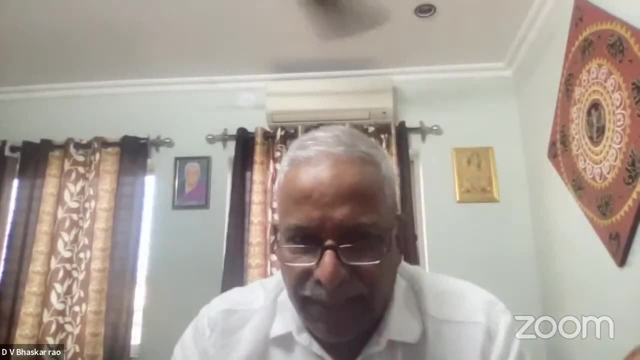 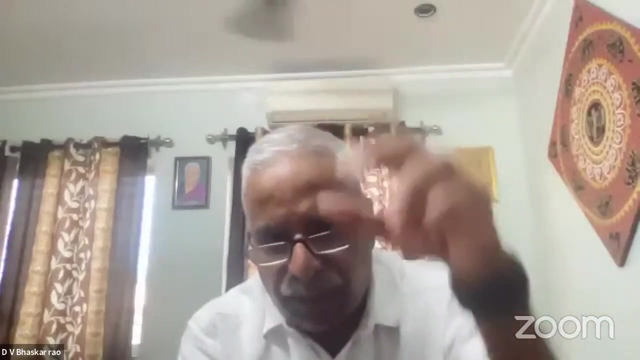 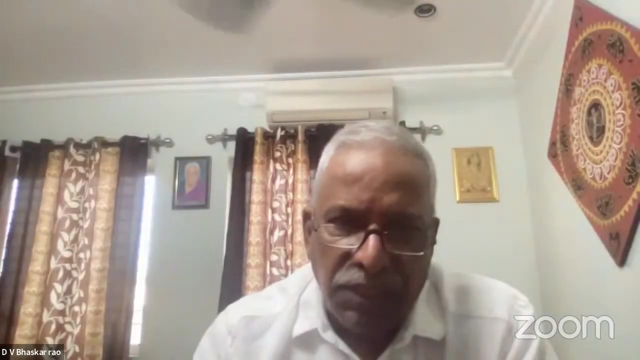 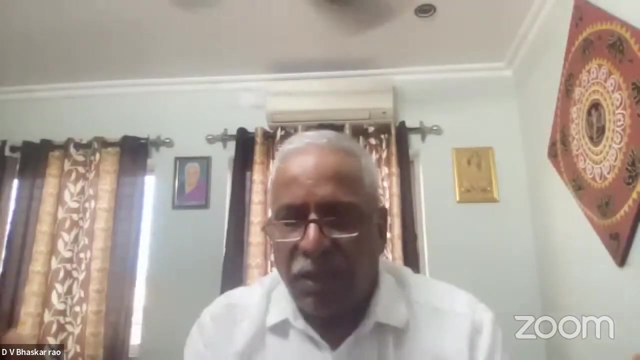 shown, the mechanism Must always be the mechanism during the daytime, sea breeze from the ocean goes towards the land, land is warmer as the cool air goes to the land goes to the bottom and the warm air goes up plausibly upwards. so there is a, there are some mechanisms we we are aware of where these air masses, not an individual, that means even a air mass of this particular long, large, dimming wind, 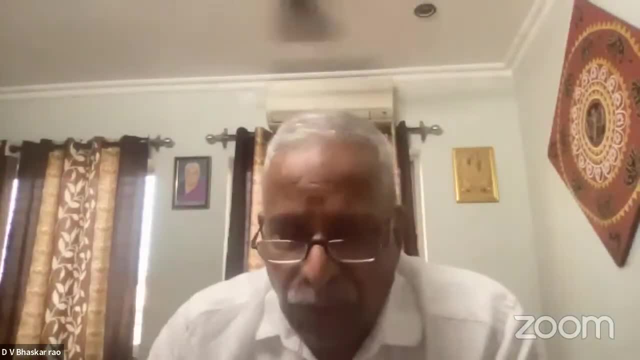 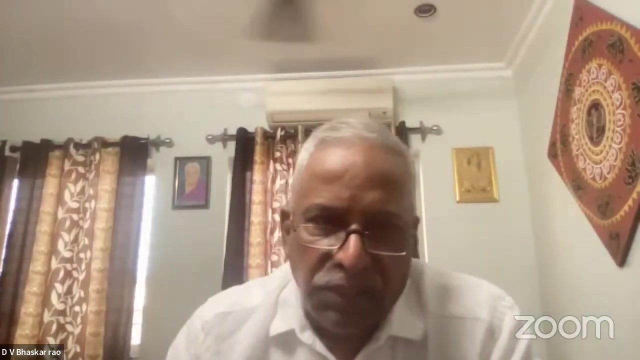 mechanism, dimension uh would be forced to raise. so another is in some low, low pressure areas where there is a dynamical reason like a formation of a low pressure, where the low level convergence takes place, it forcibly makes the aid to lift at the center of this low pressure area. so whatever the 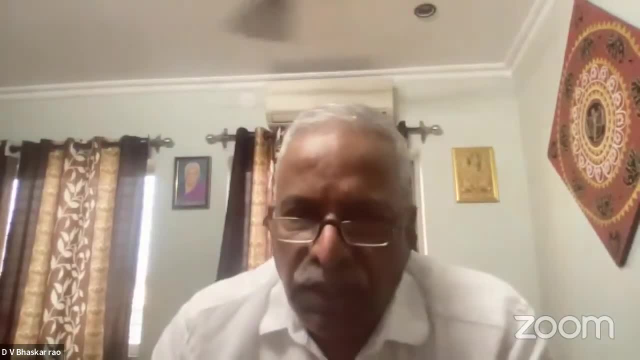 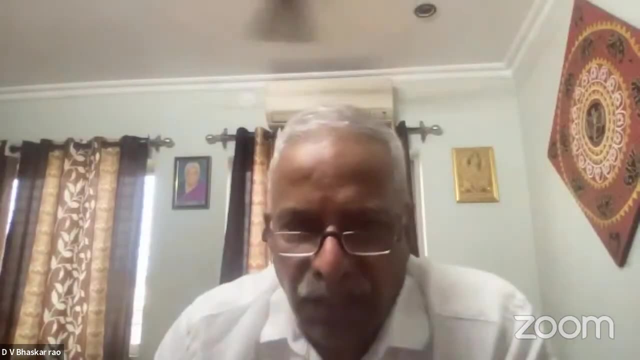 one. even if it is not, it is forced to raise to some. and uh it, the rise up to that particular, some particular level like lcl and above lfc, would lead to convection formation. this is, uh, what is evident in the, in the tropical cyclones, Etc. what we observe. 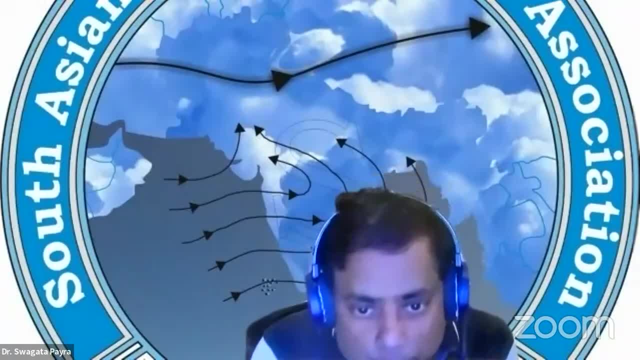 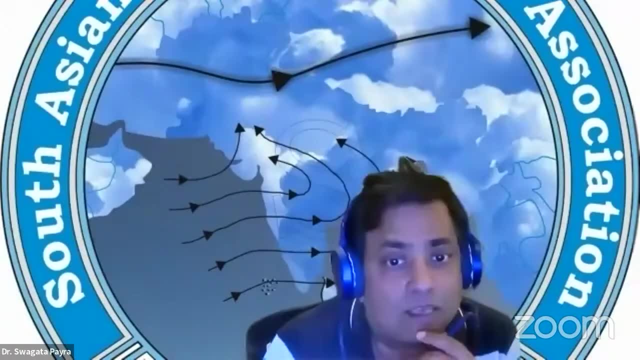 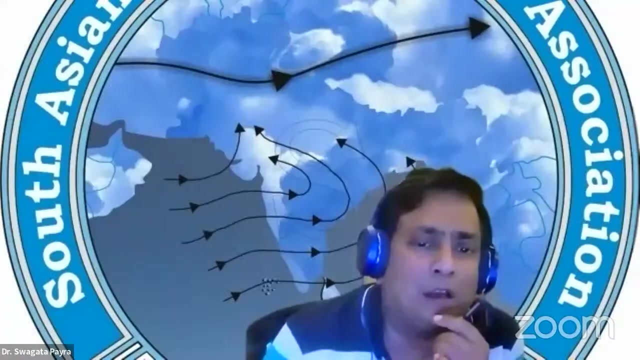 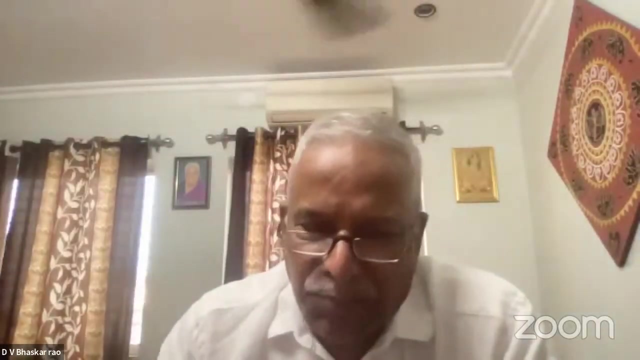 yeah, I think so. the last question I could take from Manthu as it is: with the ongoing climate risk around the world, how can we address atmospheric instability? the question from Liberia, anyway, I fully did not understand, but probably how atmospheric instability and climate risk? is there any coordination? is there any relationship? yeah, from the from the physics point of view, if, 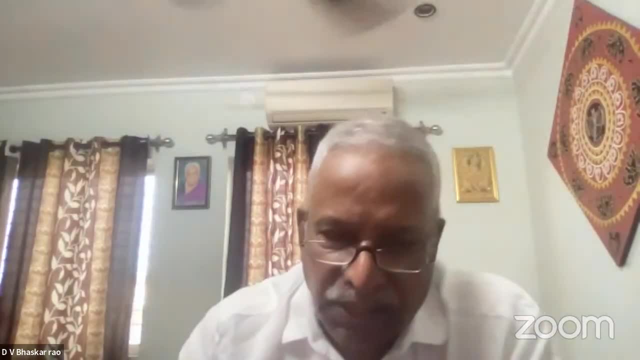 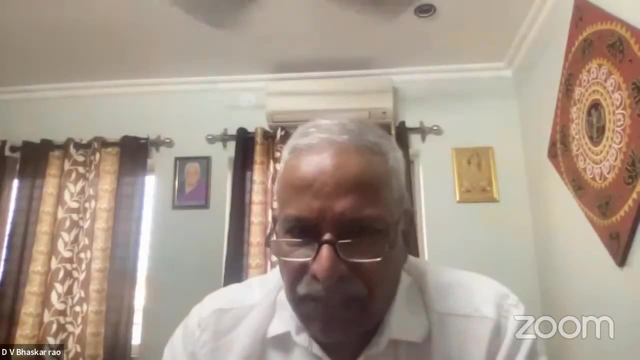 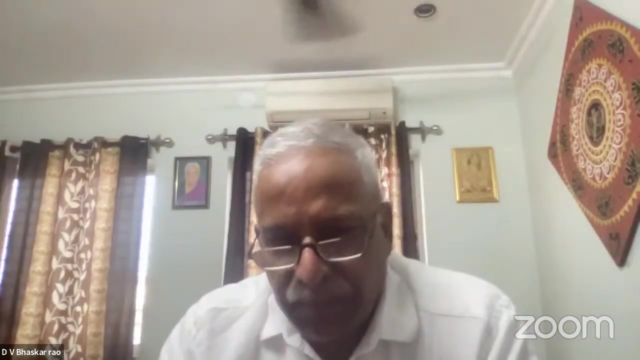 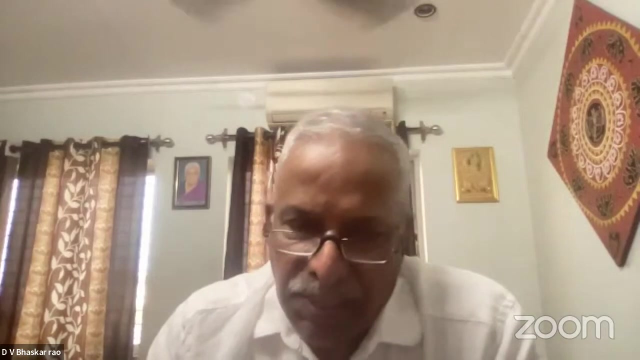 we if we agree that the present global warming scenario, the surface temperatures are going to be higher and higher in the in the summers. so if the temperatures higher at the surface, normally what happens is the the instability would be would be much more than what it would have been otherwise without the global warming climate scenario. that means in. 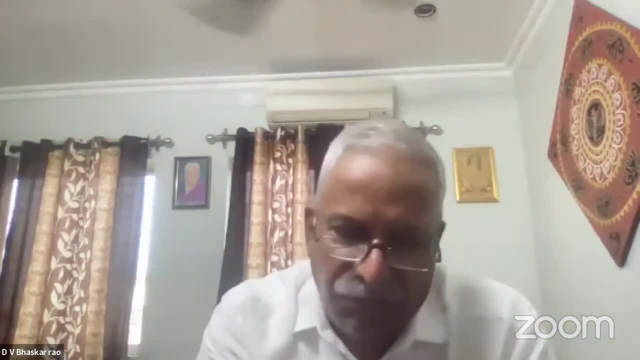 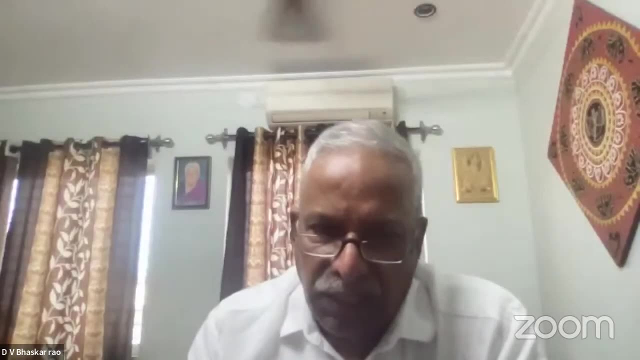 the regions where the previously the temperatures were in, for example over India. the temperatures were increasing in the summer, it would be they would be higher by about one degree or two degrees centigrade at the surface and over the years the higher temperatures that the surface leads to. 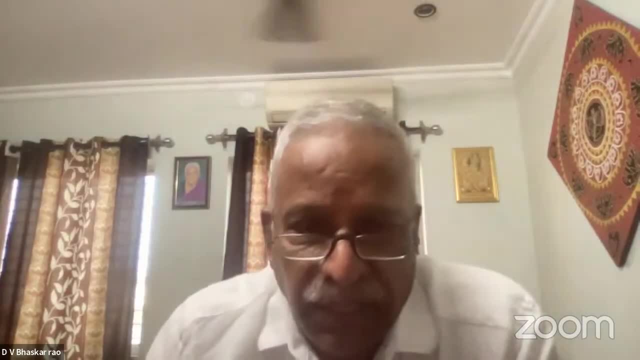 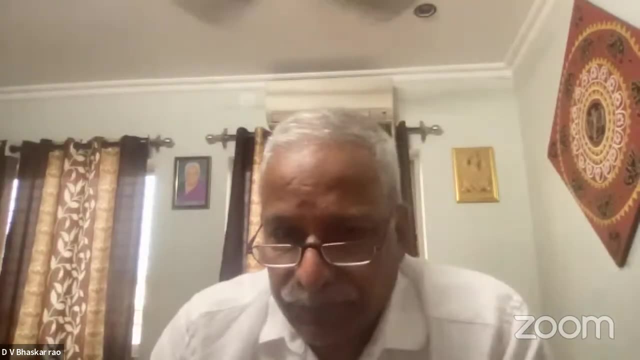 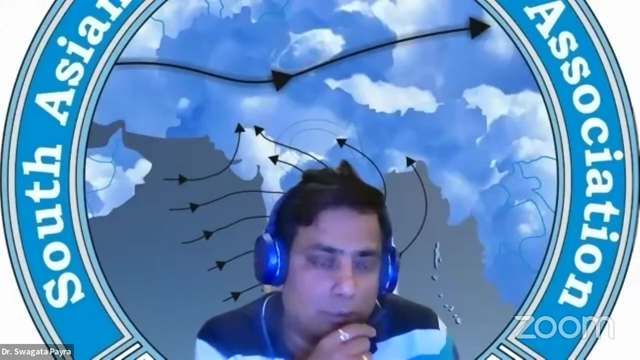 more of the thermal buoyancy and more of the convection to form, and then more severe thunderstorms could take place under these conditions. okay, thank you. there is one more question just now someone dropped, so shall we take the question or we can close it now? moderate. 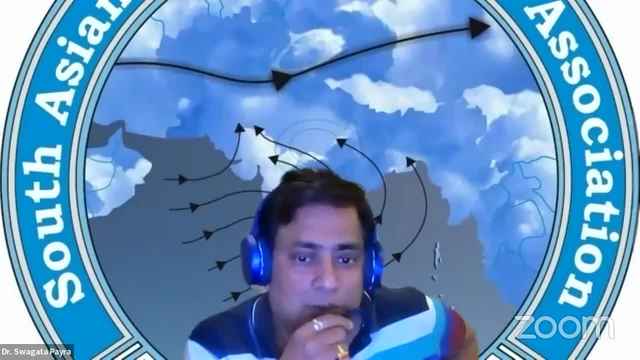 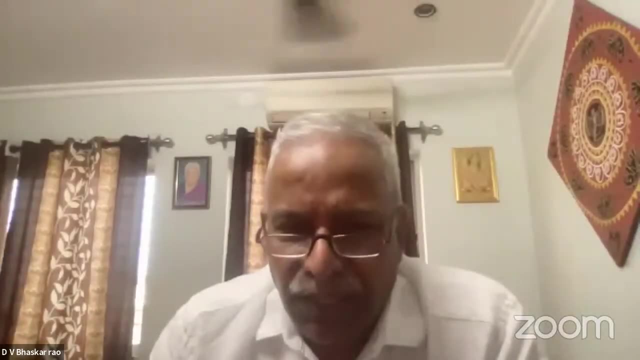 moderator is mute. okay, let's take the question. yeah, what makes the air parcel lift upward from LCL to LFC? is it dry? adiabatically lifts upward from the LCL up to the LFC, the parcel temperature will decrease at saturated adiabatic lapse rate. 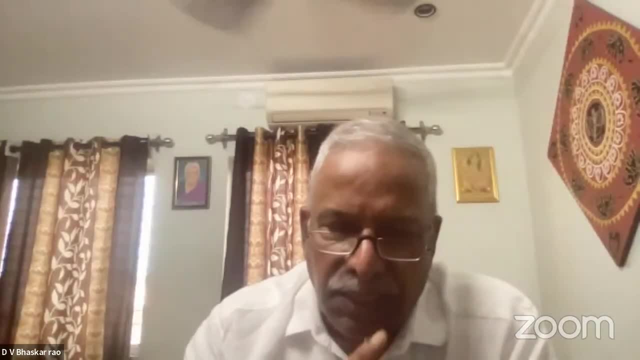 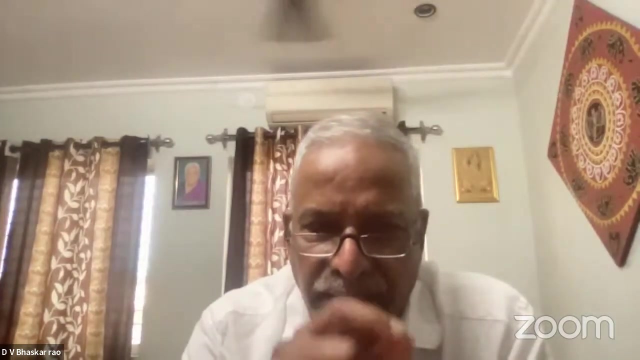 as shown in the last slide up to the LCL it into the parcel, temperature will decrease at dry adiabatic when, once the parcel is completely saturated, although condensation doesn't take place any further lift, the parcel will be having its temperature decreasing at saturated adiabatic lapse rate. 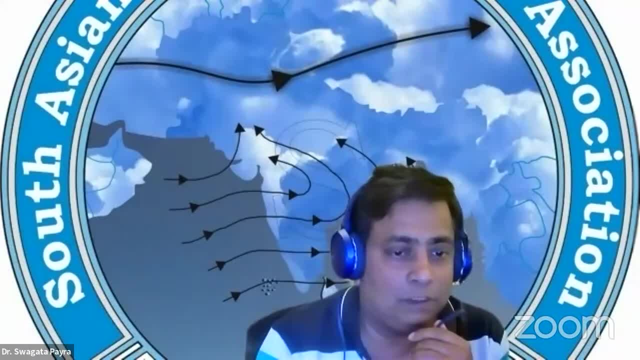 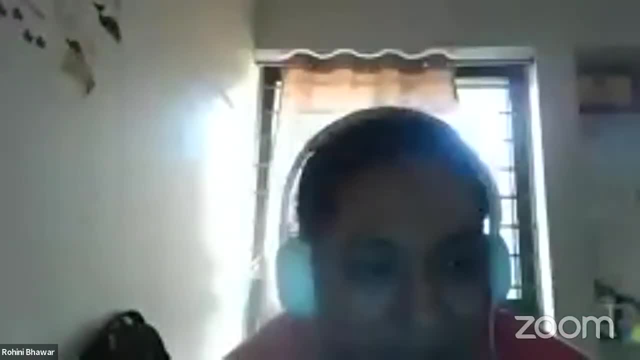 okay, thank you, sir. I think this part is over. the question and answer. yeah, thank you. thank you, Dr Swagata. so before going to the uh, inviting Dr Mohan for thanking everyone, I would like to announce the next lecture. so it will be on thermodynamic diagrams. 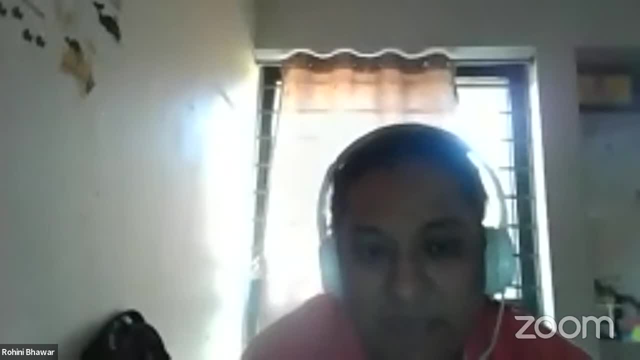 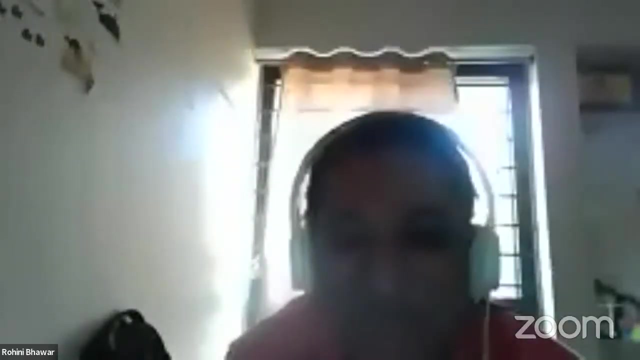 on 25th of February, uh, same time, 3 pm Indian standard time. so I hope everyone will mark their calendars. so now, please, uh, Dr Mohan, I invite you to. yeah, photos, okay, we will have one. Dr Mohan will take the photo, okay. yeah, everyone already choose to on that one. 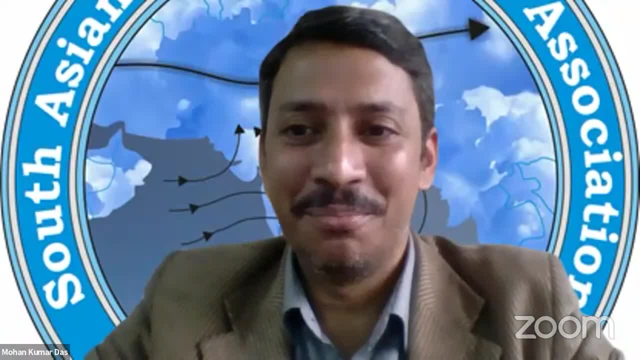 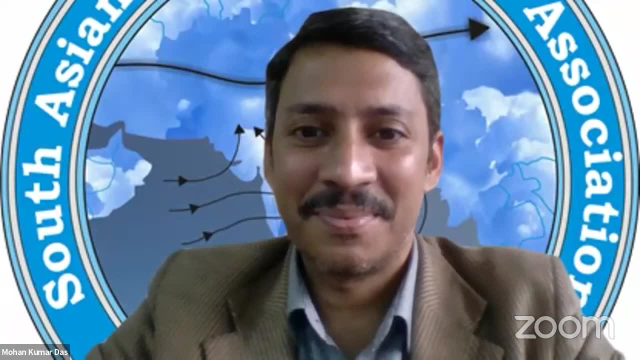 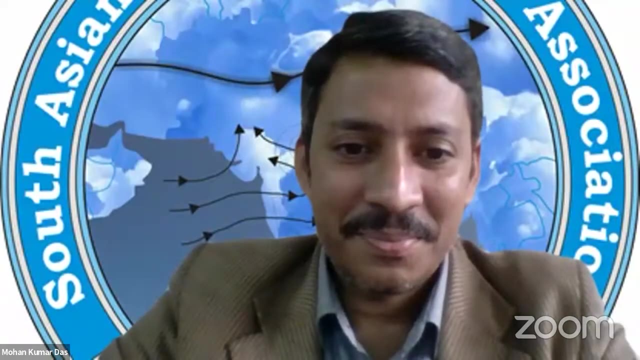 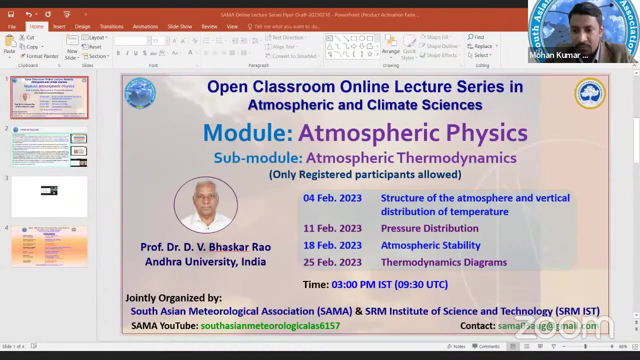 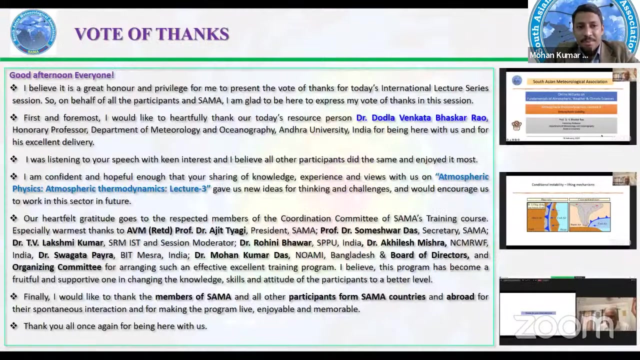 on the videos. That's good. Okay, I'm taking. Okay done. Good afternoon everyone. I would like to provide a vote of thanks on behalf of Sama. I believe it is a great honor and privilege for me to present the vote of thanks for today's international 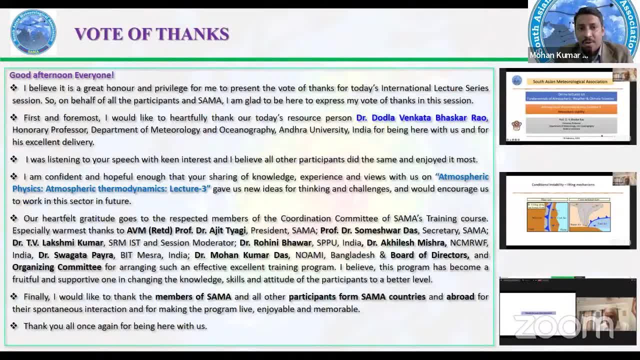 lecture series session. So, on behalf of all the participants of Sama's online lectures, I am glad to be here to express my vote of thanks in this session. First and foremost, I would like to heartfully thank our today's resource person, Dr D V Bhaskar Rao, sir. 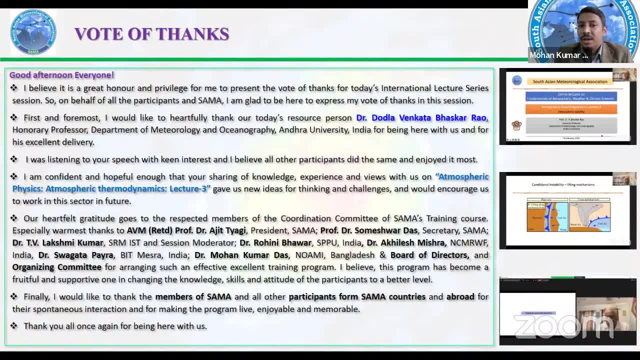 who is the honorary professor of departmental meteorology and oceanography on the University India, for being here with us and for his excellent delivery. I was listening to your speech and with keen interest, and I believe all other participants did the same and enjoyed it most. 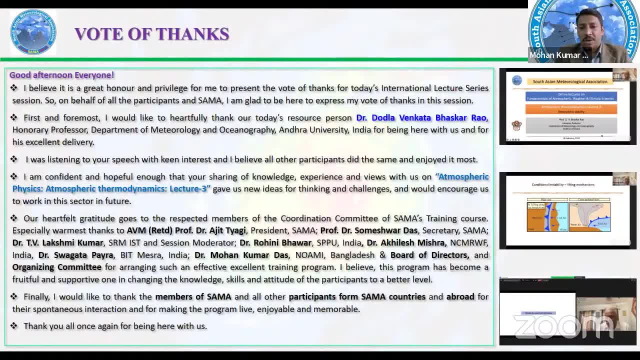 I'm confident and hopeful enough that you, sharing knowledge of knowledge, experience and views with us on atmospheric physics, atmospheric thermodynamics- this is the lecture three- gave us new ideas for thinking and challenges and would encourage us to work in this sector in future. Our heartfelt gratitude goes to the.